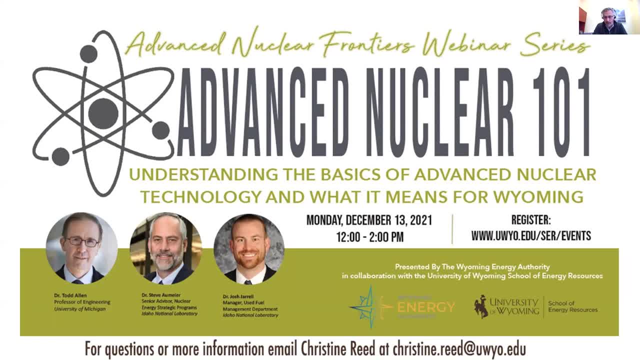 and important role aspect of a future energy economy in Wyoming. So, like I said earlier, I'm Glenn Morrell, I'm the Executive Director here, And the Energy Authority was established the first July of 2022 in the simplest form, to create an agency that could act in a coordinating 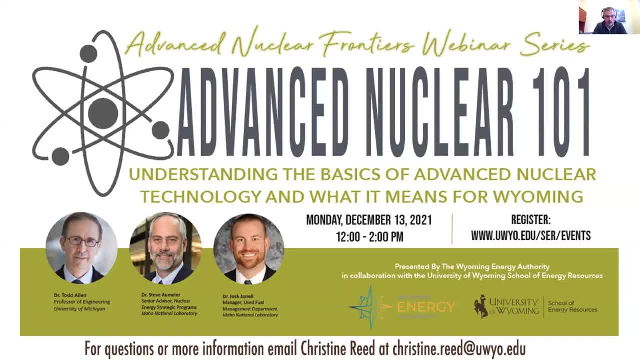 role for all the energy activities that are going to be happening in Wyoming And I'm going to talk about that in a little bit. So the Energy Authority is a very important entity that's going on within the state of Wyoming, both public and private. So the public 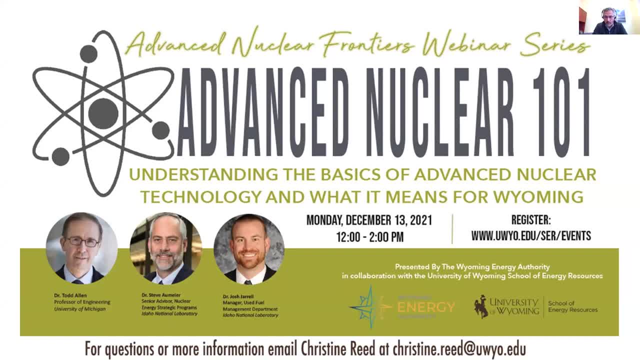 side. the energy sector here is addressed by quite a few different agencies and authorities. There is no central Department of Energy for Wyoming, as there is a Department of Agriculture. It's spread across multiple agencies and other organizations which is in some ways a little. 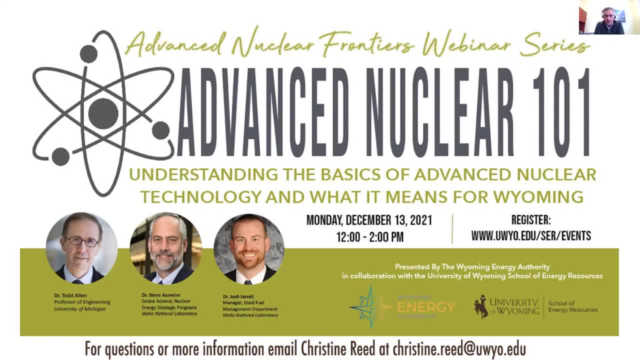 strange, given that the energy economy is such an important part of Wyoming's economy as a whole. The energy sector is the largest component of the Wyoming economy in total. It's also Wyoming has the third largest energy economy in the country on a state by state basis. 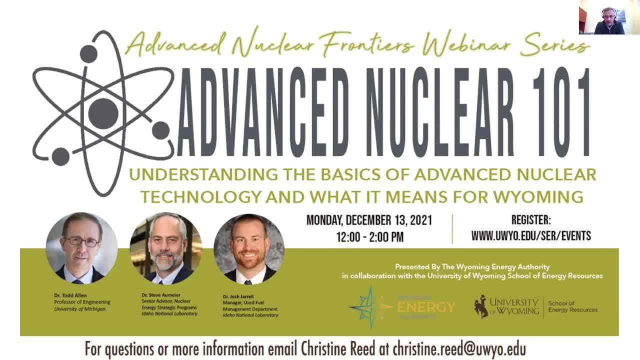 And if Wyoming were a country, it would be the 13th largest energy economy and equivalent to that of Norway. In Norway, of course, there's no slouch when it comes to energy, So the Energy Authority sits in the middle of it all, trying to make sure that there is a cohesive 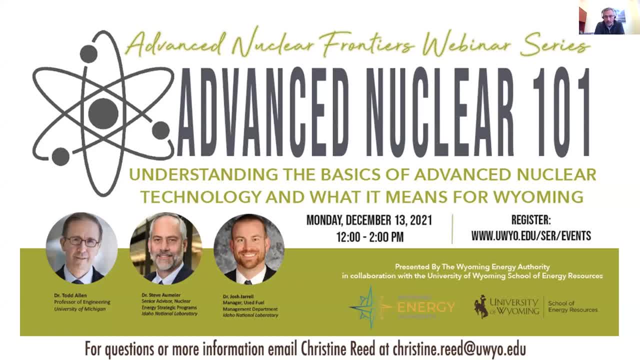 vision to what's going on, And so the state agencies and hopefully our private partners are trying to do in terms of advancing the energy economy in general, And we do that by developing and administrating the Wyoming Energy Strategy. The Energy Strategy, as most strategies have, is a central, unifying objective around continuing to power the nation. 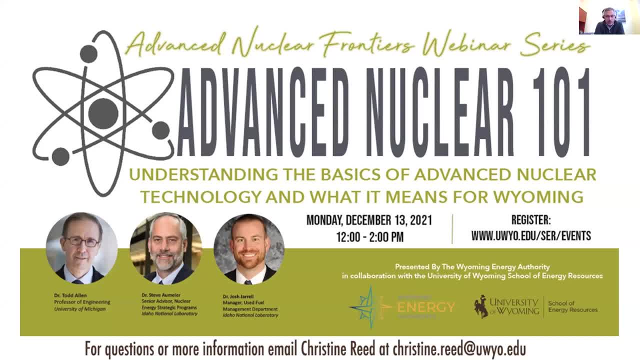 within all of the above and, most importantly, a net zero carbon emissions objective. The net zero piece is very important because we're able to see these opportunities, see these opportunities for a greater and more efficient future. We can't do those things without the fourth and 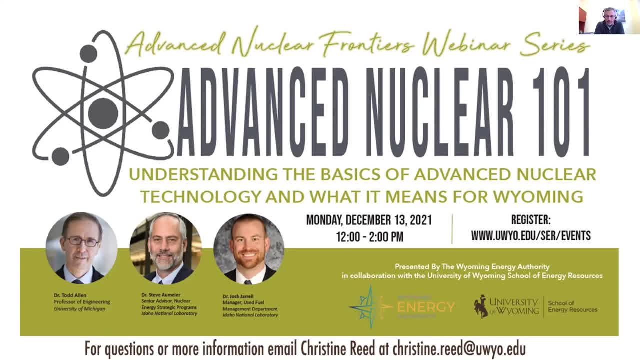 because it's simply the only way that a traditional hydrocarbon-based energy economy like that of Wyoming can continue to be relevant and sustainable and have access to our consumer markets in the future. Another interesting statistic is that we export 90% of our energy that's produced in Wyoming. 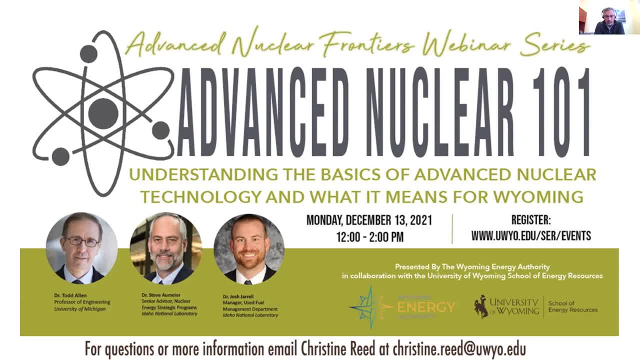 90% of it is consumed outside of our borders. And the market access. so obviously the market access is incredibly important. If we cannot preserve that, then we're gonna have issues moving forward. So net zero becomes very, very important. I could spend hours talking about the strategy. 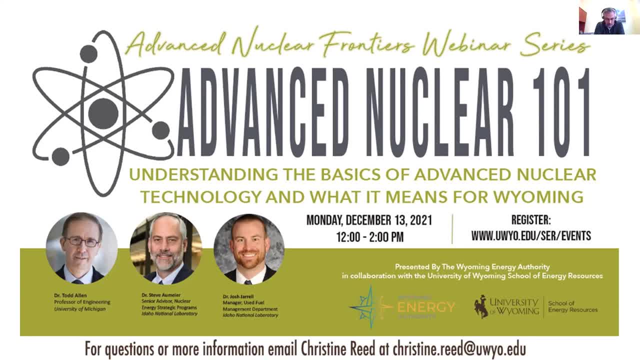 but I wanna move on a little quickly. The strategy itself has three primary initiatives, which are all really part of this vision: to transform what we have today in a way that adds a lot of value. takes a traditional economic setting and advances it through integration of technologies. 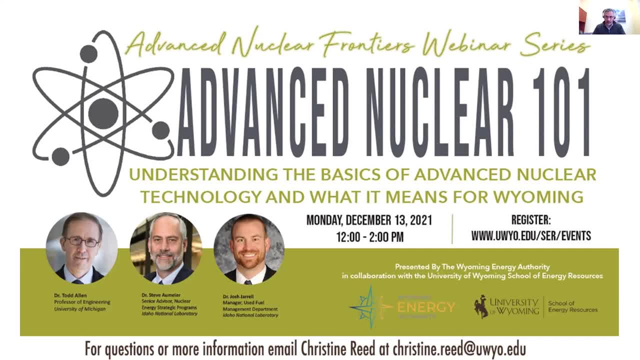 and recognition of that net zero aspiration. So we have a CCUS initiative, we have a hydrogen initiative and the third one is advanced nuclear And it has always been part of the strategy but it's really brought to the fore by the big announcement in early summer. 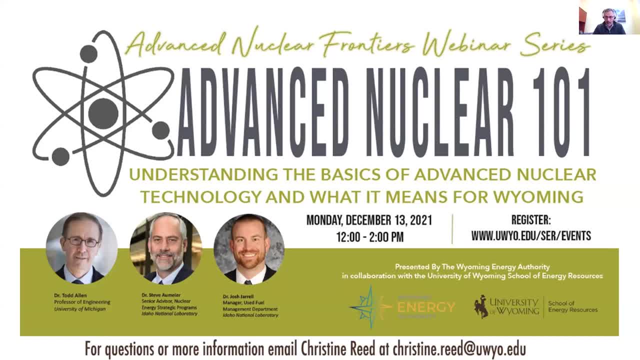 when TerraPower, in partnership with Pacificor and the DOE, announced that they would build a test reactor, a natrium reactor. Since it's been announced, it'll be in the camera area And, aside from simply being a very, very exciting announcement, as a technology guy 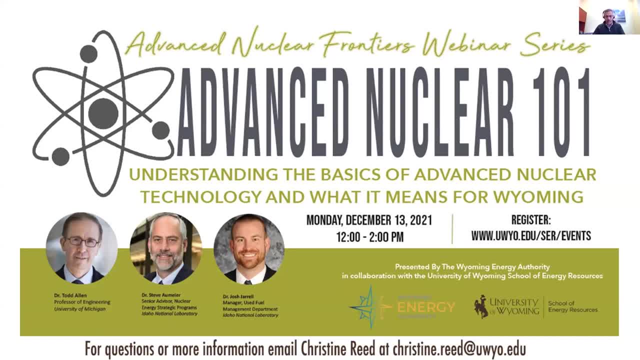 it's a very, very exciting announcement As a technology guy. it's a very, very exciting announcement. As a technology guy, I was super excited. I just thought that was the coolest thing ever. But what we've learned over the last four or five months or so, 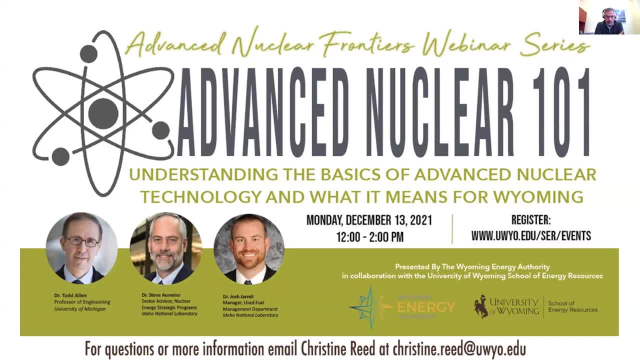 and it's been a very steep learning curve- is that it's much more than simply a test reactor, And we've learned that through consultation and engagement with our colleagues at Idaho National Labs, which has been a tremendous benefit to the state. It's also been a tremendous benefit to me personally. 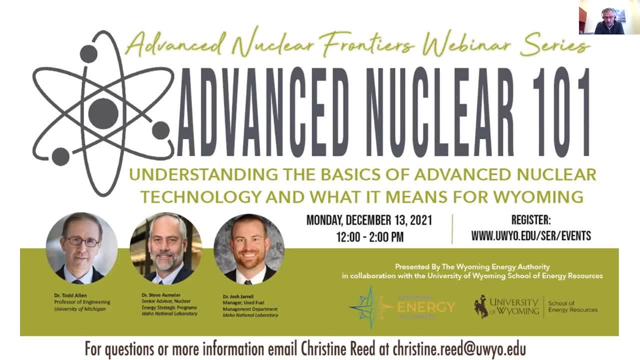 but many of the people in the state have really benefited from having a conversation with our colleagues over there, And one of the things we've learned is simply that it's not just reactor, it's not just electrons and it's not just Wyoming. 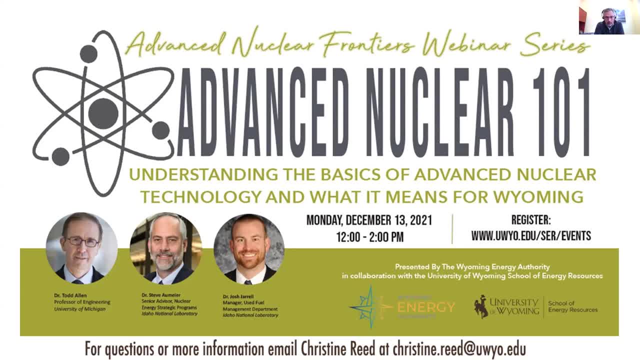 So what do I mean by that? Well, I think we're probably going to learn a lot about that from the panelists, But to give you a quick idea, it's not just a reactor. it's all about other value chains, manufacturing. 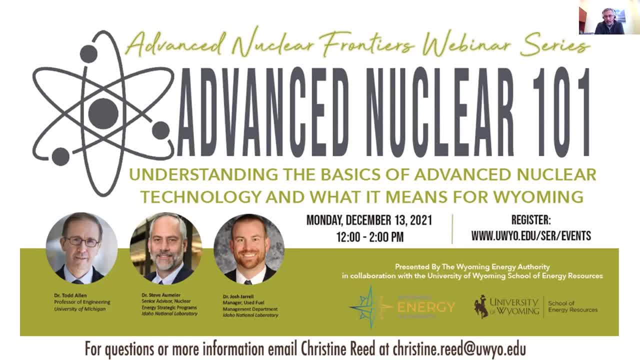 Something about these new advanced reactors is that the business case is built on being able to produce many of them, rather than just one big reactor. You get economies by producing more and more and more of them, So there's a manufacturing opportunity there. Wyoming has a lot of heavy manufacturing capabilities. 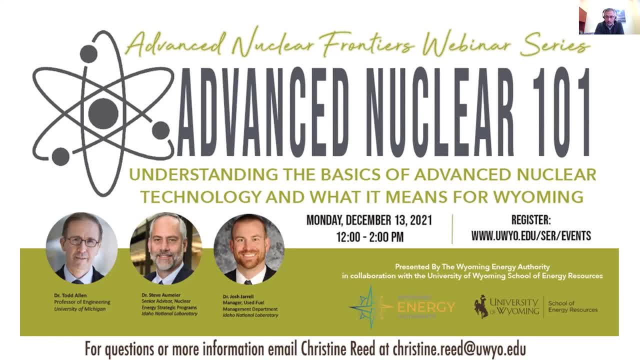 built on the back of the coal, oil and gas sector for the last four or five decades or so, So there's a lot of capacity and this represents an opportunity for them to build out of that traditional sector. There's also a fuel cycle opportunity there. 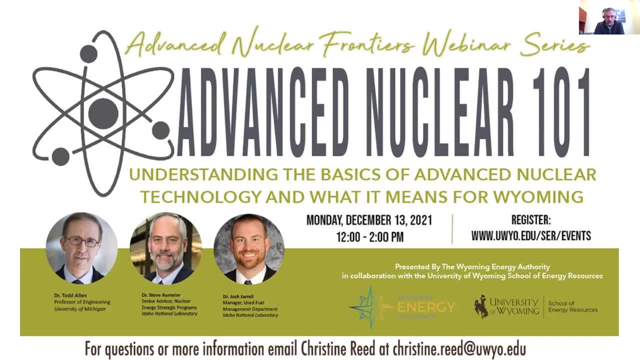 Wyoming has a rich history with respect to uranium mining, but that's only one very small part- well significant, certainly- of that, But it's a small part of the entire fuel cycle value chain that is ripe for taking advantage of. So you mine uranium, but you have to mill it, enrich it. 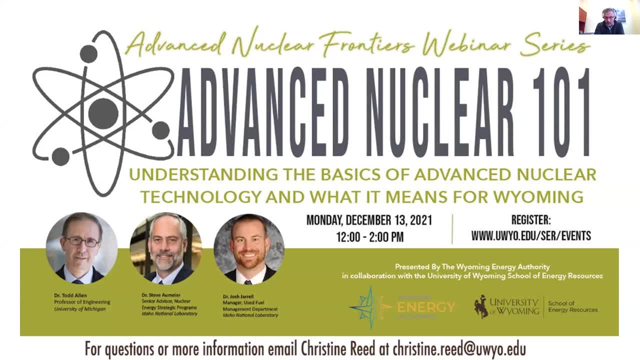 actually produce the fuel for these reactors, And that's certainly an opportunity for Wyoming as well. And perhaps the greatest opportunity really is how these advanced reactors with respect to being able to provide high-quality heat and power most critically, with zero emissions. 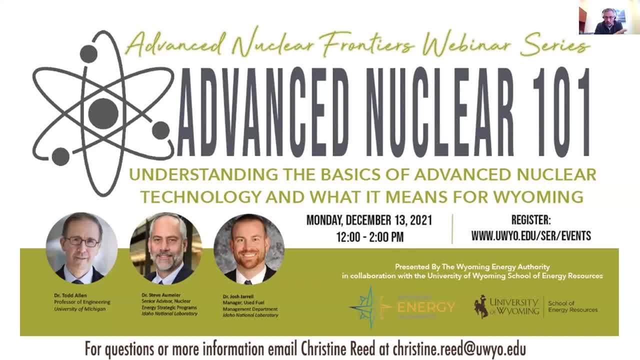 how that integrates with the energy rates into a low-emissions energy economy in the future and contributes to the development of synthetic products and with a ton more added value and other things like that. The final thing is simply that the advanced nuclear opportunity is. it just aligns very, very well. 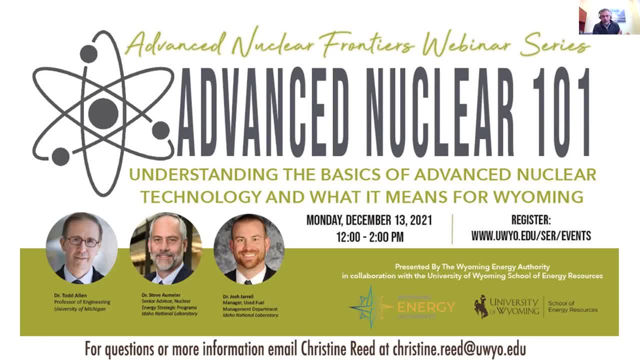 with the vision of the strategy. The vision is to transform a traditional economy in a way that remains relevant, that remains sustainable in a future decarbonized or low-emissions world, And it adds a ton of value and richness to this energy economy that we're very, very proud of. 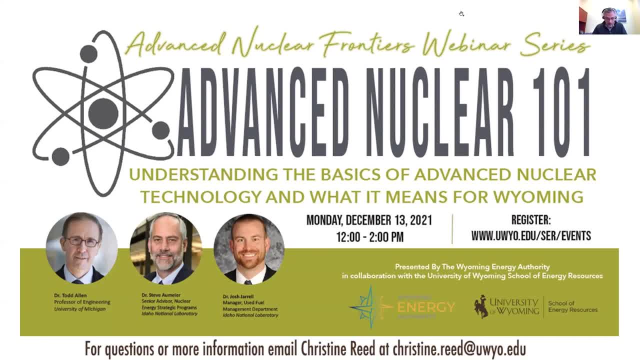 So with that, that was a brief, very brief introduction, I admit, but I want to hand it over to the panelists who are experts in this area. And to start with, I'd give a very warm welcome to Dr Steve Omeyer from the Idaho National Lab. 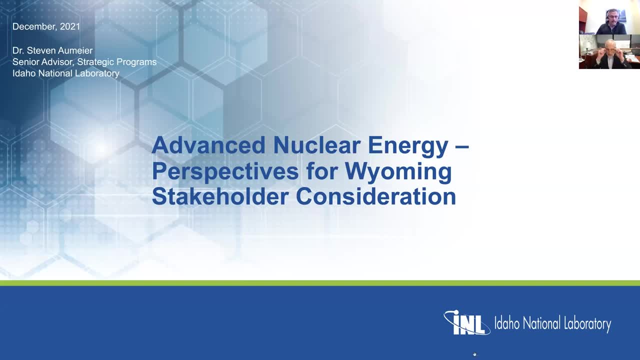 Steve over to you. Thanks, Glenn. So do you want to jump right into the presentation Or have us introduce ourselves first? Well, I think you just introduce yourself and then go into your presentation, and we'll work it that way through the next three. 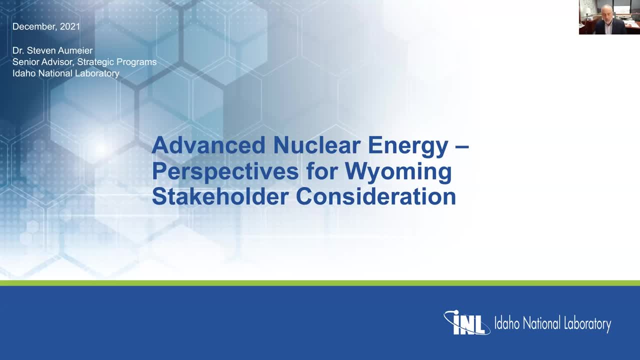 Sounds good. I appreciate that. So my name is Steve Omeyer. I'm a senior advisor here at Idaho National Labs. I am not from Wyoming, but pretty close to it, So I was born and raised a couple hours from Kemmerer. 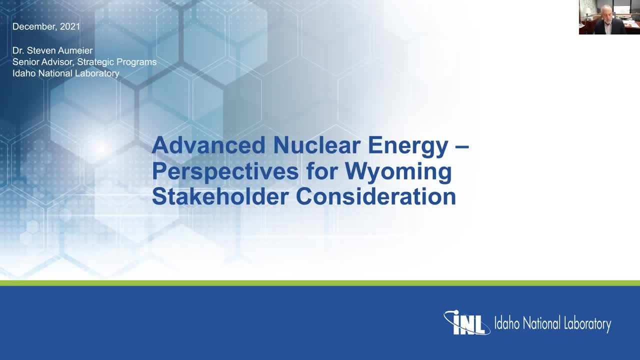 in Southeast Idaho, grew up in that part of the state, went to school, went to school here in Southeast Idaho And that's where I got familiar with, had an opportunity to work for the National Lab Argonne National Lab at the time as a summer student. 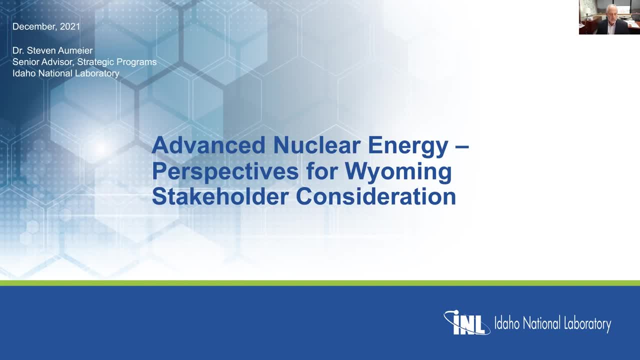 So that was my introduction to all of this advanced energy research. And then I went on to go to the University of Michigan, which is the largest nuclear engineering school in the world. From there went on to left the state, went to graduate school. 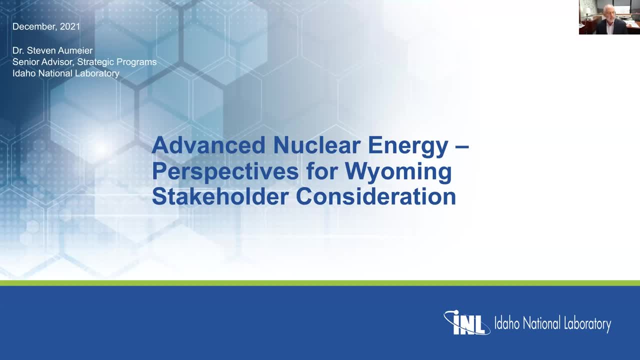 got a PhD and what I'm proud to say is the best nuclear engineering school in the country, and that's University of Michigan. Along the way, I also went to University of Chicago and got an MBA, Found my way back to Idaho about actually 27 years ago this week. 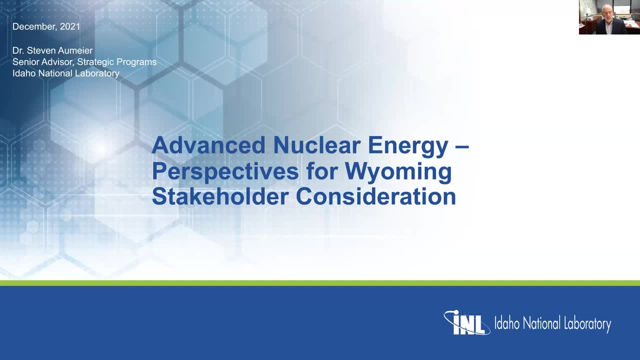 I came back to Idaho I had the past roughly three decades been working in pretty much evenly split between advanced nuclear energy. what I'm focused on right now- national security applications and issues related to nuclear and radiological science, especially counterterrorism and also nonproliferation. 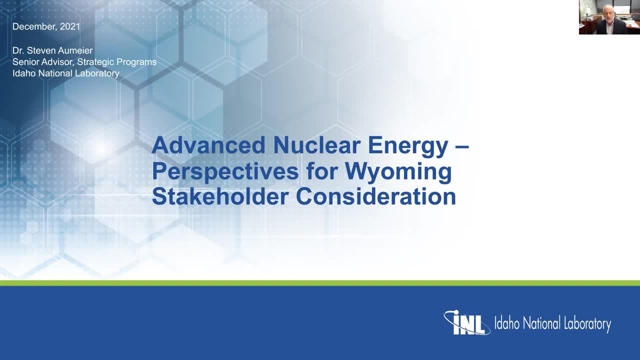 And the third area That I've spent quite a lot of time on is renewable energy and advanced manufacturing and the intersection with that, with energy systems. So that's who I am and where I've been the past 55 or so years. So I appreciate the opportunity to have this conversation. 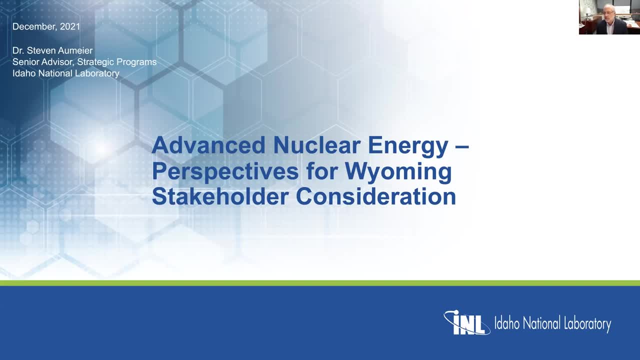 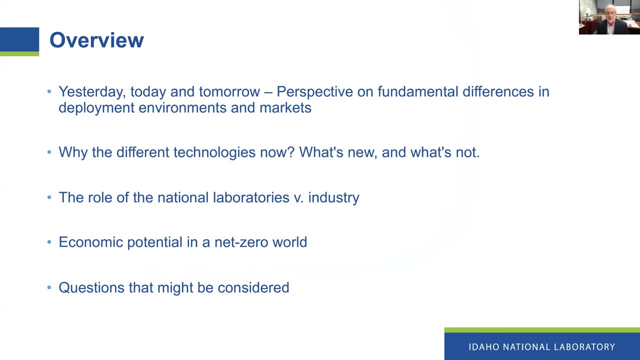 and share with you just some of the perspectives. Christine, If you could advance the slide, Just share with you some of the perspectives I think might be of interest. Hopefully it'll answer some of your questions, but mostly maybe give you an idea of where. 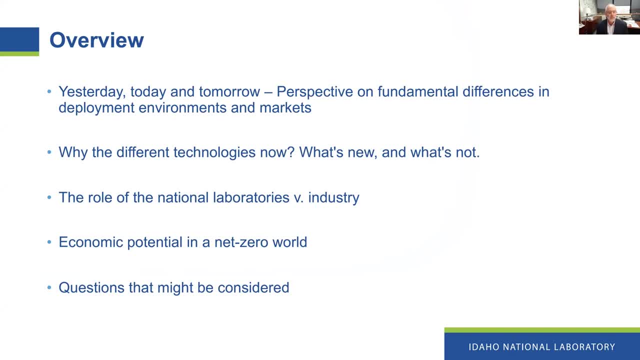 to ask questions for the future and also where you might want to spend some additional time digging in a little deeper. So I want to talk about really what's different with the markets that nuclear energy is. Thank you, And I think that that's really a big part of what 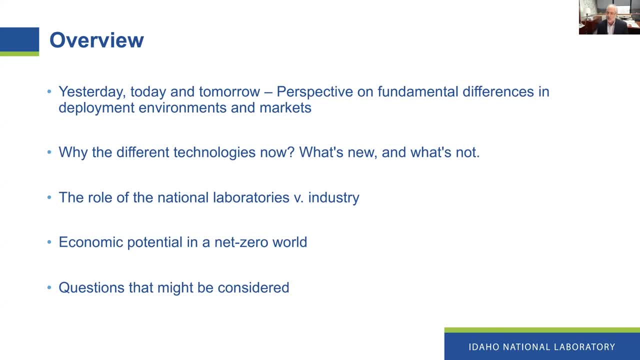 the energy goes into in the future. It really is a different way forward than we've experienced in the past And it's important to sort of have that picture of what's different going forward versus, say, 50 years ago and even 15 or 20 years ago. 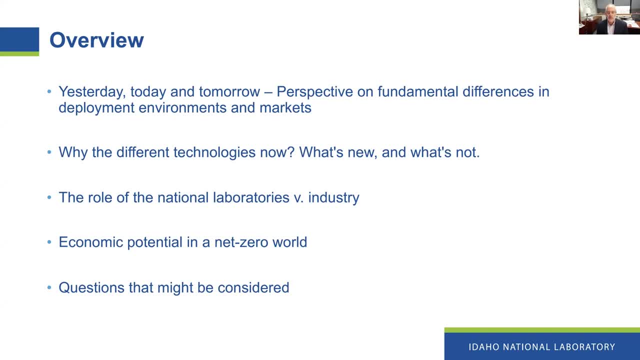 That explains a lot about why you see different technologies um coming forward today, um, and also we can talk a little bit about, really, with those technologies, what's new and what isn't new. uh, there's, there's a lot that's been done in the 65 plus years of. 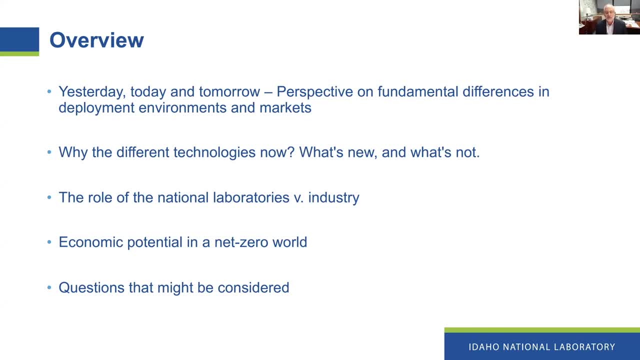 commercial nuclear energy. so not everything that you see today is new, but it might have new, new applications. i do want to mention a little bit about the role of the national laboratories, especially in advanced nuclear energy, versus the industry, versus, uh, the government itself. uh, that's, that's important to understand, and also then talk a little bit about, uh, what, what glenn? 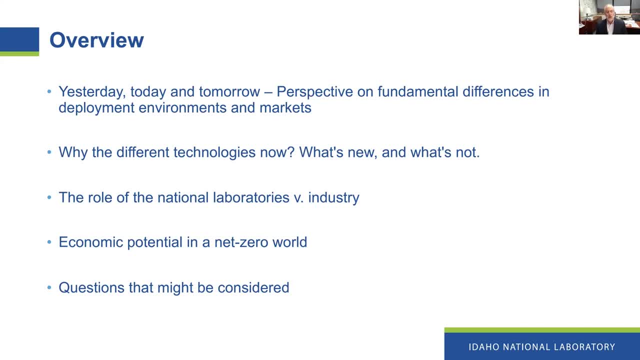 began to to scratch on maybe what? where is the economic potential of nuclear energy? uh, especially nuclear energy for wyoming? uh, in this evolving world of traditional nuclear production? and sorry, butwhat's unique about climate change is that choose to think that we're going through very phase one period of climate change. 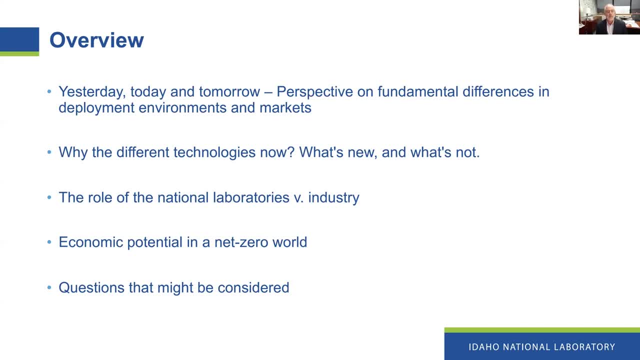 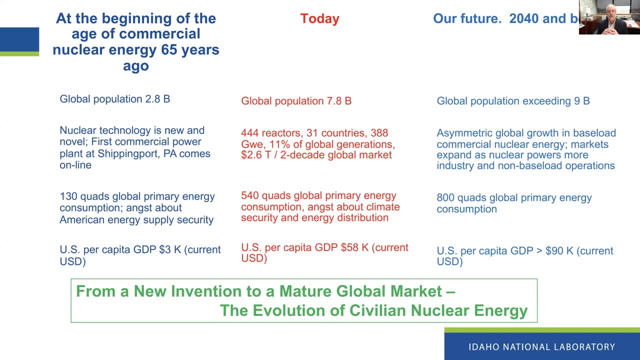 and you know uh m завu, the echo of climate change, uh first commercial nuclear energy plant was built um. it was being built and nuclear energy was conceptualized really for uh, for the market of that day, very fast growing um electric energy demand. it was a brand new technology there. really there were not the uh, the, the uh operational uh. 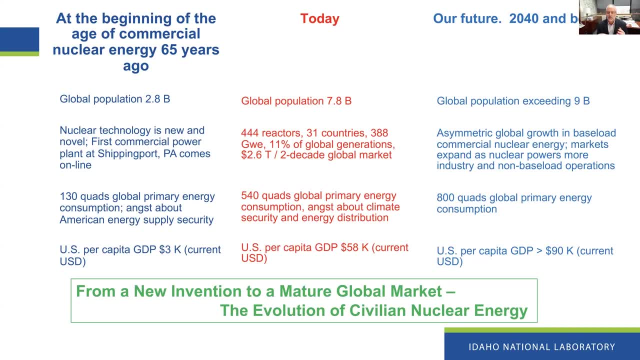 cultures and approaches put together. yet there wasn't uh, there was just beginning to be uh, export uh rules and regulations and and and the such. so brand new technology in a post-world war ii uh era, and keep in mind at that at that time, uh we um globally. 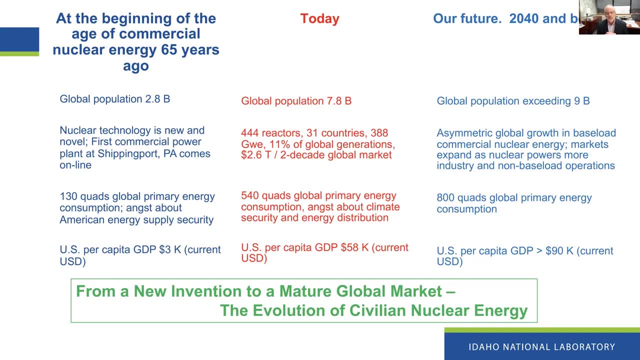 the uh the big. we were consuming about uh four times less energy than we consumed today. uh, and even today we're looking at a growth in energy consumption uh by about 50, just uh, just in the next 20 years. so so fast forward from this brand new technology. 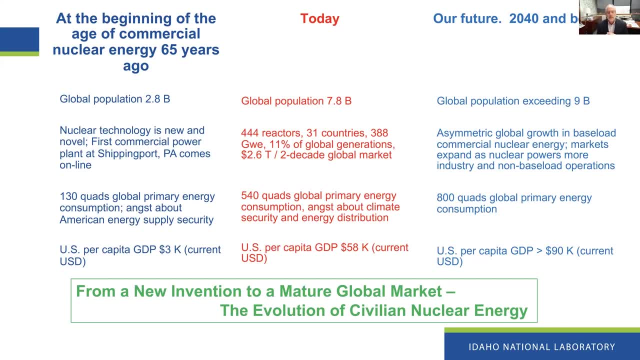 uh, the first commercial application. uh, very different world to today. there's about 440 450 reactors around the world producing about 10- 11 percent of electrical generation. um, have a number there on what, the, what, the markets for nuclear technology and associated operations, fuels and and everything: 2.6 trillion uh over. 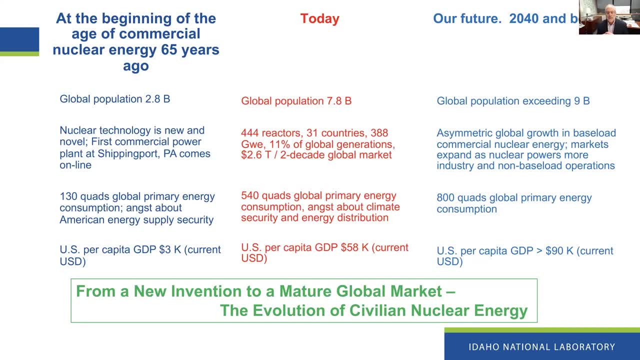 the next two decades. i just saw a number, um, actually just last week um, that put that number at about eight trillion dollars uh over the next uh two to three decades. so uh the the bottom line here is there's a mature, a very mature nuclear industry uh out there globally. 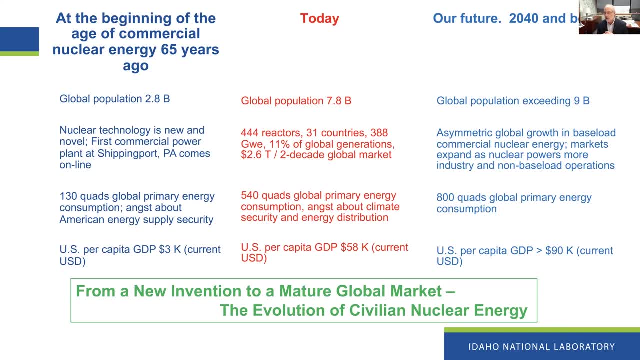 it's not going away, it's um, it's only growing, especially with um, with net zero goals of various countries, not just for prime primary energy production, but products that the energy feeds and as we look forward again to, i always think about a world of of nine billion people. i mean think about, think about what that means in terms of the 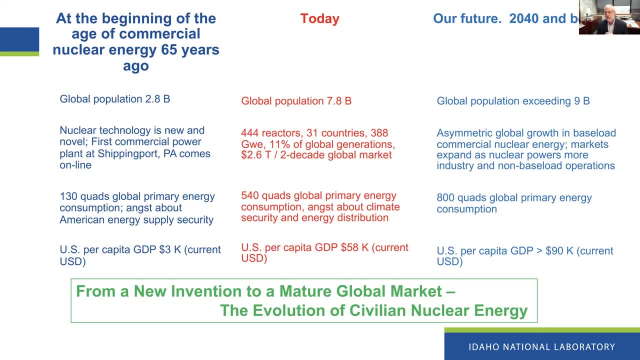 environment, in terms of energy demand, in terms of um of of markets and stability around the world, um, and, and that's what frames, uh, really frames- my thinking about advanced nuclear energy, is where we've been, where we are today and and where we're likely to be in the future. so next slide. 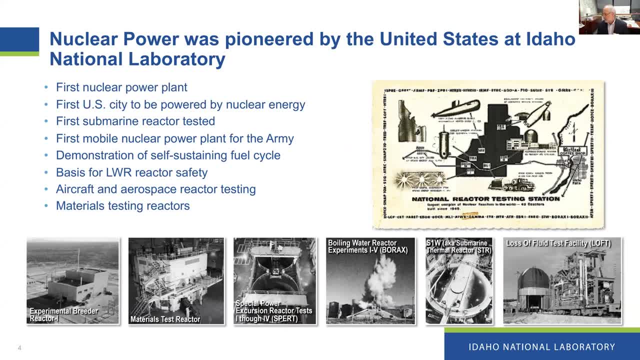 uh and as nuclear energy over the past 65 years grew into this global multi-trillion dollar uh enterprise, is producing a good portion of of electricity around the world. the lab, the national labs and, with respect to nuclear energy, uh, what is today? the idaho national lab, really played a. 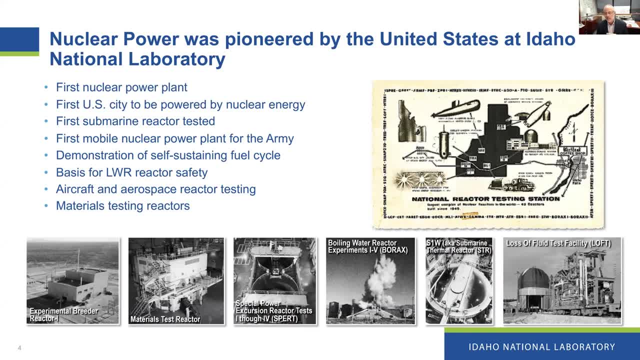 very significant role. so, uh, a boss of mine used to like to say, uh, that the labs do what? what? industry, uh, academic, in academia, can't, won't or shouldn't. um, and that's really the role of the lab. lab isn't here to to sell anybody any technology. we're here to. uh, we're here to innovate, to create new, both. 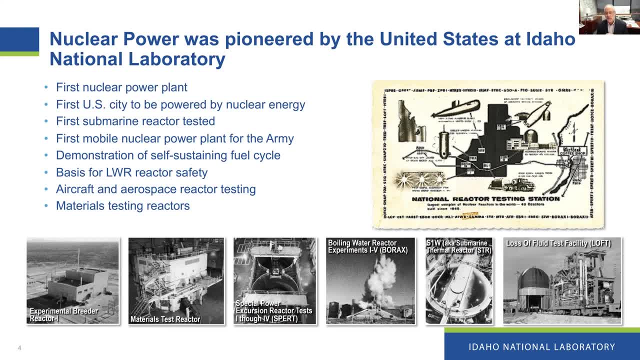 fundamental technologies but also the enabling science that goes goes with that, but also test and validate and feed that testing validation back into the regulatory process, back to uh industry and and uh in government so they can make informed decisions about where to go with technology and also work with the universities. 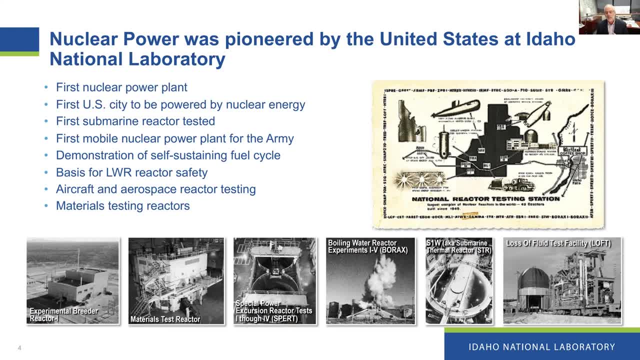 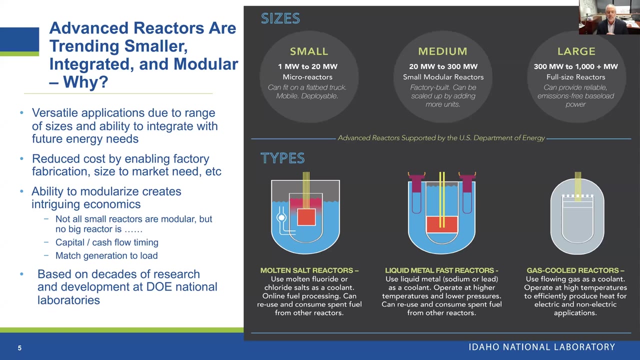 to spur innovation. so uh, so the lab, uh, this laboratory uh has had a huge role uh in in in building up, helping uh establish that, uh that framework for what is today global uh global nuclear commercial nuclear uh industry uh next slide uh so so. so today we we see quite a lot and we hear quite a lot about advanced nuclear technologies. 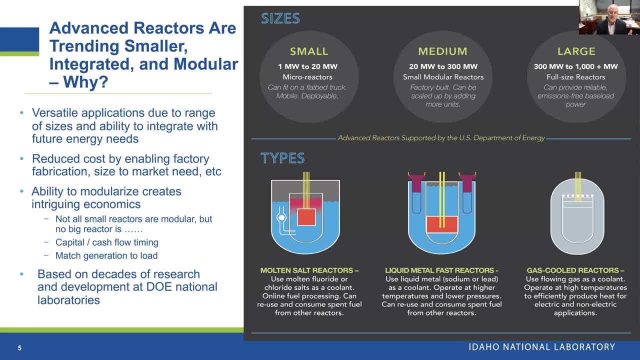 and and typically uh, the difference between what we saw in the past and what we see today in terms of commercial uh, interest is focused on two things: one is on size and the other, uh is on simplicity, and in many cases those two things go hand in hand, and simplicity translates, can translate. 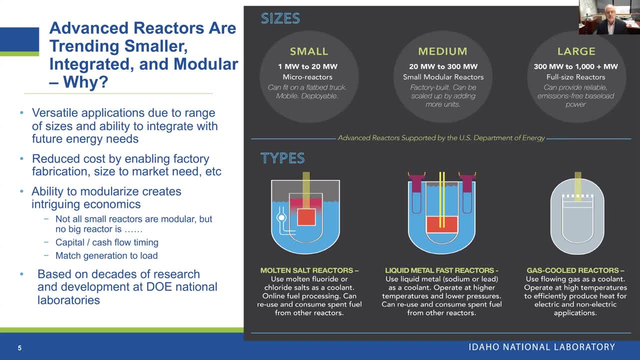 into even safer systems. you have extraordinarily safe systems now. but simplicity helps in both the economic um施設 as well as operations of those machines. And we think in sizes, in kind of small, medium and large, and I show some numbers up here. 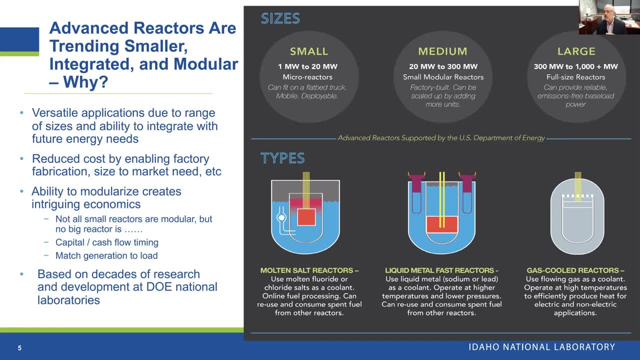 These aren't meant to be absolute cutoff points on what's small, what's medium and what's large. In fact, many people consider very small reactors, micro reactors, to be up to 50 megawatts in electrical Generation. then you have the medium sized reactors. 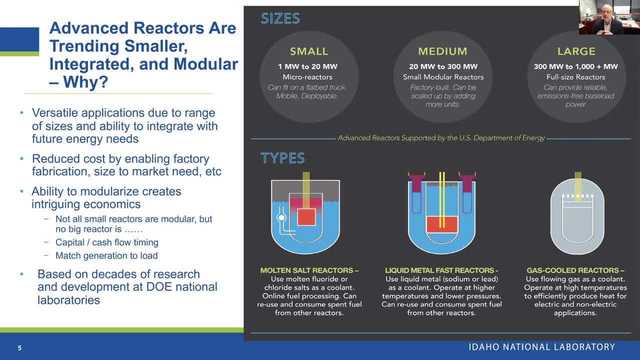 you know that might be 50 to 250, 300 megawatts, And then you have large reactors. Well, why is that important? It's important because, just like you see in other industries that have matured, the nuclear industry has matured. 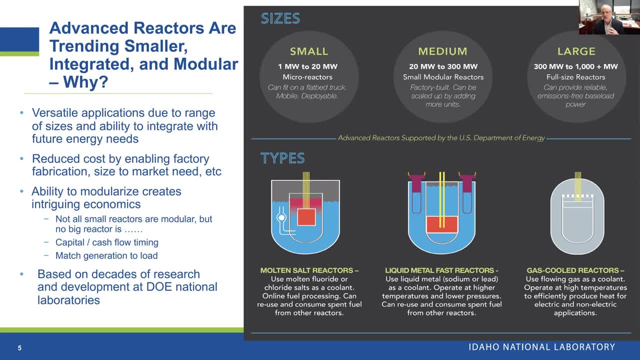 and is then moving beyond generation one and two and three technologies To better match technology type to the actual application that's needed and also advance the constructability of the machines. I think about this in a similar way as I think about the aircraft industry. 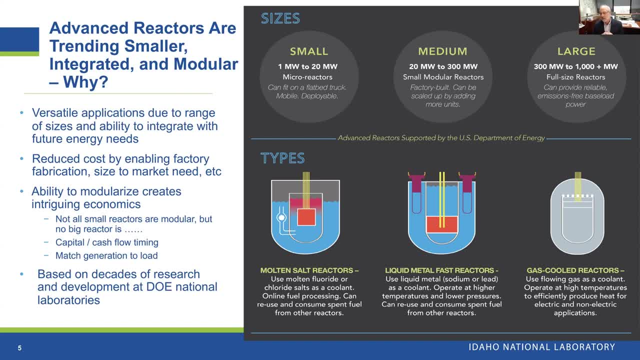 how they've aircraft have really segmented the markets based on size, based on range, So you can optimize the technology to the application. Again, you see that across a number of the industries as they mature- and nuclear industry is no different- You also see modularization of those technologies. 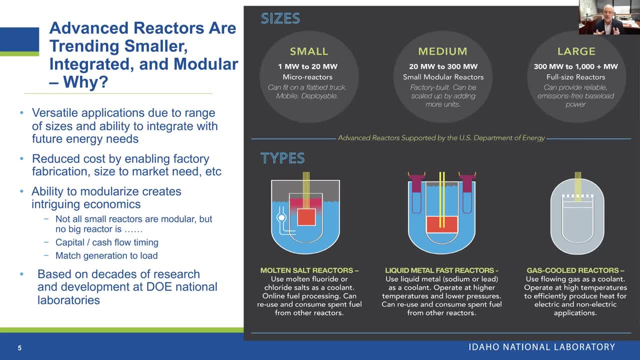 And we'll talk a little bit about that in a minute- And that can really help in terms of efficient deployment of capital resources: matching a technology, size and constructability to an actual application, Not tying up capital for 10 years of construction. And also we'll talk a little bit. 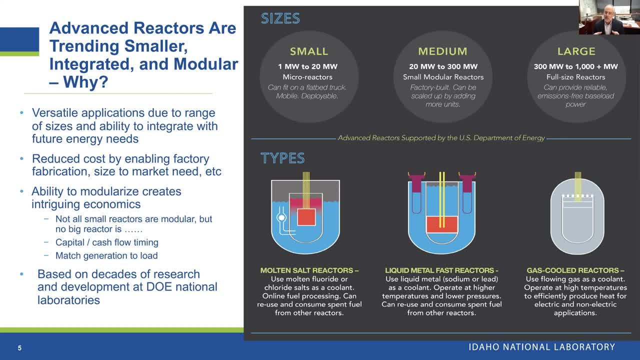 about matching generation load. But all of these reactor classes have very deep roots in the national lab and academic areas. But with the national labs there's been a lot of testing validation on these classes of reactors, some more so than others, And we'll talk a little bit about that in a few minutes. 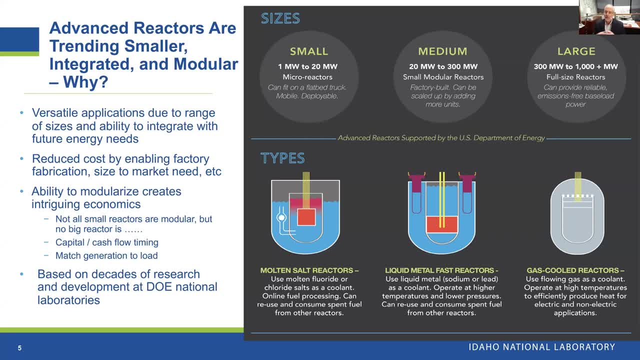 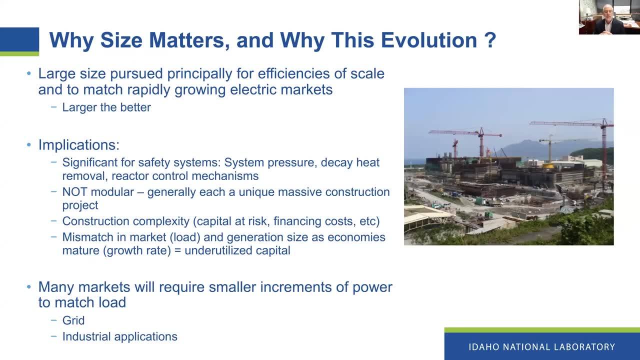 So that's kind of why you see these different types of machines coming out now. Next, slide Size does matter And I wanted to just dig on this a little more. So early on in the nuclear era, actually, the first reactors were relatively small. 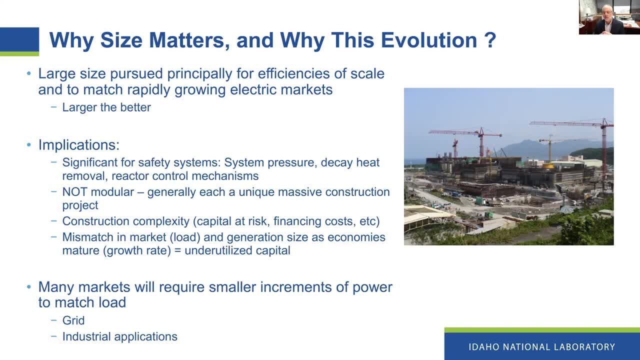 The commercial nuclear reactors were relatively small, in the order of 60 megawatts. But for the purposes of economies, or efficiencies, I should say of scale, the machines got bigger and bigger and bigger And today many of the reactors are 1,000 megawatt electric. 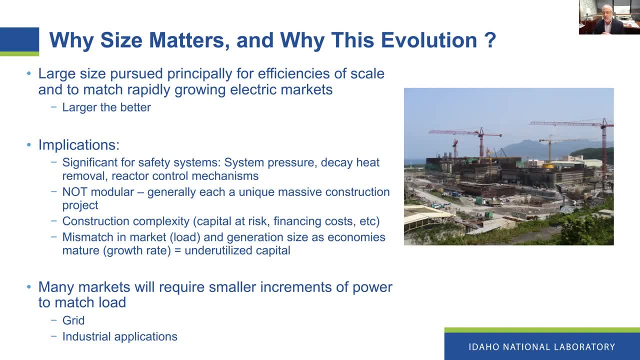 They go up to. I think the new European reactors are 1,600, 1,700 megawatts And that has a lot of implications for the system and how it's designed With light water reactors when you have systems at large. 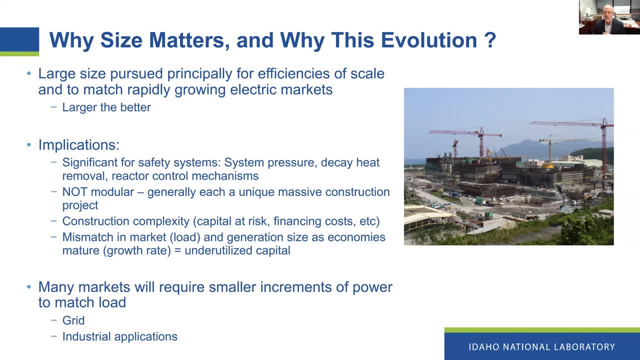 they're high pressure systems. You have to put all kinds of engineered systems for decay, heat removal and safety purposes, And these are most. They're definitely not modular systems. These very large reactors are generally a unique construction, a huge construction project in and of itself. 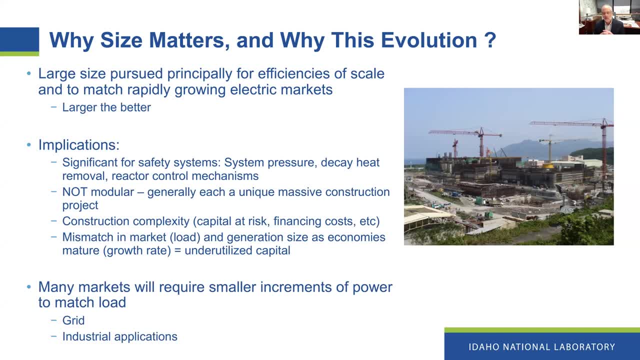 And just the nature of that construction project means you're putting a lot of capital at risk for a long time. There's financing. Financing becomes an enormous issue And there's a risk premium to be paid If anything goes wrong in construction. you're going to get delayed. 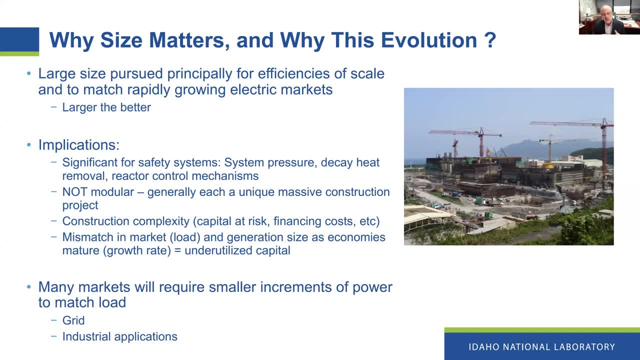 There's also something else to keep in mind. As economies have matured as well, you can see in the United States the demand for electricity has actually gone down. The rate of growth has gone down markedly over the past 60 years that nuclear energy's been here. 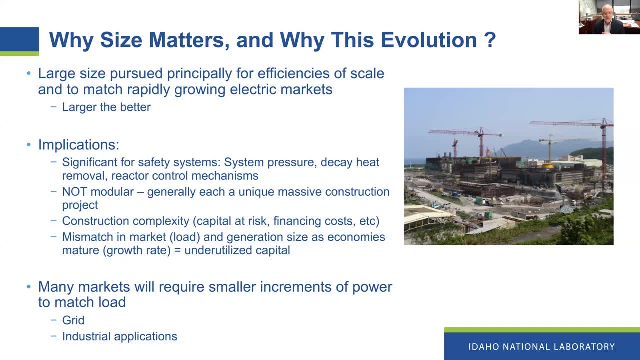 So sometimes it really doesn't make sense to drop 1,500 megawatts new generation- Or if you're talking about a multi-reactor plant, you know multiples of that- into a market all at once. It makes much more sense to incrementally provision. 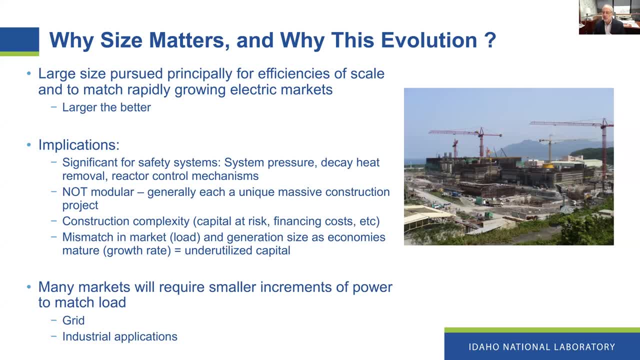 the amount of generation needed with smaller, bite-sized pieces that are easier to build. So in this regard, especially in these regards, size really does matter, And we're at a point now where we can size the machines much better to meet the different types of markets. 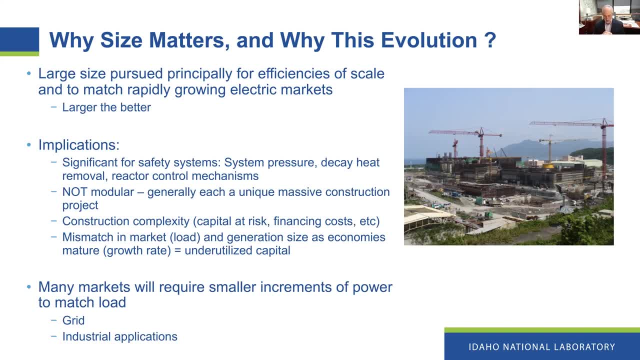 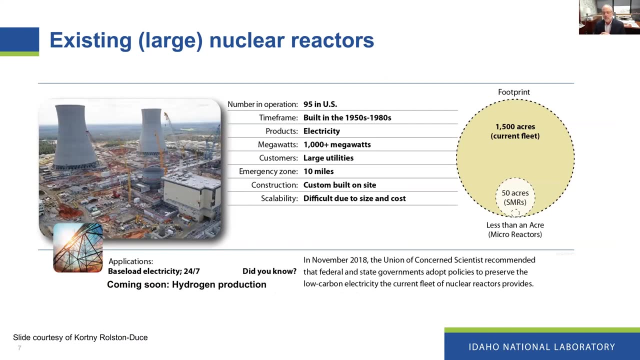 which are electrical generation that we'll talk about. maybe more interesting, non-electrical uses of nuclear energy as well. Next slide. So let's just walk through real quick, these types of reactors, And I can make these slides available to you if you want to take a look at these more in the future. 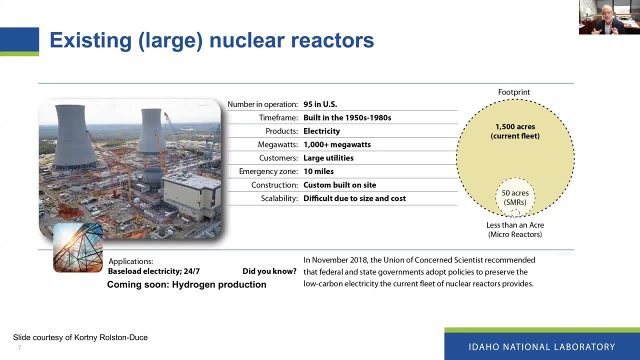 as well. So very large reactors, Like I said, huge, massive construction projects. They have very large exclusion areas So the physical footprint that those reactors take up are very large. It doesn't mean we shouldn't be considering where to build large reactors. 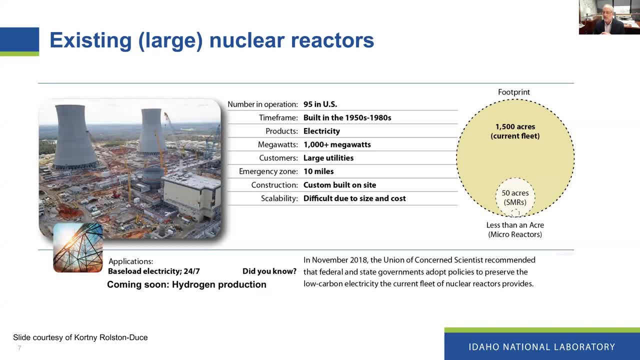 Especially around the world. many populations are energy poor and they need big pieces of generation Like that. But these are big, massive construction projects with big footprints. I should have had a notation on water use in nuclear. I've gotten that question several times. 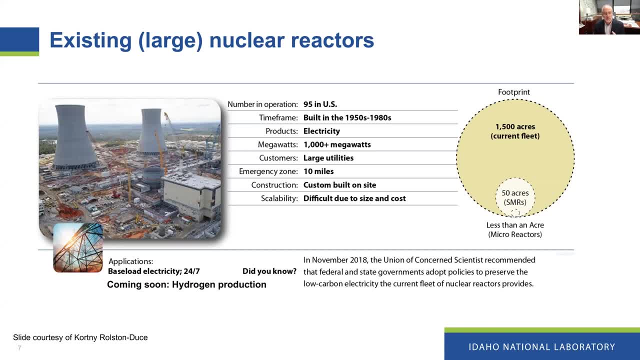 And water use in any thermal generation, whether it's coal, whether it's gas plants, whether it's nuclear, it really doesn't matter what energy source you're generating, Right, Right, It's just the amount of water that you're using to generate the heat with. 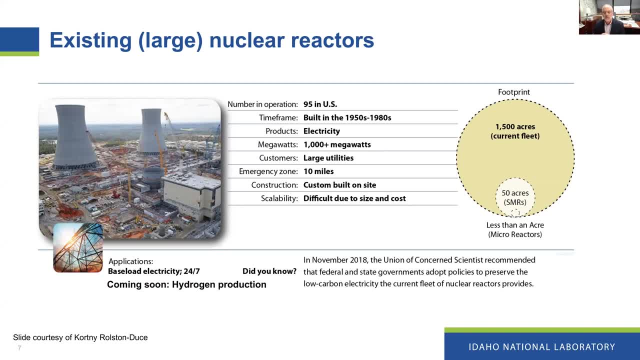 The amount of water used is a function really of the efficiency of the system. So with nuclear in general you can think about nuclear taking on the order of 700 to 800 gallons per megawatt hour And you're going to see actually a little less water use. 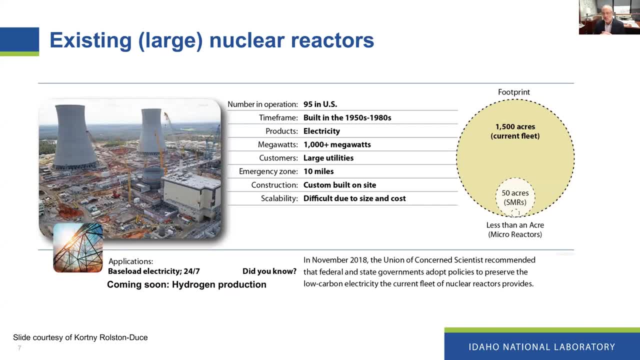 with advanced gas plants because they're more efficient. You see about the same. You see about the same amount of water use with solar plants. So, again, it doesn't matter what the size of the reactor is in the number of gallons per megawatt hour. 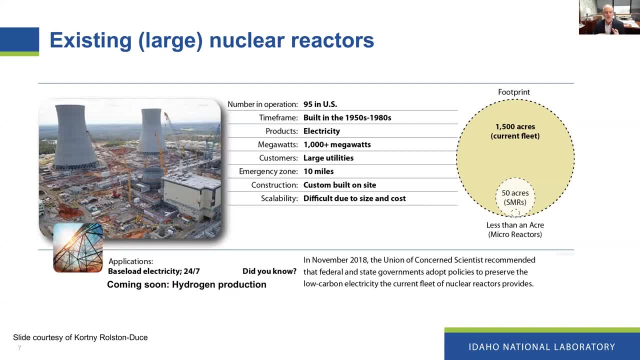 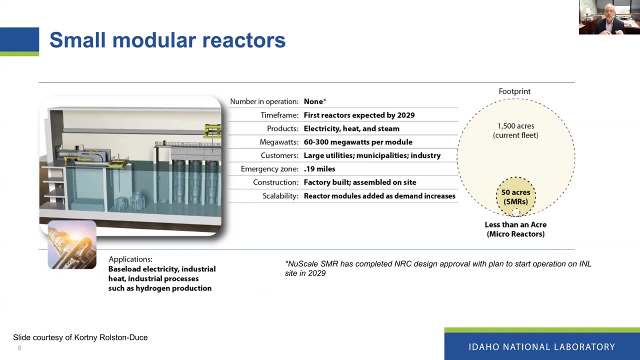 It matters how efficient it is. So that's just something to keep in mind with any electrical generator- thermal electric generator Next slide. So small reactors, and we'll talk about small and modular. These are a couple of different considerations, But small modular reactors are something. 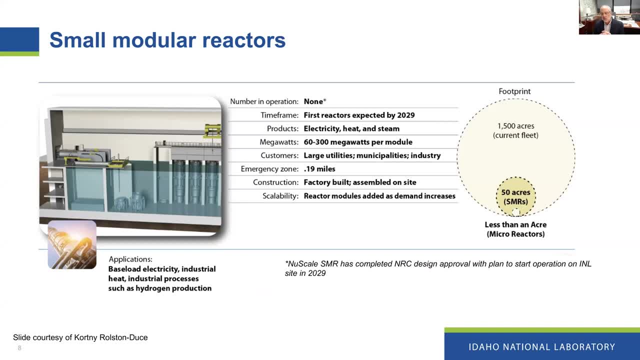 you hear quite a lot about right now. They have much smaller physical footprints that they take up because of the bite-sized pieces. if you will, that you put a plant together with Much more, in theory, more efficient to fabricate, because the reactors are actually. 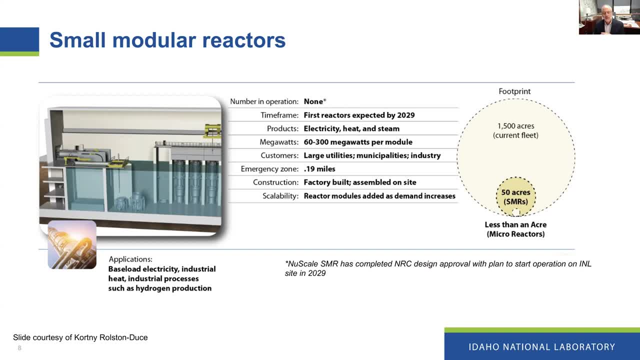 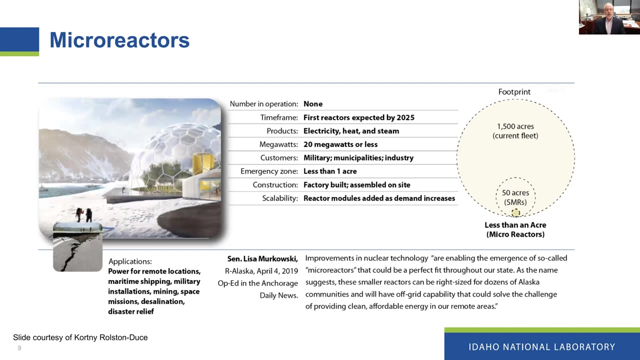 factory fabricated, although you still have all the capital construction that is required to put together the physical infrastructure. But these reactors, again on the order of 60 to a couple of hundred megawatts electric, much smaller footprint, Next slide, And then a really interesting class of reactors. 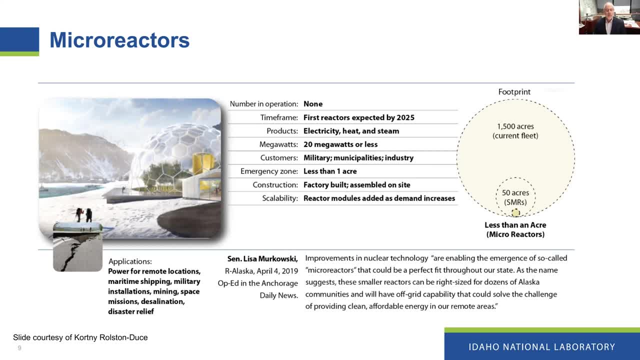 for a lot of different applications are what many people don't know, What many people call micro-reactors or very small reactors. So the notion is really 50 megawatt electric or less where you can put. these systems are meant to be factory fabricated, but also more of a cartridge. 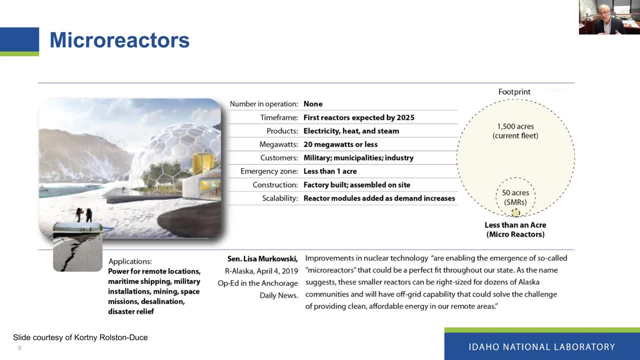 core typically So when they tend to be envisioned as having longer lifetimes, up to 10-year lifetime. So when the core is expended, you take that and you store it where you would used fuel. then you replace that with another core. 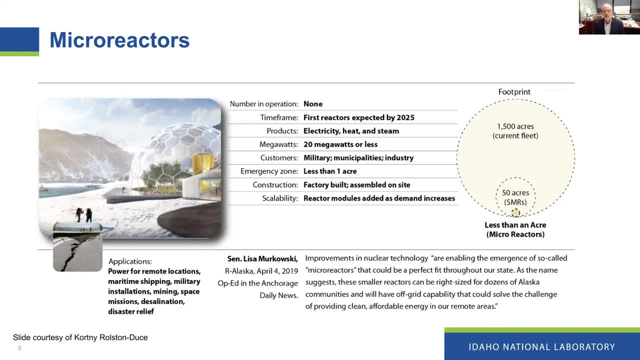 So some people call this a nuclear battery, Some people have called it a quantum battery approach where nuclear energy just becomes a plug and play sort of power of either an industrial process or a remote location mining applications. Next slide So you can see the. 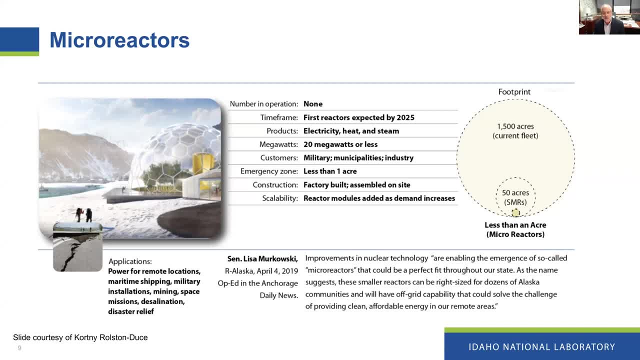 very, very small footprint for these types of reactors And there is just a heck of a lot of interest in those now. Actually, you'll probably see one of these will be the first demonstration projects That you'll see here at the lab, probably within two to three years. 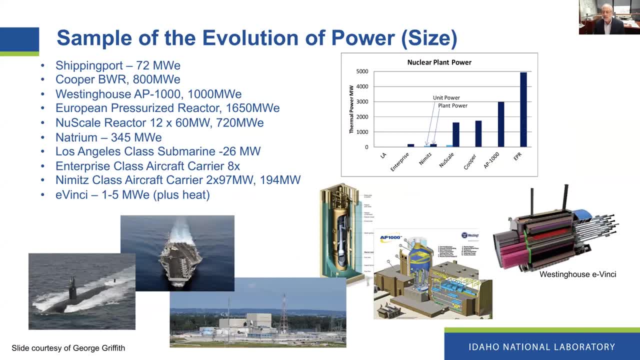 Next slide. Just a quick note on the number of different applications that you've seen across this spectrum of reactors. So those classes of reactors are not new in and of themselves. I mean we've built, we the collective, we have built and operated the smallish commercial. 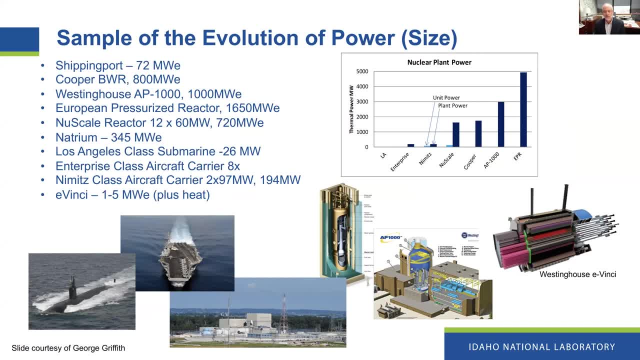 reactors. The shipping port reactor was the first commercial nuclear reactor. Then they've gone to kind of a medium-sized. the example is a Cooper boiling water reactor at 800 megawatts. Today you see large 1,000 megawatt Westinghouse AP 1000s. 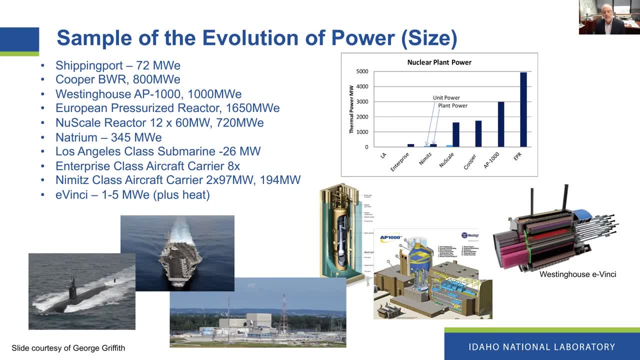 I mentioned the 1,600 megawatt reactors. Well, what about small and medium reactors? Well, we've operated Those swell many, for example, in the military realm, 20,, 40,, 80,, 90 megawatt reactors are powering ships. 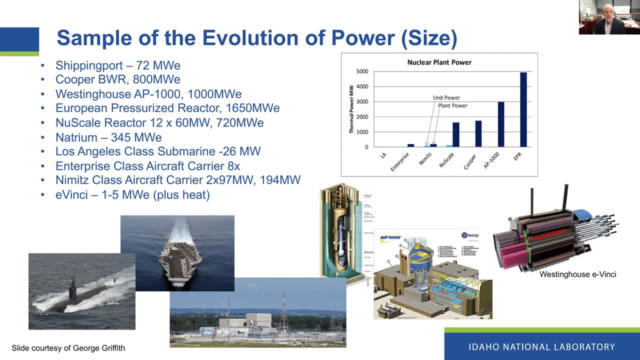 all over the world and for other nations are powering commercial and icebreakers and all kinds of different vessels. And then in terms of test reactors- we'll talk about that in just a minute- There's been quite a lot. There's been a lot of built and operated as well. 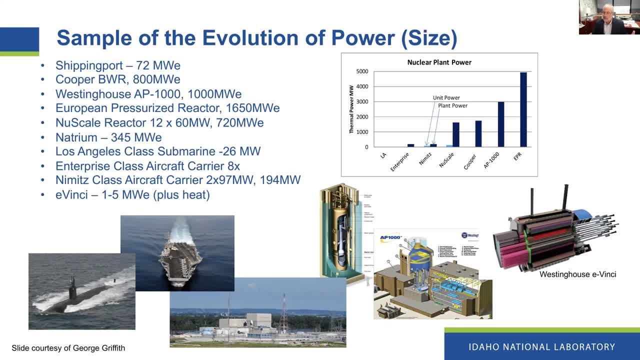 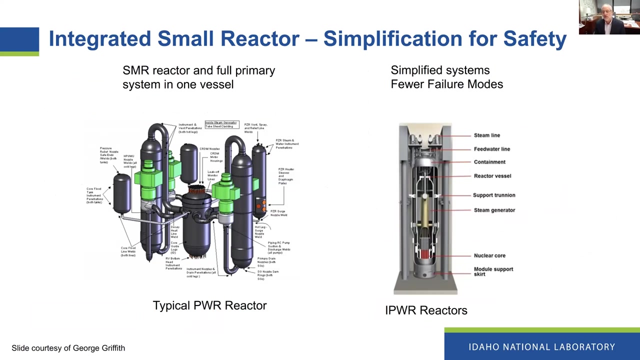 So there's been a lot. There is a lot of experience building and operating very small, medium and very large reactors, But many of the advanced reactors are going back to a thinking of much smaller and much more modular Next slide And the notion of modular reactors, and especially 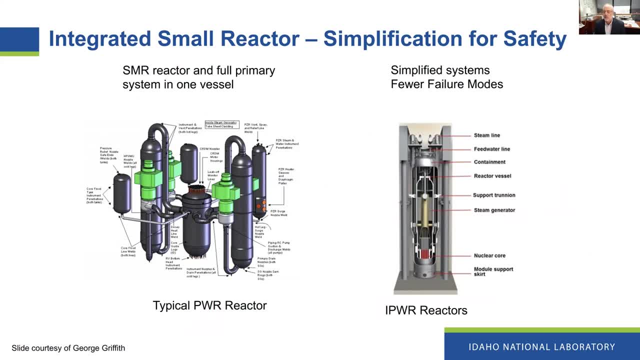 integrated Systems within reactors is really very important. So on the left- and I don't expect people to be able to see the words on this, Actually, maybe you can- That's a general layout of a commercial pressurized water reactor, just in general. 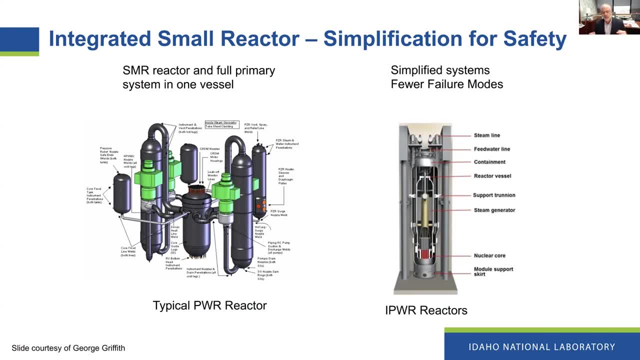 But you can see the equipment that's actually feeding into that central. That's central And That's the granular piece. that's the actual reactor core. Everything else is cooling systems and pressurizers that go on that Well. today, many of the reactor designs 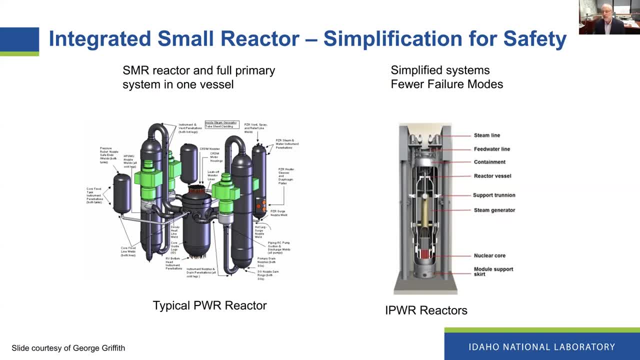 are going with much more of an integrated or integral approach where much of that machinery is actually being placed within the reactor core And there's inherent safety benefits. It's a go with that. but also manufacturability of the system has been shown to be much more favorable. 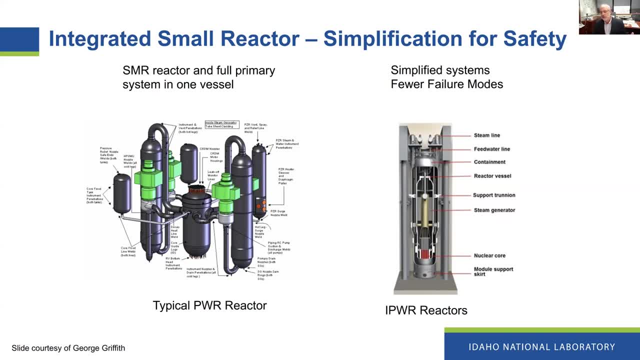 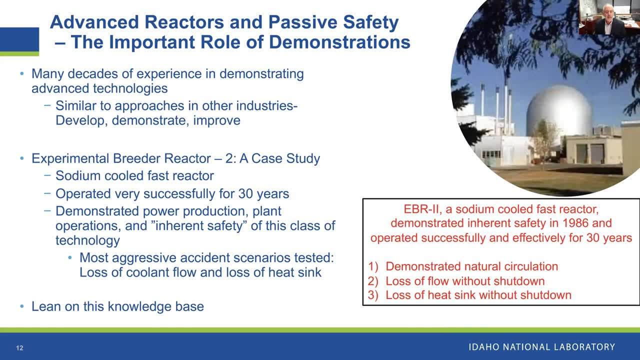 So again, maturation of the technology, learning from the past 60,, 70 years of experience, Next slide And the demonstration and testing that's gone on with systems like that is really important Because there's been again six, seven, actually seven. 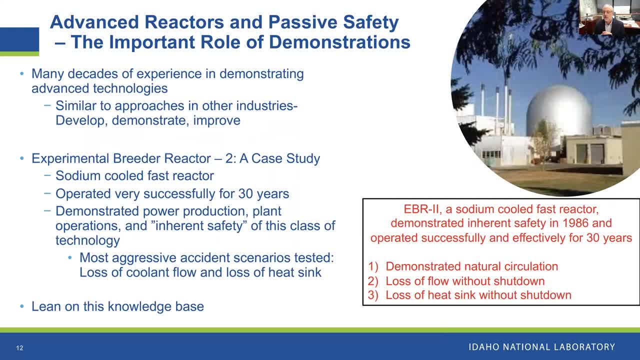 and a half decades of testing, evaluation of different types of reactors, And those demonstrations were important in the past, They're important now And they're going to be very important in the future to continue to mature and improve the technology and be able to incorporate new materials and new technologies. 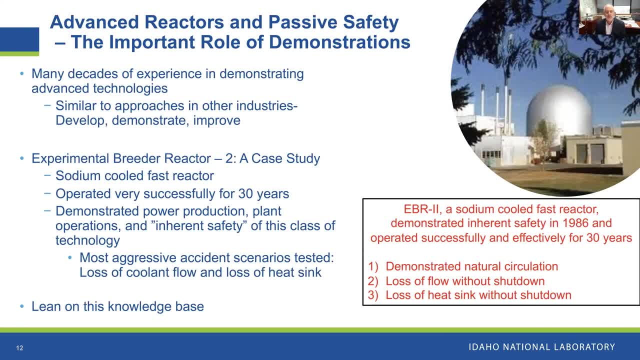 And that's what we're trying to do. Next slide, Next slide, Next slide: New technologies within those systems. And one of the more important ones I think that this group might be interested in is the program I actually grew up in as a student. 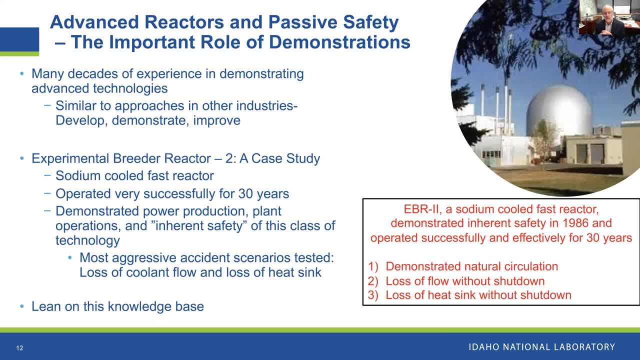 in an early researcher, And that's the Experimental Breeder Reactor 2.. So EBR2 was a reactor that operated here at what's today the Ida National Lab. The site was actually the Argonne National Lab West. EBR2 is a sodium-cooled fast reactor. 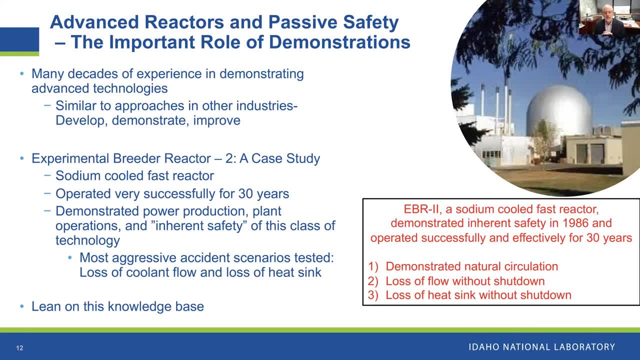 so a pool-type sodium-cooled fast reactor. So you can think of the natrium class of reactors. But this one was much smaller. It was about 20 megawatts, 30 megawatts I think, 20 megawatts. 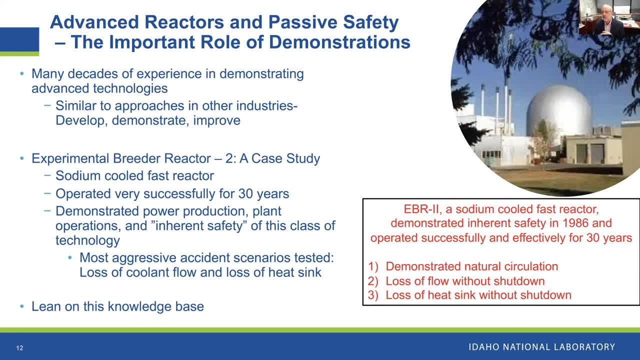 electric, But that reactor operated very, very quickly, Very successfully for over 30 years, Demonstrated not just power production using this type of reactor, but also maintainability operations, set operations protocols And maybe the most important thing was a set of safety demonstration tests. 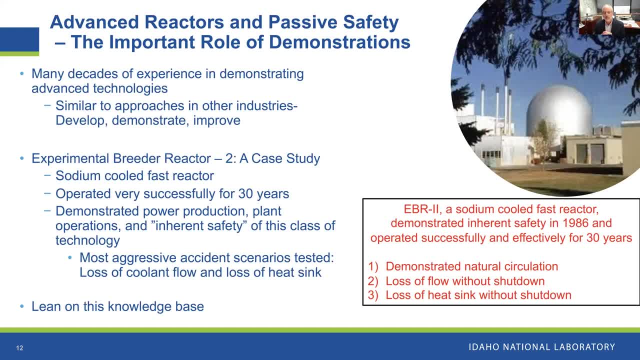 that they did in 1986. And this might be actually a top. I think that you'd be interested in a whole hour of discussion and presentation. So during that safety demonstration test, they demonstrated with actual operations inherent safety. So you'll hear a lot about inherent safety features. 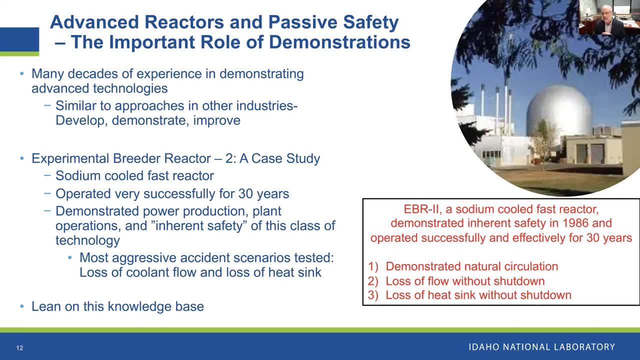 of advanced reactors, But with that system they demonstrated two of the most aggressive types of accidents that a nuclear power plant can have, And that's loss of flow, coolant flow without shutting the reactor down, And then loss of heat sinks So you're not able to shed the heat. 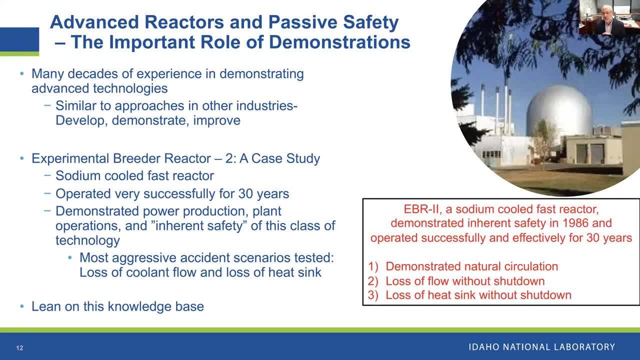 and the reactor doesn't shut down, And in both cases, in a number of other tests, the reactor performed almost exactly as they predicted. Temperature goes up a little bit and there's a negative- It's called a negative- temperature coefficient for the bulk of the reactor. 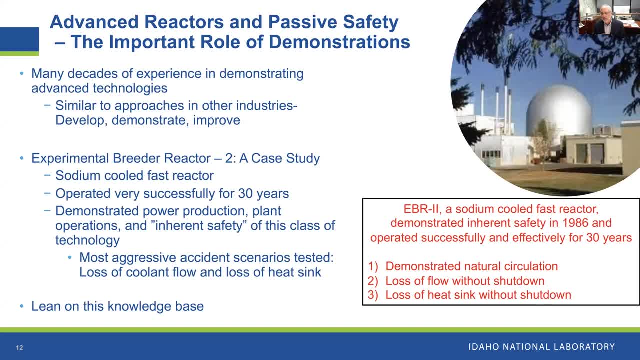 And it shuts a reactor down without any operator interference. So those were really successful tests that unfortunately, many people don't talk enough about what's been demonstrated and tested with those systems. So I wanted to point this out because there's a huge body of knowledge that one can lean on to understand. 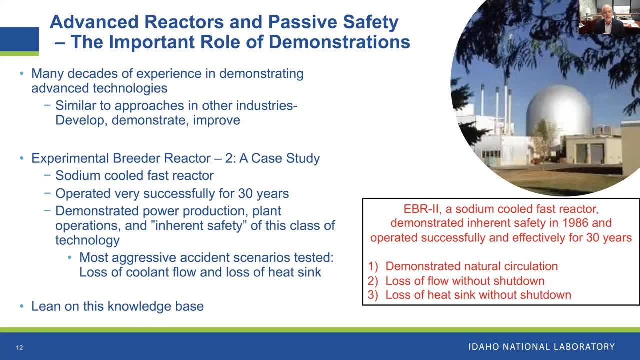 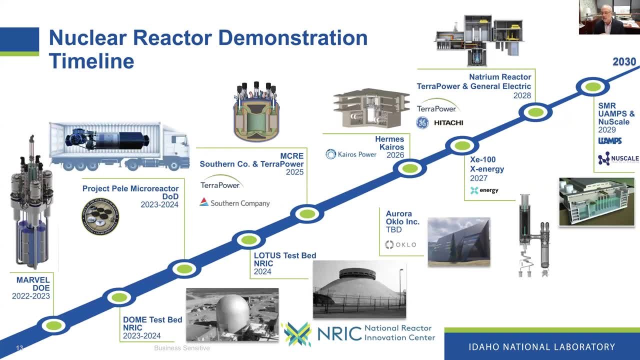 These classes of technologies. Next slide In demonstrations. there's going to be an opportunity to take a look at demonstrations in the future as well, Because they're as important in the future as they have been in the past. So, both on our site here in Idaho and in other sites. 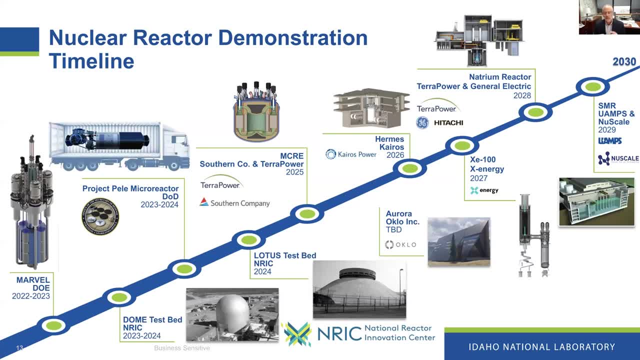 you're going to see different reactors, demonstrating Different maturity of reactors. You should see some very small reactors demonstrated on this site in the fairly near future, And then there's plans for other ones. And Natrium- the Natrium reactor is shown on that timeline as well. 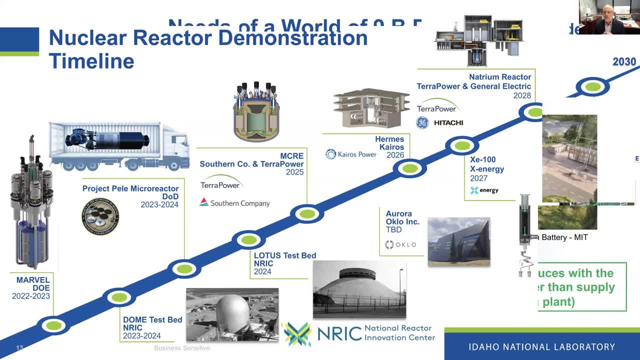 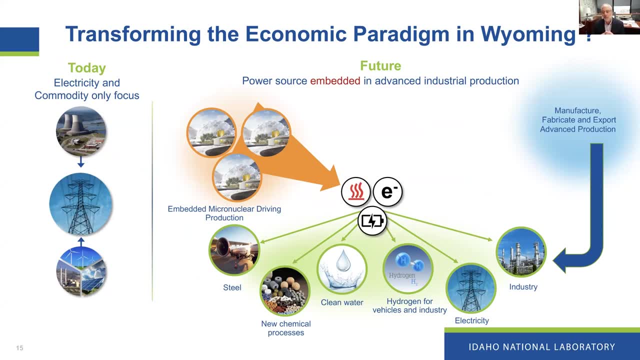 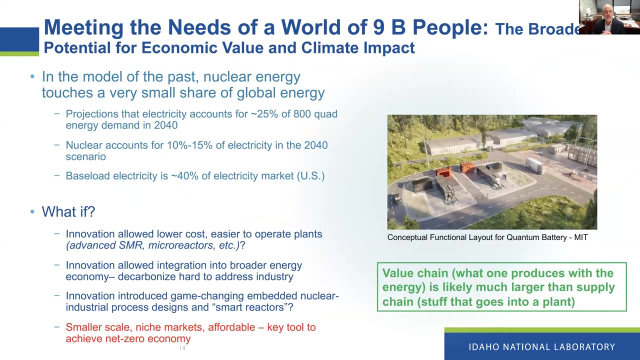 Next slide. So I think You know. So I think electricity production, uh, which is which has been, uh, the focus of advanced nuclear, uh, actually, is there a slide before that, christine? yeah, there we go. so electricity production, of course, very important, especially in the net zero world where much more of our energy consumption is being 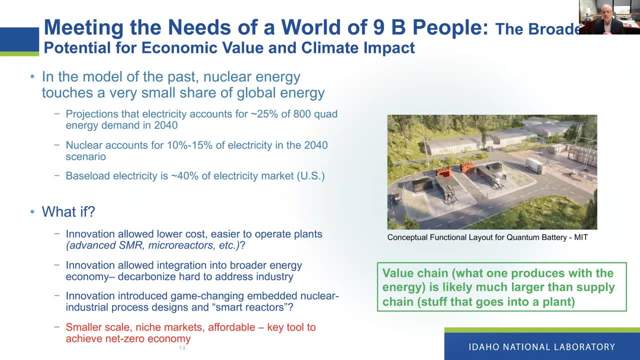 pushed toward the electric sector, for example, advanced transportation. but in today's paradigm, you know, a clean source like, like nuclear, is really only touching about. it's about 15, 16 of the us energy market. that's because, uh, nuclear in today's paradigm is only used for. 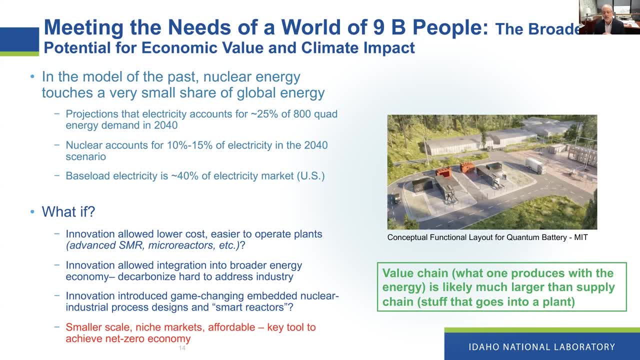 base load electrical production. but more and more that's not where uh, that's not where, not always where we we need the energy. so we think about how one can better utilize uh nuclear energy, especially through these very small and and uh smallish uh sorts of plants to 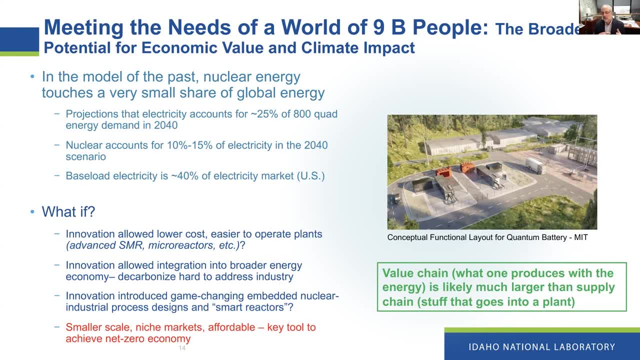 power very hard, very hard to decarbonize industry- steel production, uh cement production, chemicals productions, uh things of that nature- and also enable uh the grid to uh to function in a safe and secure fashion as we put more energy demand regionally on the on the grid with advanced transportation and such. so this is an exciting thing to think. 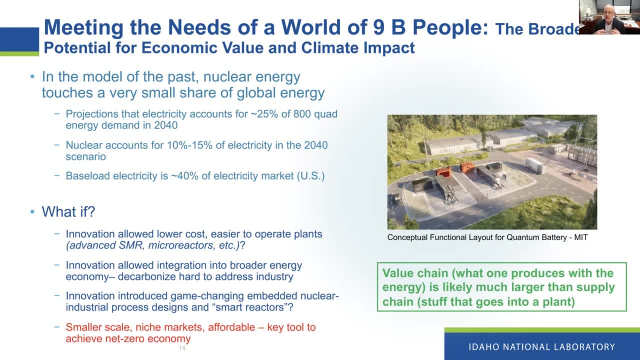 about. so you think about beyond electricity. you think about how to match. how do you create a reactor that's much more of a plug-and-play used as a clean energy module, uh with, uh with industrial processes and such. so next slide. so if you can do that, 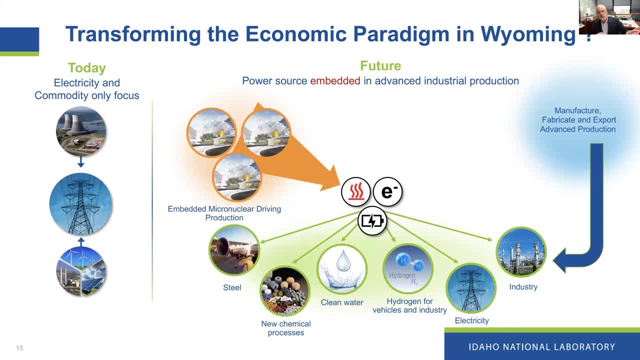 um, you go from what's shown on the left, which is, you know, nuclear, big base load, and then renewables, intermittent renewables, feeding the grid in in more of an integrated energy paradigm, then you begin to think about how you you, how can you use nuclear? is that high density energy sort? 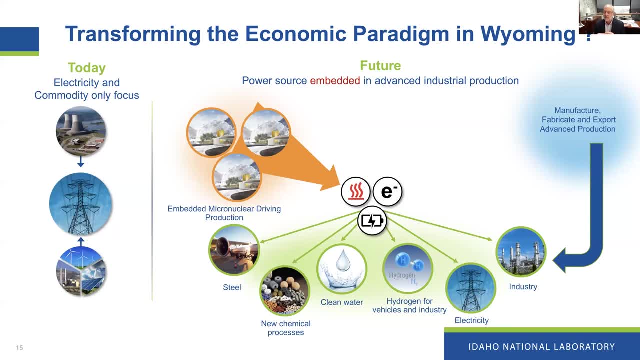 of energy in that kind of a way to uh complete your industrial process that you could imagine uh some of the same things that uh other industries like manpower uh could be doing with uh renewable and uh nuclear energy. uh a lot of it has to do with uh. 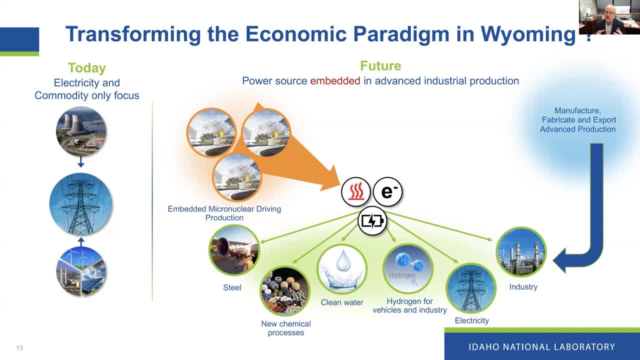 refining of the grid and so, um, and you think about, uh, you know we've cản be doing, uh, a lot of work with, uh. you know, uh, wind and solar, wind and solar, you know, and all that sort of stuff, um, and you think about how it's going to impact the future of industry, uh, and also, you know we have some. 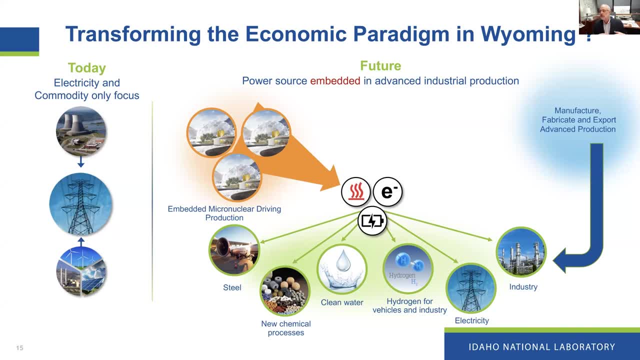 uh, uh uh. the state and the government, uh uh, as a, the state and the government are thinking about how to uh make smaller plants that are more regionally located so you don't have the risk and the demand of tying into bulk transmission grid. But if you can do that, then you think about the value. 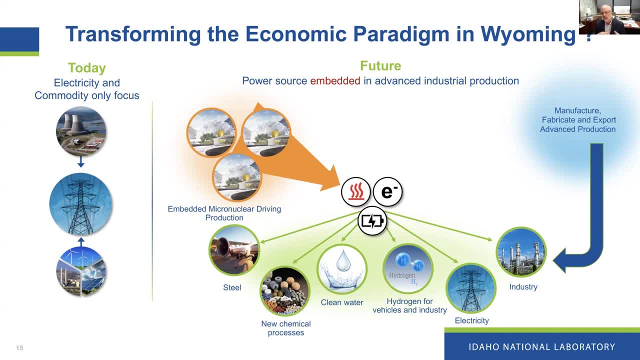 associated with engaging that nuclear market, not just from the standpoint of the reactor and the energy source but also the modular industrial processes that is powering. So you begin to think about actually manufacturing integrated products and integrated plants. And as the world begins, as actually export policy and global trade policy begins to 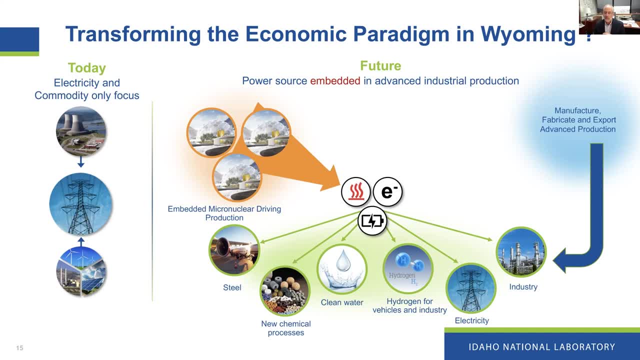 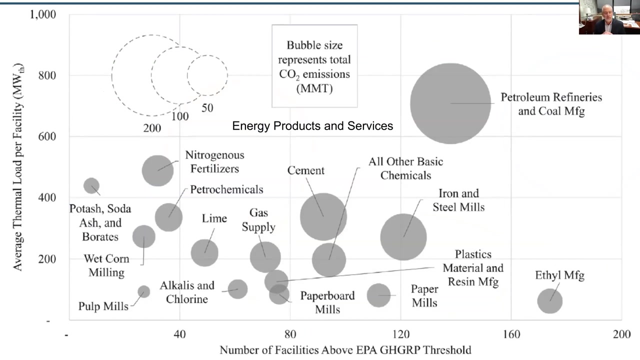 change because of net zero goals. being able to export that sort of thing- modular industrial processes are powered by clean energy modules- becomes very important, And I think that's a very, very intriguing and intriguing to quite a few people. So next slide, And I just wanted to give you just a quick picture of this. I always found this an 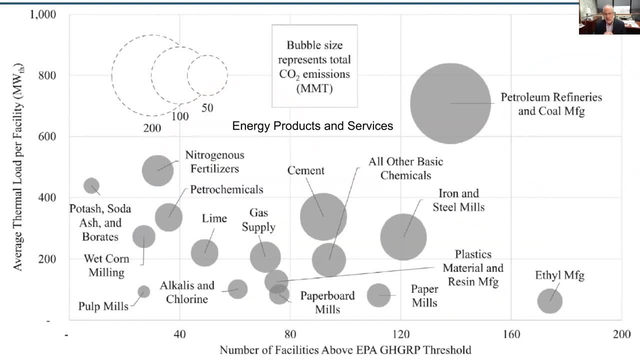 interesting chart This shows. on the horizontal it shows the number of facilities that are in the country that exceed a greenhouse gas reporting threshold And then on the vertical axis it shows the average thermal load. So in Wyoming you can see all the way on the left not all that many of these carbonate businesses out there. 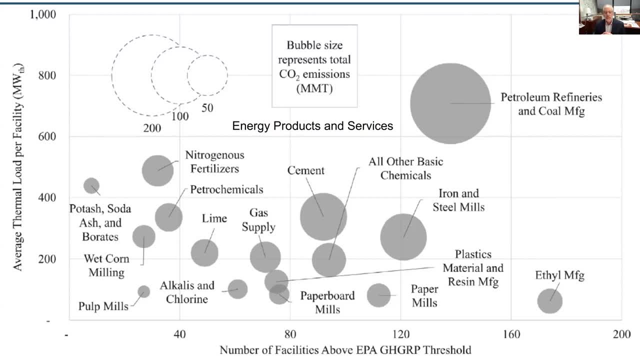 but the ones that are there are energy, very high energy consumption, Fertilizer manufacturing, the same of course with the petroleum refinery, a large heat load associated with those and also a large number of facilities. But that gives you an idea of the landscape, of the number of industries where one could. 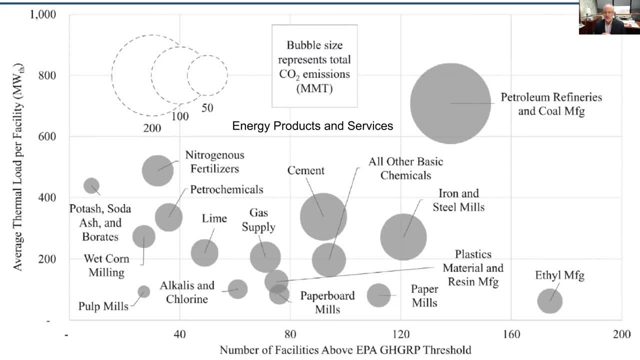 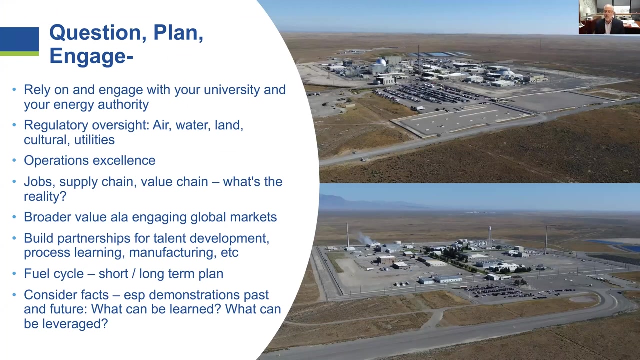 begin to integrate nuclear as a clean energy source to power those industries. And those are generally more difficult to get to a net zero basis because they just require just a lot of energy. Next slide. So that's kind of what I wanted to leave you with. 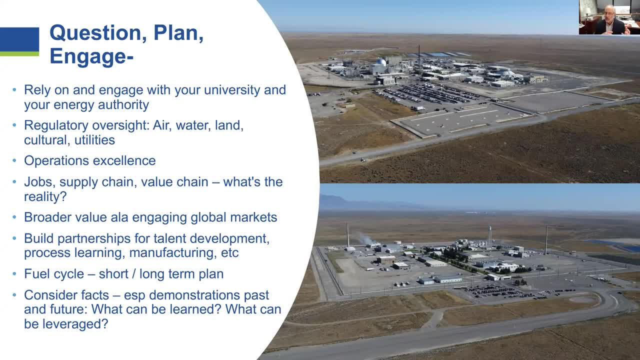 David Morgan As a perspective on why nuclear going forward is a little different. It is a natural evolution of what we've seen in the past. There's a lot that's been done in terms of testing and validation. There's a lot that's been done in terms of testing and validation. 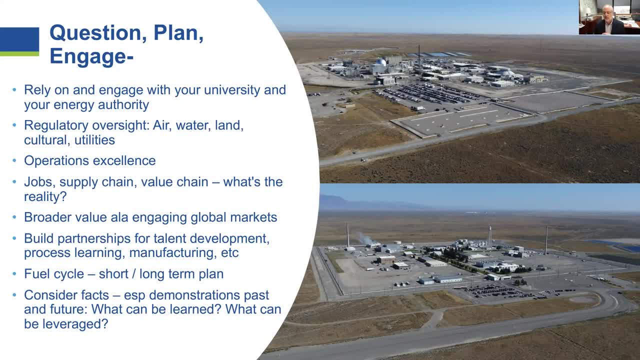 validation of those classes of reactors, especially the sodium cool fast reactor. I want to draw your attention to that EBR2 experience. Actually, these two pictures that are on this slide are two of the reactor testing areas at the National Lab. The one on top is the old EBR2. 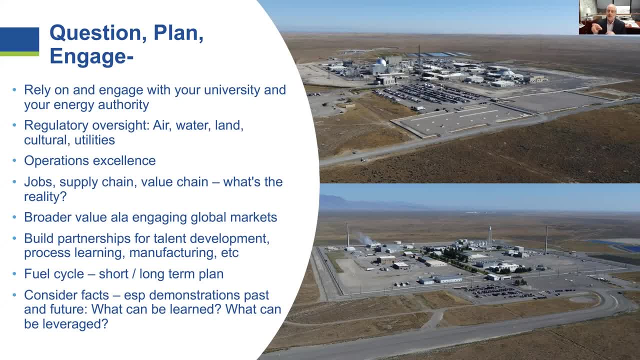 site You can still see the old dome. So that's the site I grew up working at, And then the bottom one is the advanced test reactor that's operating today and very successfully and safely. So questions I think is useful for any stakeholder to consider and think about. 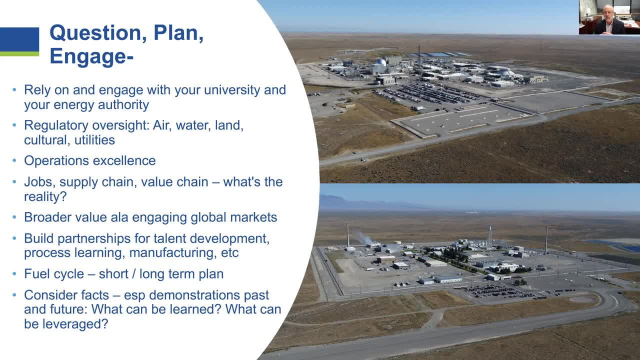 Like I said, definitely rely on and engage your, your, your university, your community colleges, your energy authority and the labs happy to engage and answer questions as we can as well. Regulatory oversight: that's something you'll get involved with. although NRC is the Nuclear, Regulatory Commission is the. 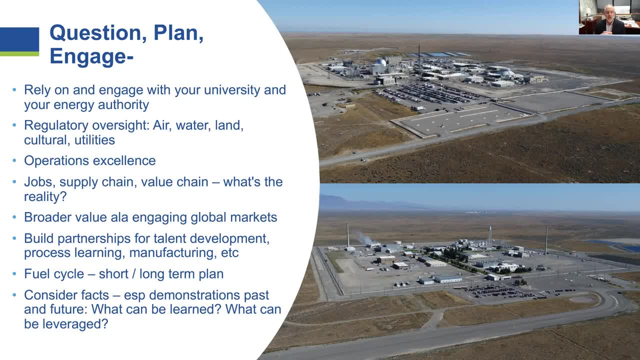 regulatory authority for nuclear materials and reactor operations. The state is going to have some footprint in air, water, land, cultural and even utility operations. I would always encourage people to encourage your leadership to focus on operational excellence. Many of the challenges that have been experienced globally, we've seen them as well And I think the 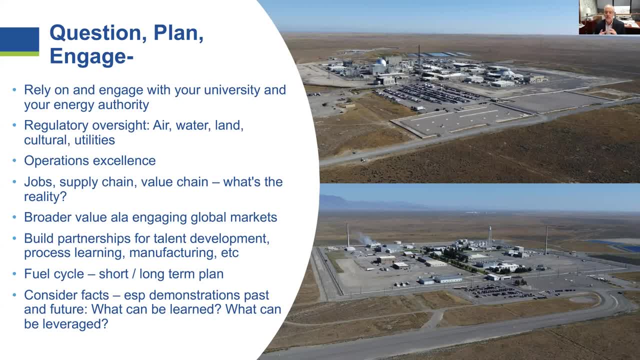 experience globally with nuclear industries and a number of other industries are rooted in operations, not the fundamental technology Jobs. We get a lot of questions about how many jobs are associated with a commercial nuclear plant. One can think about the number of jobs directly tied to the plant. A lot of people talk about supply chain for nuclear 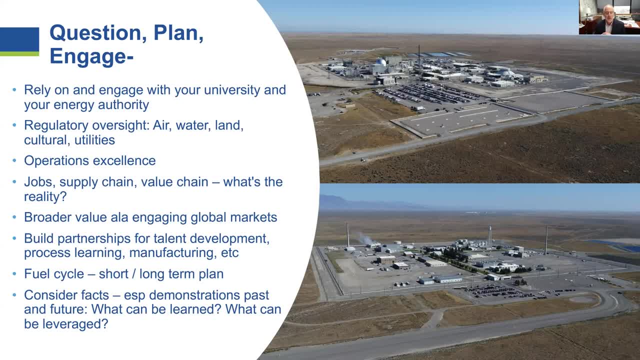 It's all the stuff that goes into the reactor and operations. I'd encourage you to think about the value chain of having a clean energy source Instead of just putting electrons on the grid. what can you manufacture with it? That's a force multiplier for economic. 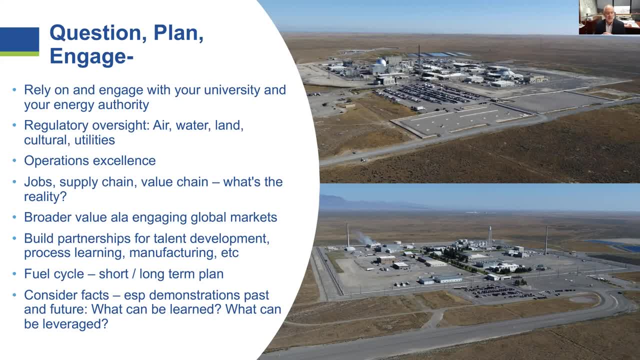 value. That's really the exciting piece. That ties to: how do you then engage global markets with a clean energy driven process? Yeah, Yeah, Yeah, Yeah. I think it's important to think about the value chain of a product, whether it's chemicals. 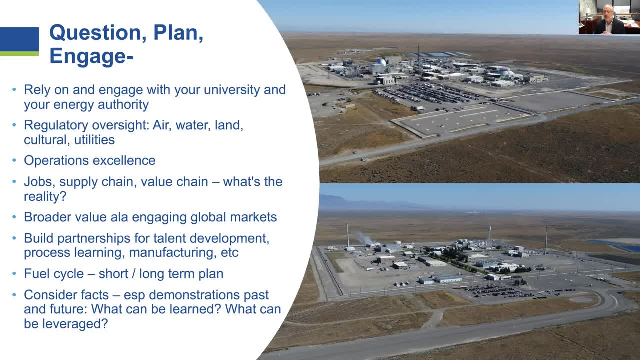 or plastics or cement or steel or whatnot. Partnerships, I think, are important. They're important to tap into that value chain, Both the value chain and the supply chain. quite frankly, Josh is going to talk about fuel cycle. Those are really important things to 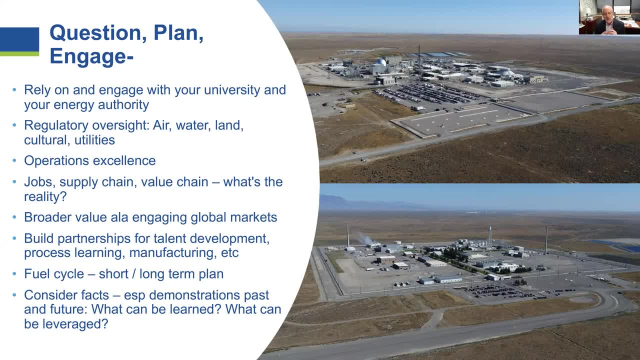 And then I'll leave really where I started and that's, you know, lean on that 65,, 70 years worth of knowledge, lessons learned and others to inform your questioning and getting answers to your questions. And so I'll leave it there and look forward to your questions after my colleagues are finished. 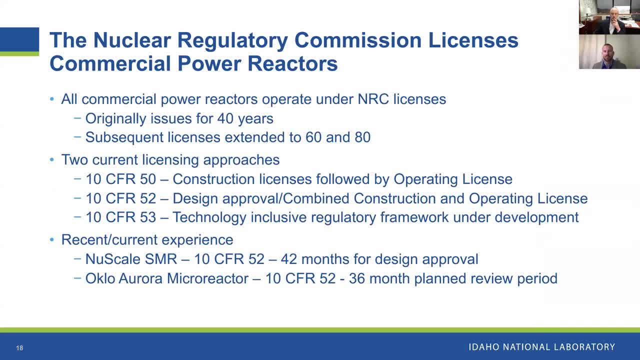 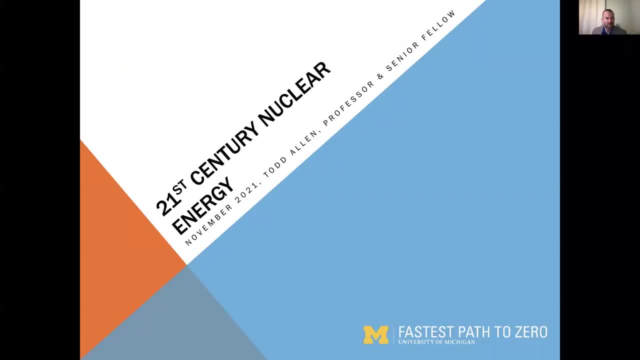 Yeah, thanks, Steve. Yeah, everybody, that is how it's going to work. We're going to go through the presentations first and then go to Q&A. If you want to submit a question, there is a Q&A function at the bottom of your screen. You should go ahead right ahead and type those in. 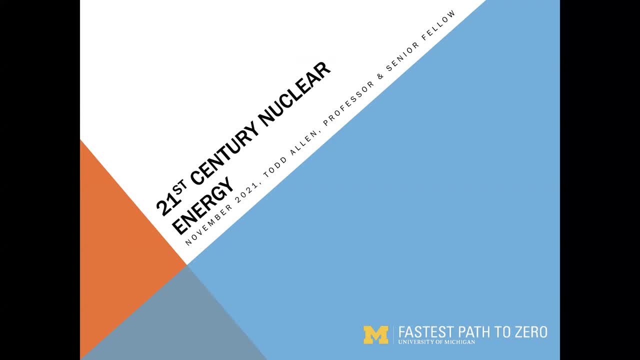 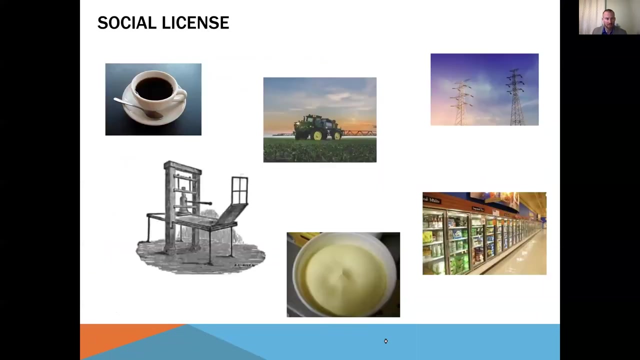 I will try and moderate my way through those, maybe even answer a few on the fly. So the next presentation is by Dr Josh Jarrell from Idaho National Labs at Christine. I think this is the wrong presentation that's showing now. I think we're supposed to go to Josh next, but yeah, it looks like we've got that out of order. 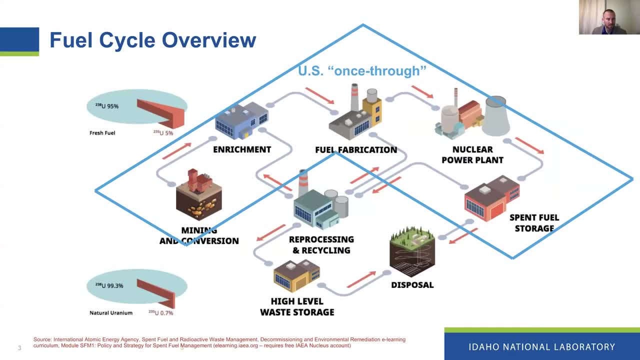 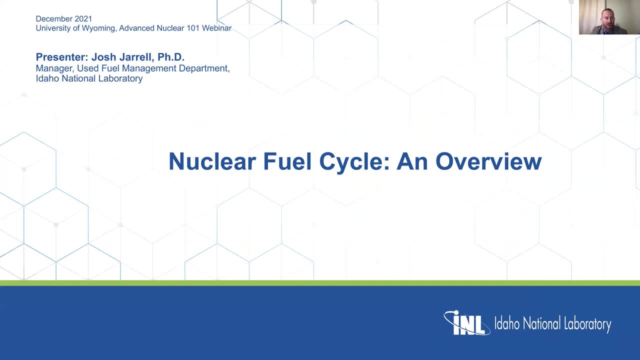 But yeah, Josh, as we sort that one out over to you, Thank you, Thanks, Glenn, And, as Steve mentioned, let me kind of give a quick background on me, who I am. So I'm a nuclear engineer. I grew up in Texas, actually. 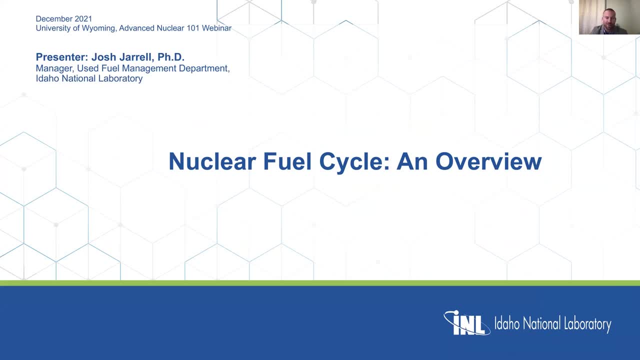 I went to school down in Texas- A&M, I would argue it's also a very good nuclear engineering program. I got my PhD down there. I came out of school and then went and worked at Oak Ridge National Lab, which is on the east side of Tennessee. 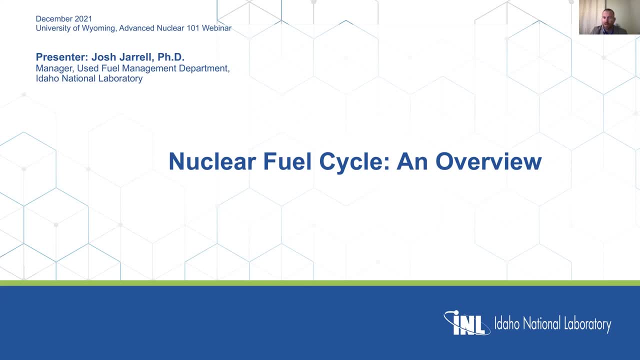 And then, about almost five years ago, I came out to Idaho National Lab and I currently manage a used fuel department here, And so my group and my staff. they focus really on spent nuclear fuel, And spent nuclear fuel is just one piece of the broader nuclear fuel cycle. 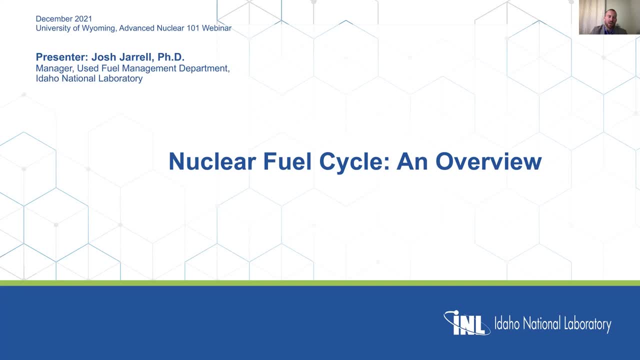 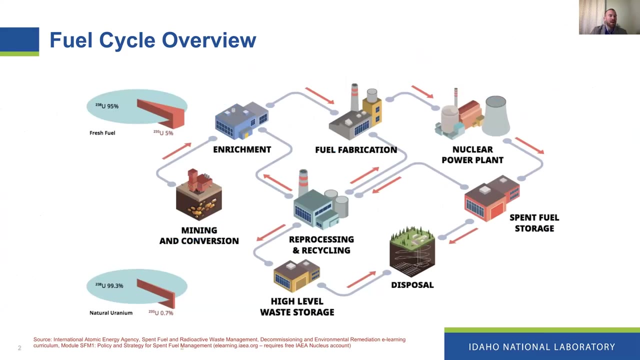 And that's what I'll be touching on today. So let's just go to the next slide. Christine, I'm not seeing the next slide. Oh, there we go. So you know, for any of these reactors, obviously you have to have nuclear fuel to operate. 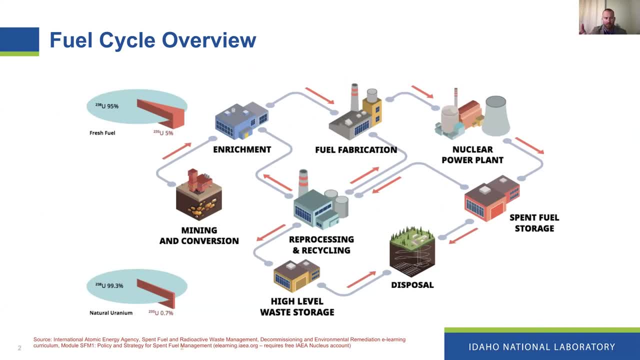 These reactors, And so when we talk about some of the fuel cycle, the supply chain, I think it's important for everybody to kind of understand what that entails. And so uranium is the key for nuclear reactors, at least for the vast majority of the currently operated ones. 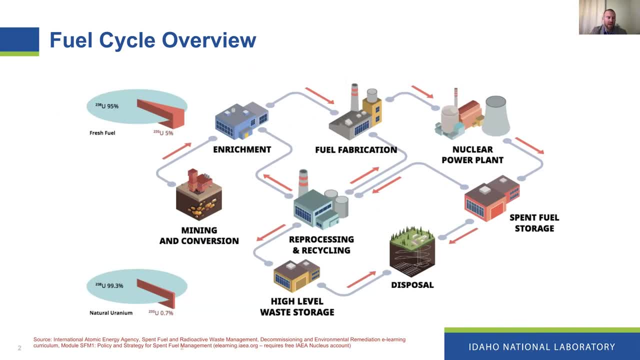 And so we pull uranium out of the ground, We mine it. When uranium comes out, it's natural uranium, And there's a specific isotope- uranium-235, that you can use That you really need for reactors to operate effectively. 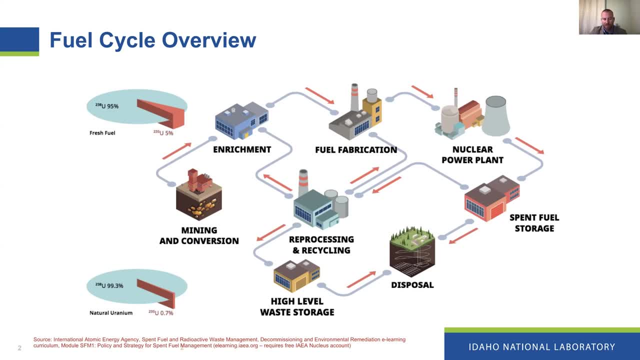 And so the amount of uranium-235 in uranium is a little bit less than 1% in natural uranium, And what you need, at least in the current operating reactors, the large you know thousand megawatt sort of reactors, light water reactors that Steve mentioned- is you need fuel that's about 5% enriched with this uranium-235.. 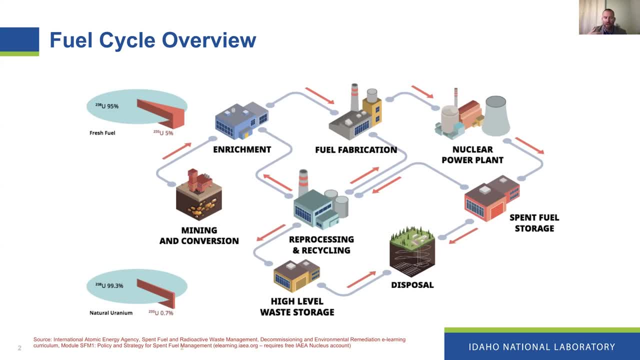 And so once you mine it, you have to Then enrich it up to about 5%. You can then fabricate the fuel, And I'll get into these details. Then, once you have fuel that's in the right form, you can put it into a nuclear plant and operate that plant. 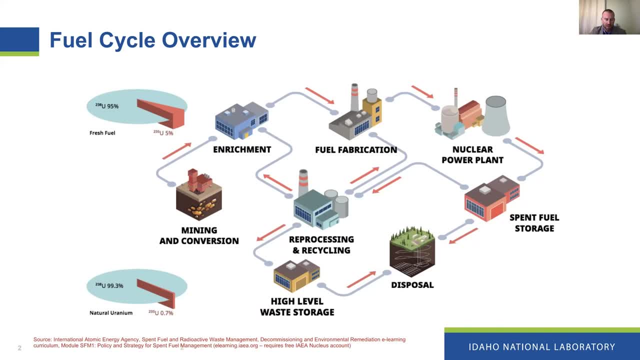 After maybe several years, the fuel is no longer useful in that current plant, And then the fuel comes out and it's spent fuel, And so you have to manage the spent fuel, And the goal- The goal is to The goal for spent fuel, at least in the US- is to eventually dispose of it in a deep geologic repository. 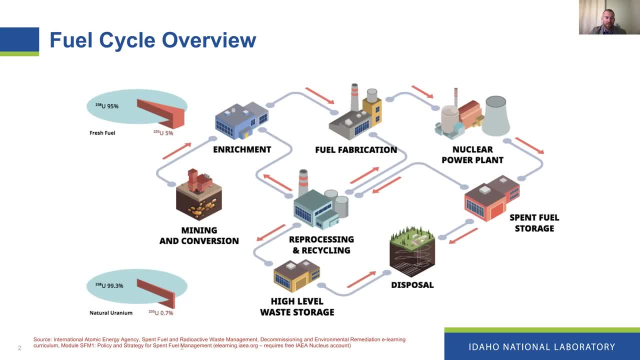 There's also the option of recycling or reprocessing the fuel. However, the US doesn't generally use this process. Instead, it goes: Christine, will you hit the next slide? We do what we call the once-through cycle, So we do not reprocess or recover the uranium. 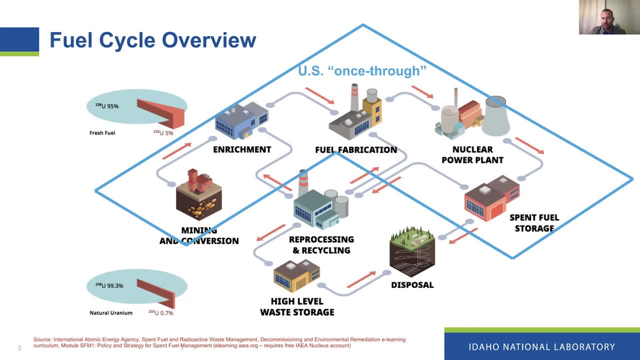 We just basically at this point, because we do not have an operating disposal repository, we basically are storing the material right now at the current reactor sites, And so this is kind of in the broad scheme of things, what the fuel cycle looks like. 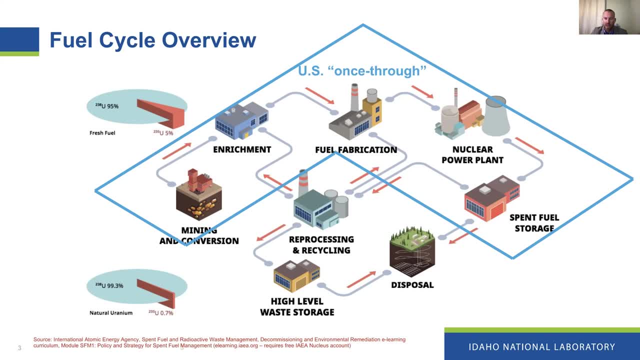 Really, you know, we generally operate these light water reactors. this current fleet that we have, The advanced reactors that we're talking about, we're not going to be using them. We're going to be using them for a lot of other things that we're talking about- may have other opportunities to potentially recycle in the future. 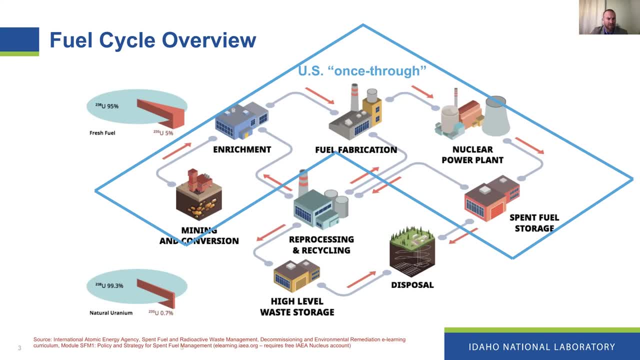 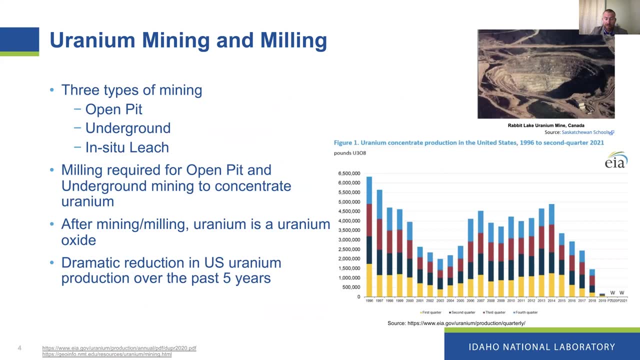 But right now this is where we're at, So if you go to the next slide, we'll start with the mining and milling. Wyoming has an extensive history of actually uranium mining. There are three different types of mining and in two of those types of mining milling is required to concentrate the uranium. 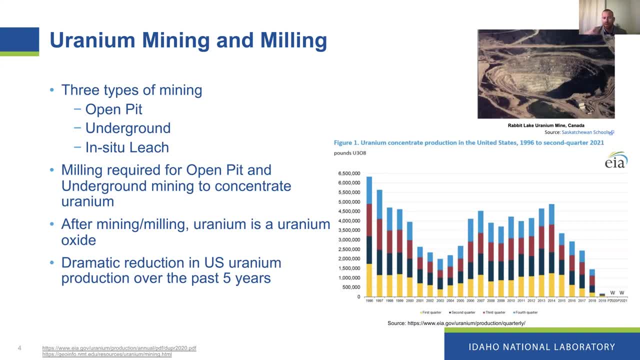 And when you pull it out of the ground and you basically have what we call a uranium oxide. So that's important to note because the form of the uranium does matter for several of the steps in the fuel cycle. One thing: if you look on that far right image that shows the uranium production in the US by year and the far left, I think, is 1996,. 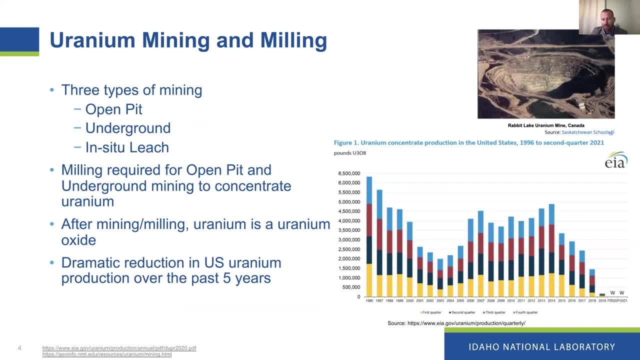 you'll see that the production over the last four or five years is down dramatically. You'll see that the production over the last four or five years is down dramatically to essentially almost zero, And so there's reasons for that. but it's something to just keep in mind, that Wyoming 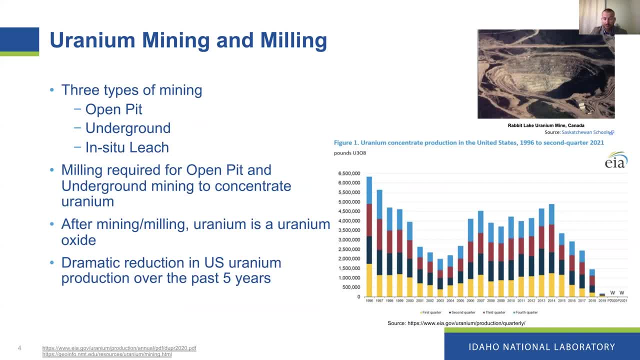 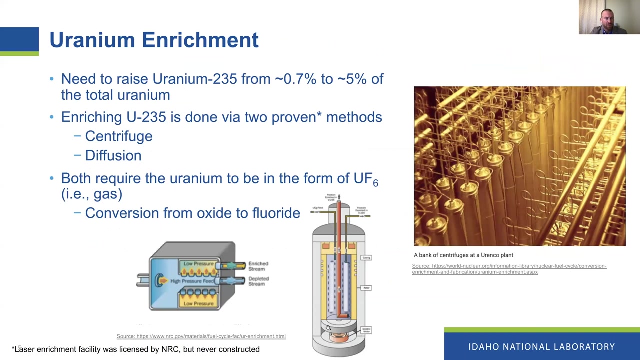 which is one of the largest uranium producing state, was the largest uranium mining producing states- has basically wrapped up or greatly reduced the amount of uranium that it's mining at this point. All right, so next slide. Maybe I'm seeing multiple slides. 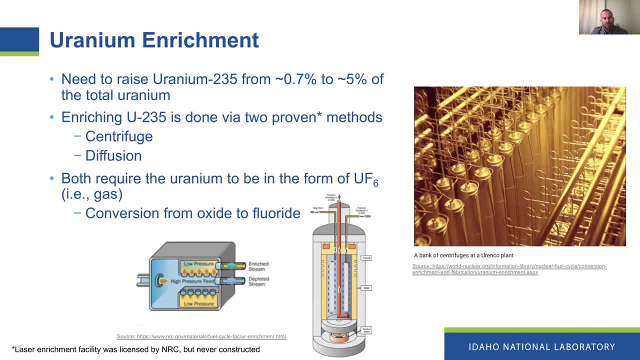 There we go. Okay, so enrichment. One of the things, as I mentioned before, is uranium. Naturally, uranium has less than 1% of uranium-235, so you need to enrich that uranium-235 up to about 5%. 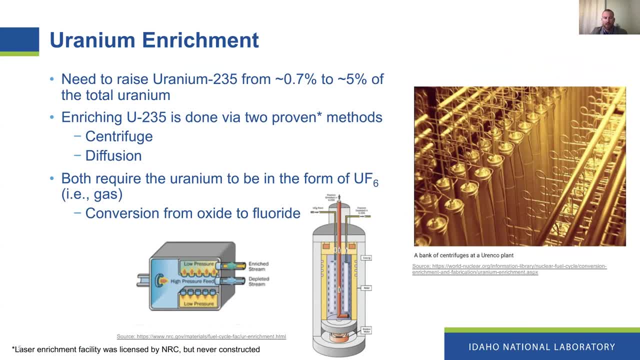 And there's a couple different ways, two sort of proven methods to enrich uranium. One is centrifuges, which are small, basically cylinders that spin the uranium and can separate, basically use the physics that some of the isotopes are heavier than the others. 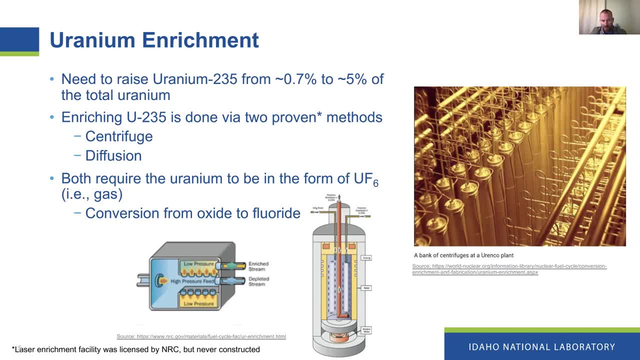 and enrich that. So you can do that in that fashion. That image right. there is a bank of centrifuges. There's also a diffusion method that you can basically use: diffusion and again the size of the isotopes to enrich, But for both enrichment methodologies. 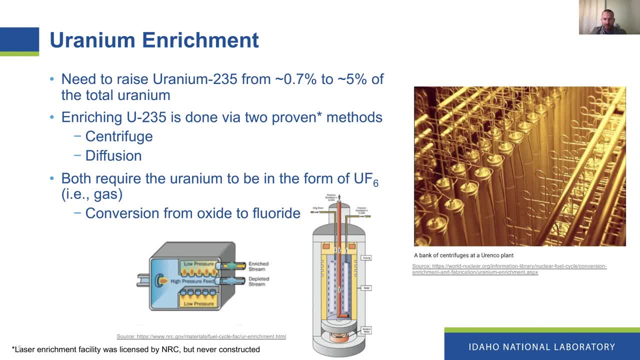 you have to convert that uranium oxide that I talked about- That's basically when you come out of the ground- to a gas, to a fluoride. they call it UF6, or uranium hexane of fluoride and um. so when you hear the term conversion or deconversion, you're basically 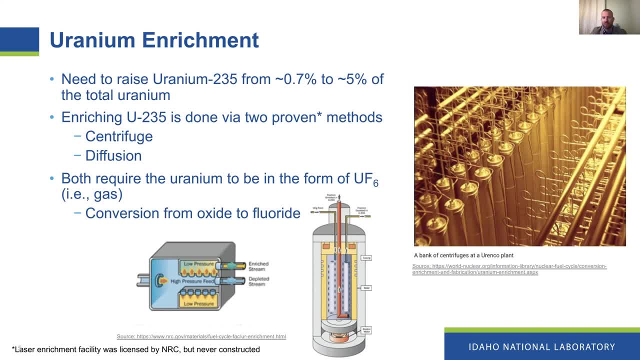 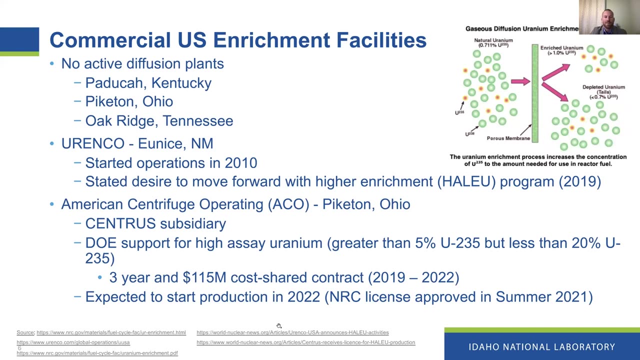 changing the form of the uranium from an oxide to a, a gas or a fluoride. so if you go to the next slide, all right. so, um, this is just kind of given the state of play of the enrichment facilities. diffusion, uh was was very popular um 30, 40, 50 years ago. uh, really to support um the nuclear. 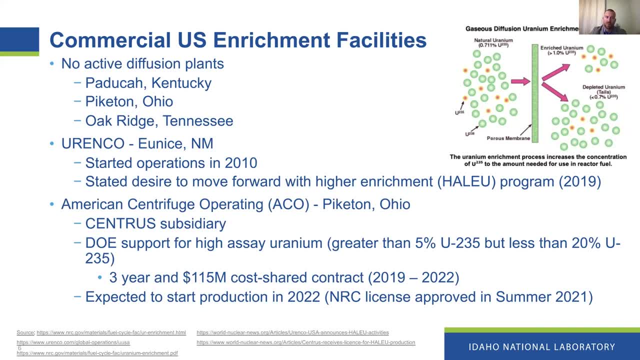 industry but also nuclear weapons. um, and there were, there was several diffusion plants: kentucky, ohio and tennessee. none of them are actively producing enriched uranium through diffusion anymore. these tend to be very large facilities, very in energy intensive facilities, and so that's one of the reasons that the diffusion plants have kind of have gone away to the centrifuge. 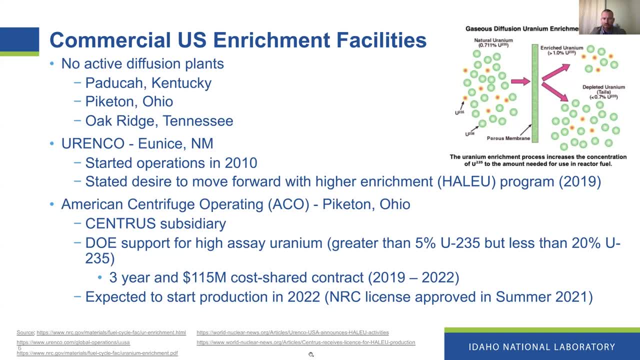 uh concept. so there is an active uh enrichment capability in new mexico. your rinko is the name uh- of the uh facility. they've been operating for a little over 10 years. um, and one thing that's interesting- and i i haven't mentioned it yet, so i'll do that now- is 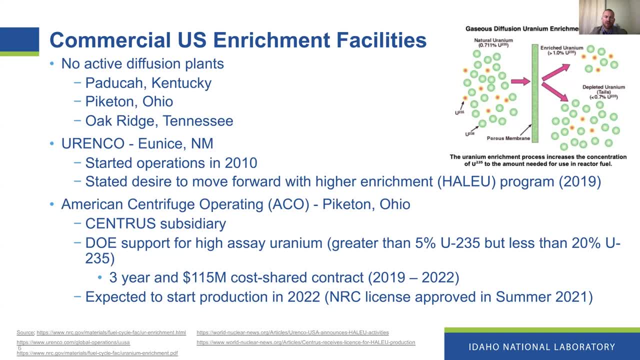 um, the normal light water reactors that we have uh need about five percent enriched. however, a lot of the other light water reactors that we have uh need about five percent enriched. however, a lot of the advanced reactors are looking at up to maybe 20 percent- 19 to 20 percent enriched uh uranium. 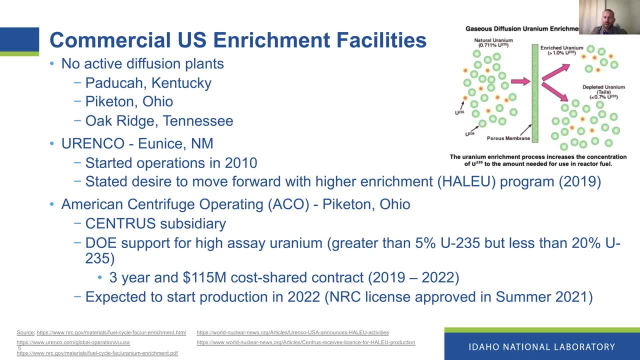 and so one of the questions is where and what facilities are available to do that next sort of phase of enrichment. so, um, uranko has actually stated they'd be interested in producing this higher enriched uh uranium. they actually call it halo, which is high assay, low enriched uranium. 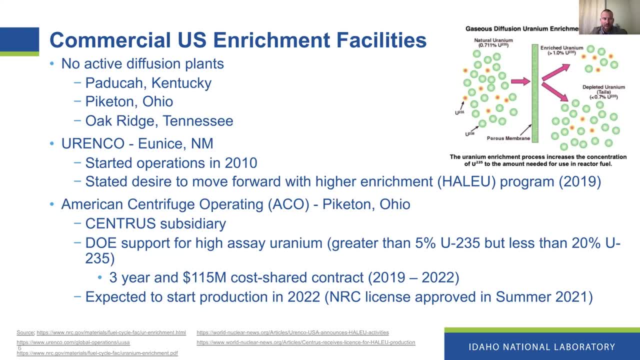 so that's that 19 to 20 percent uh material, though they have not moved forward. however, um, there there has been a facility that's kind of came up and is now running in piketon ohio, which was the facility that was originally a diffusion plant. they've now 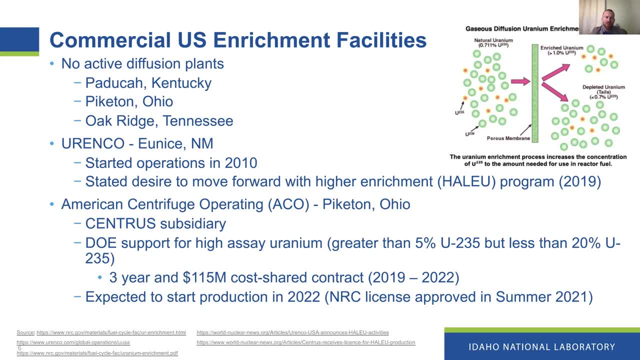 used or now set up some centrifuges to actually develop and produce high assay, low enriched uranium and that has actually been a cost share. so the department of energy has has provided funds over the last three years um to basically set up that enrichment facility. uh, they did receive their their operations license. 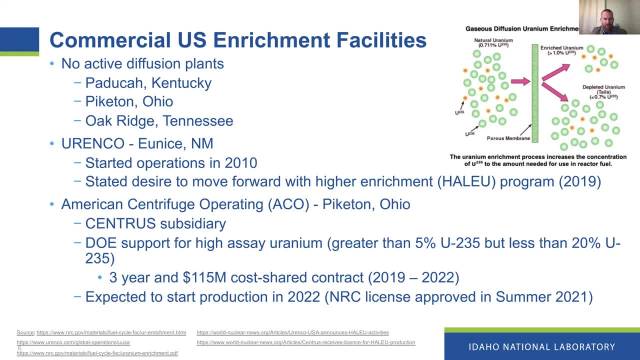 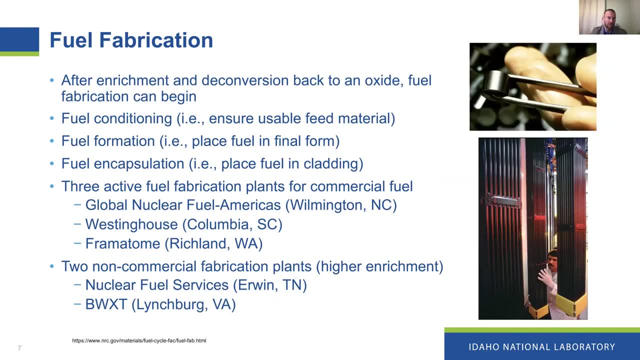 from the nrc, which is the, the regulator of the nuclear regulatory commission. um, and they hope to start uh production in 2022.. all right, so how about next slide? okay, perfect, so. so, once the uranium is enriched, uh, you can actually fabricate the material and? um, as i noted before, the 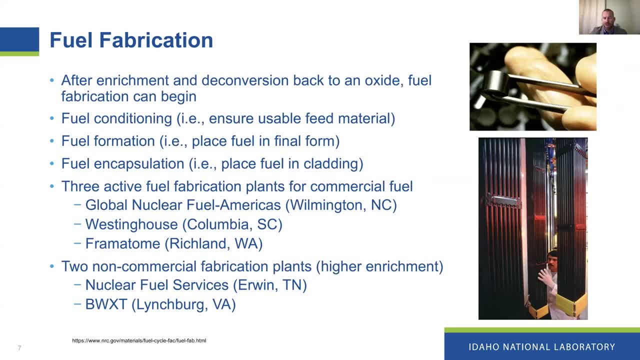 enrichment again is in this gaseous phase you actually move it back to an oxide, because in light water reactors, uh, we use a uranium oxide based fuel, and so then you actually get create these small pellets, which is that top right uh figure is actually a uranium oxide pellet. 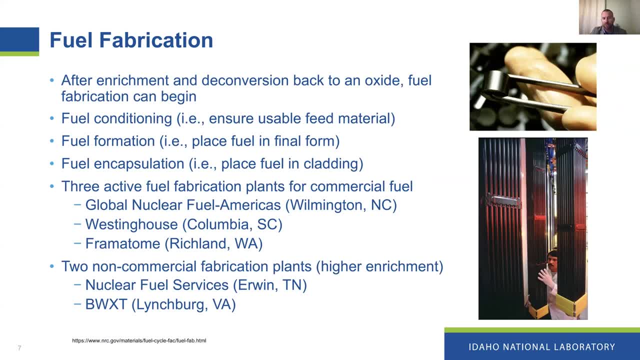 um, you'll form it and then you'll actually what they call encapsulate it. you'll put it inside of some other cladding material. generally for light water reactors we use a zirconium clad, but for some of these advanced reactors you'll have different fuel forms and you'll have different cladding materials. 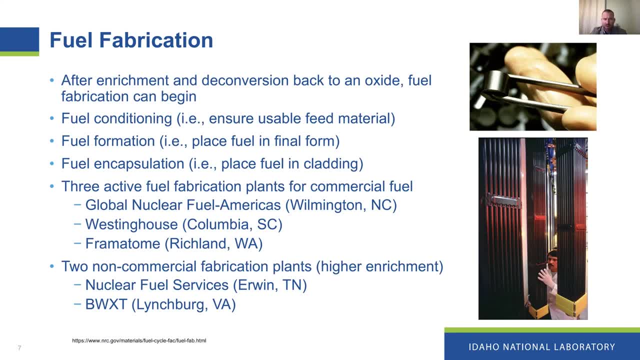 now there are several active fabrication plants again. we we do have almost 100 light water reactors operating, and so they need continual fuel each year, and so there are three big plants: one in north carolina, one in south carolina and one in the state of washington. that 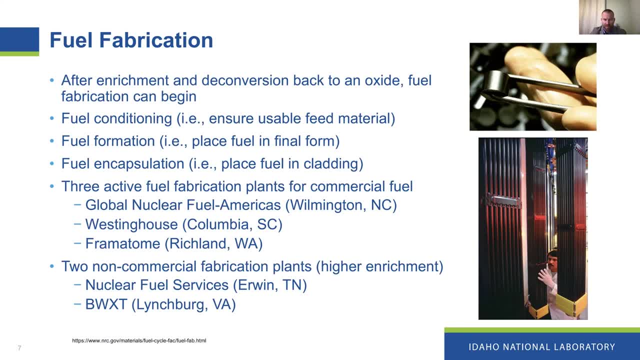 are that generate commercial fuel. so that image on the bottom right is actually a light water reactor fuel bundle. and then there's also two non-commercial fabrication plants in one in tennessee and one in virginia. they can go to much. they can handle, uh fabrication of fuel to much higher. 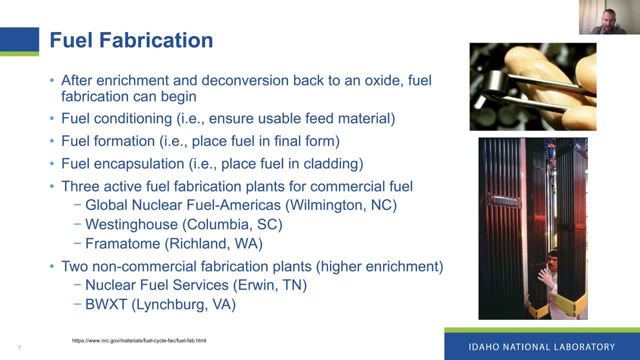 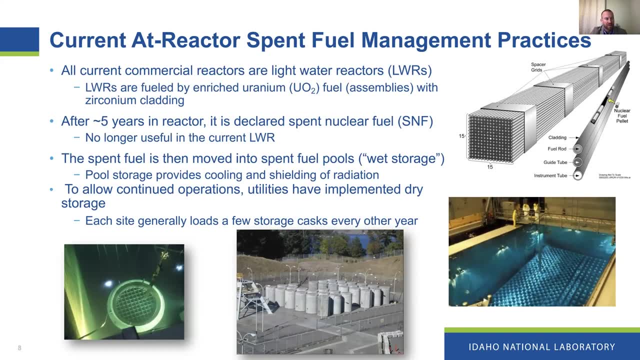 enrichments, um, for example, the naval reactors. uh, they would generate the fuel for the, for the, the subs and carriers. all right, if you go to the next slide, all right. so that's how what we call the front end of the nuclear fuel cycle generally works, um, and then again you put the re, the fuel into. 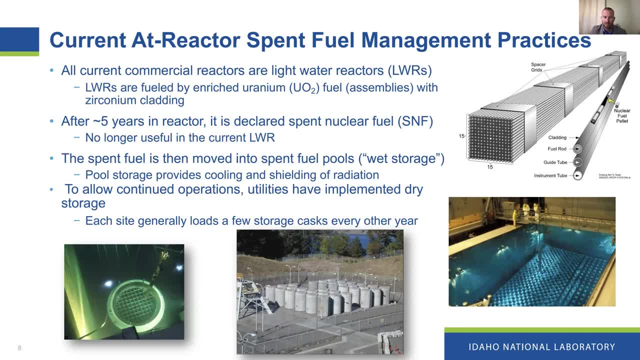 the reactor and then afterwards it's spent fuel, and so this is actually the bulk of the work that i do on a day-to-day basis is looking at what we do with the spent fuel. um, so, as i mentioned uh, light water reactors use this uranium oxide with zirconium cladding. uh, the picture on the 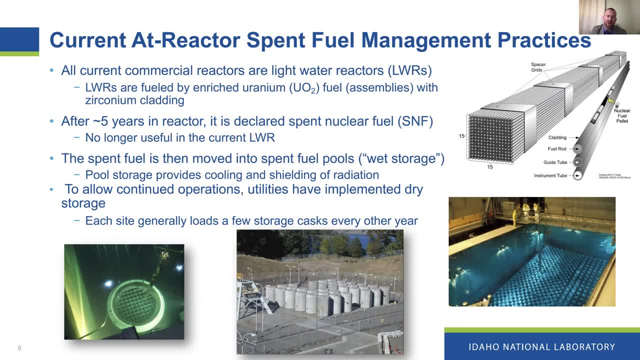 top right is an example assembly. and so after about five years in the reactor- and it kind of depends a little bit on the operations and the design of the reactor- the fuel is no longer usable. it's still very radioactive. so the main reason is the fuel is not super radioactive, it's not. 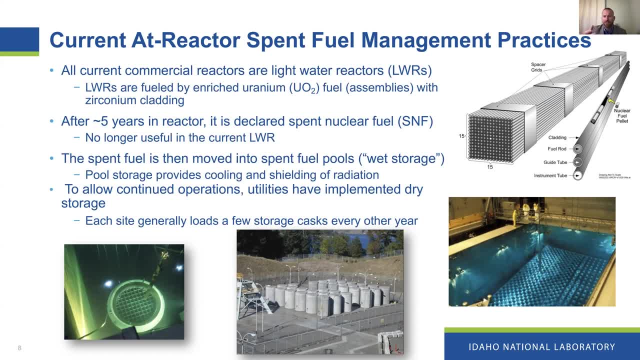 super radioactive. it's not super radioactive. it's not super radioactive. when the fuel comes out, uh, it's very radioactive, um, before it goes in. if it's just uranium, um, it's actually uranium itself is not, uh, super radioactive. it's not that dangerous. in fact, you saw people actually you. 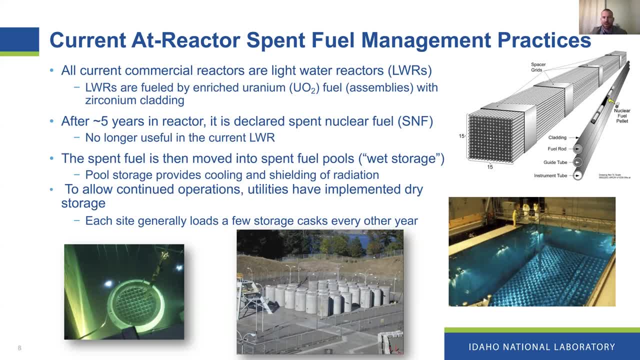 know sort of handling pellets and and and the assemblies before they go into the reactor with gloves. so it's a relatively benign material in the spent fuel And as such it's not something that you know somebody could go up and touch, And so it needs to be shielded and cooled because it still has residual heat coming off of. 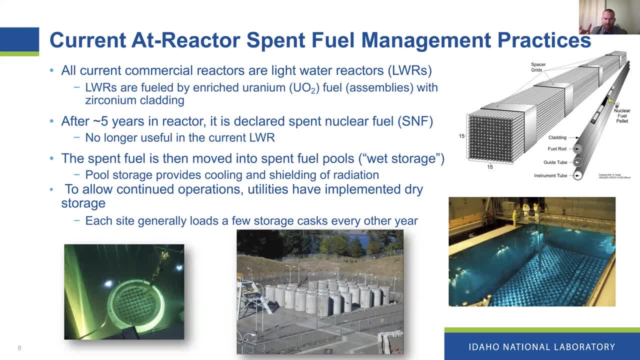 it for a few years, And so all of that spent fuel in the light water reactors actually goes into the pools, And these are very deep pools. Picture on that bottom right just shows an example pool where the fuel generally will sit for at least three to five years All reactors have spent. 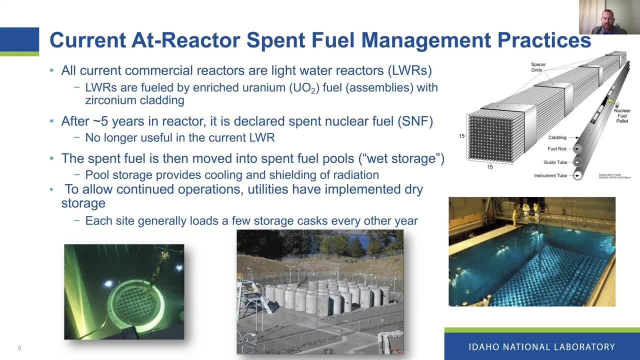 fuel pools at them, And they were designed- the pools themselves were designed to support those reactors. However, these reactors are operating for 40,, 60,, maybe 80 years, And so those pools are actually starting to fill up And, because of that, the utilities are moving to dry. 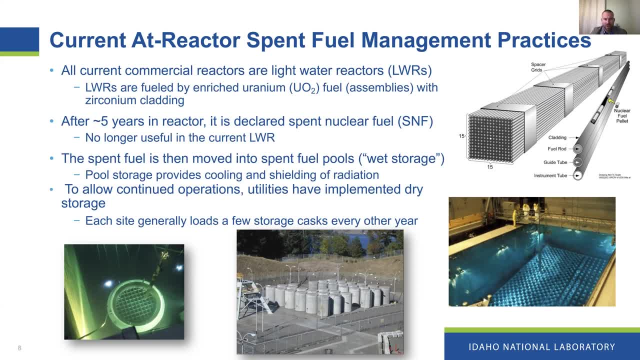 storage, And so the picture in the middle is actually a very large dry storage systems. Those are big concrete cylinders, And inside the cylinders there's generally a welded steel canister, And inside that canister there's spent fuel. And so now at the reactor sites. 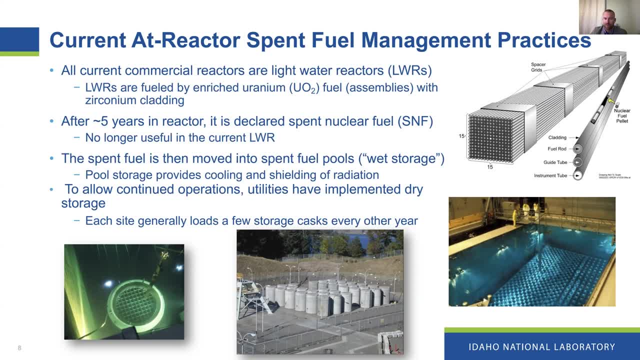 they'll load a few of these dry storage systems about every other year to make sure that they have plenty of room in their pool to discharge The spent fuel assemblies that are coming out. So you go to the next slide. you'll see some more. 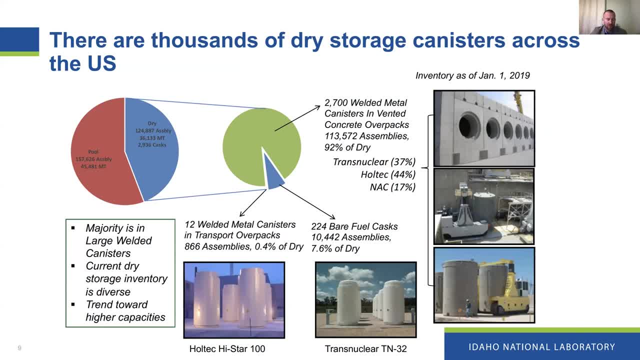 details about those dry storage systems. We have dry storage system at Idaho National Lab actually, But across the US there's- well, let's see here, I think there's over 3,000 systems now- My numbers are a couple of years dated here- And these systems again are very large, Diameter of. 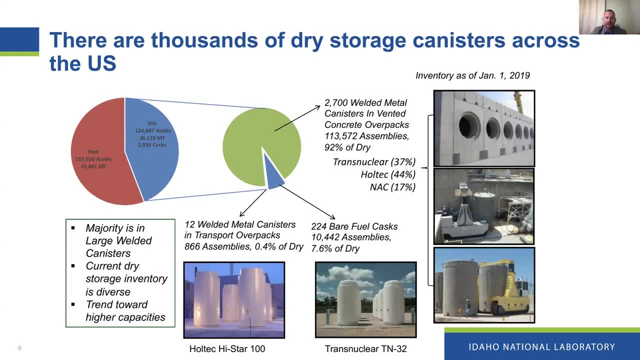 some of these cylinders can be six, eight feet And, you know, 20 feet plus tall, huge, 100 ton sort of concrete and reinforced steel, sort of structures that protect the spent fuel, shield it from the environment and provide shielding to those. 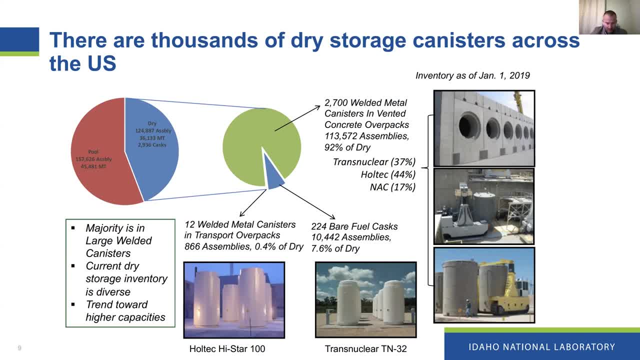 outside So you can see, in the bottom right maybe, how big those systems are- And there's actually a person there for context. So very large, very robust structures. Generally, for the most part, they're concrete and steel, but they actually have an internal canister in them. It's a stainless steel. 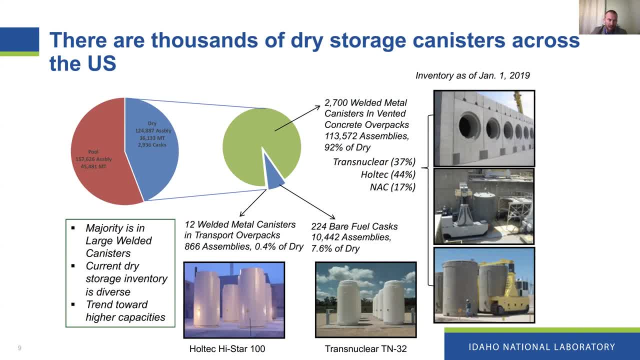 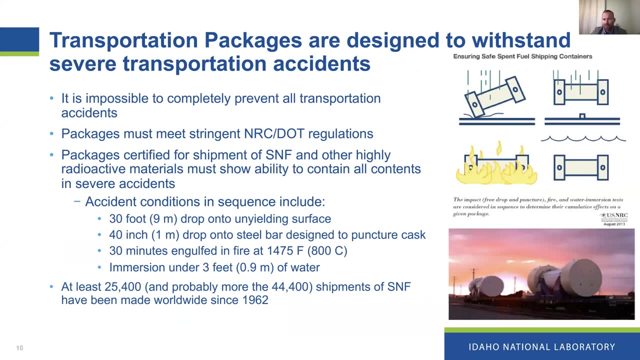 welded canister where the spent fuel goes in, And the idea for that canister is that you can then transport that material in the future away from the current sites, And so if you go to the next slide, you'll see some examples of the transportation approach. And so, basically, 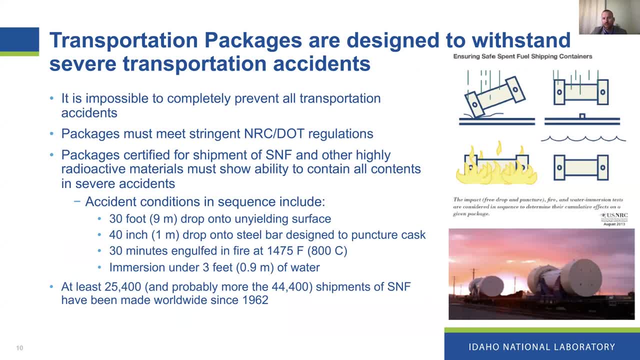 you'll pull that canister out of storage and place it into a different transportation configuration. The bottom right is actually images of transportation casks on a rail car actually- And these, these casks are incredibly robust- again, huge, 100 plus. 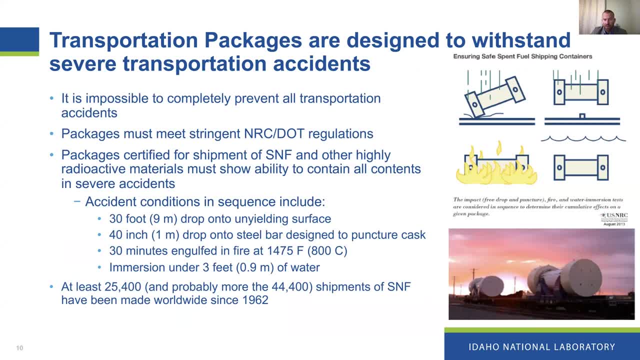 ton structures And the regulator, the Nuclear Regulatory Commission, really certifies and make sure that they will withstand several different accidents and areas- And so they actually are- are have to be tested to survive several different accidents: fires, submersions, drops And- and the last thing here I'll note- on the transportation pieces we have been 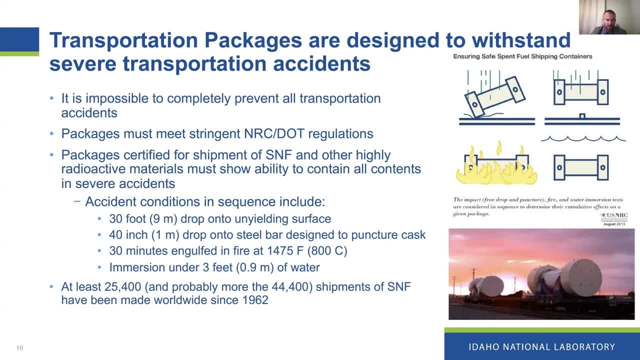 transporting spent fuel around this country as well as worldwide for several decades without sort of any significant incidents. There's some we know of at least 25,000 shipments and there's probably close to double that. that have probably happened in some of the other countries. that that we don't have maybe there's good records with, but have been made over the last, you know, 50 to 60 years without 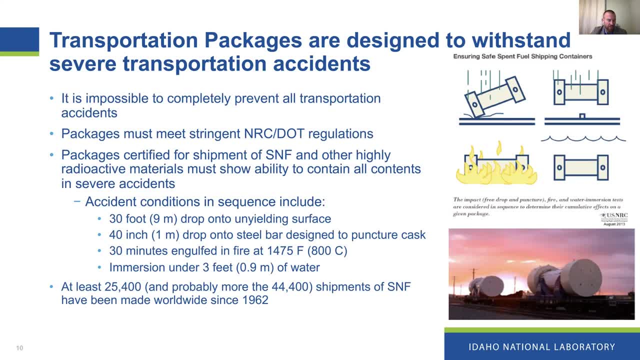 incidents of release of radioactivity, damage to the public, that sort of thing. So very safe, very robust system for transporting this material. So the goal, though, of course, is to be able to transport it somewhere off of the sites. Again, I mentioned that. 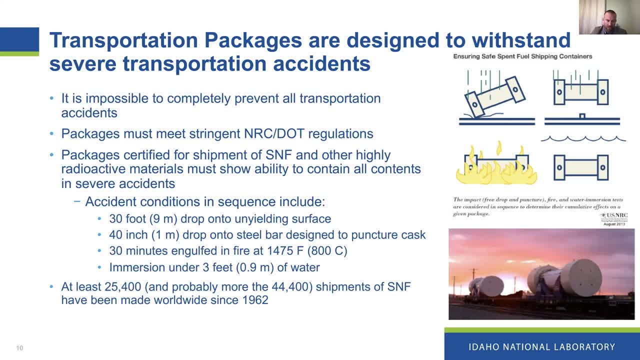 disposal, which is generally deep underground repositories are the plan, But in the US we we don't have an active repository program being worked. We do have a site, but but that program is not being pursued right now by the federal government And as such, we're looking for interim solutions to manage this material. So if you go to the next slide, 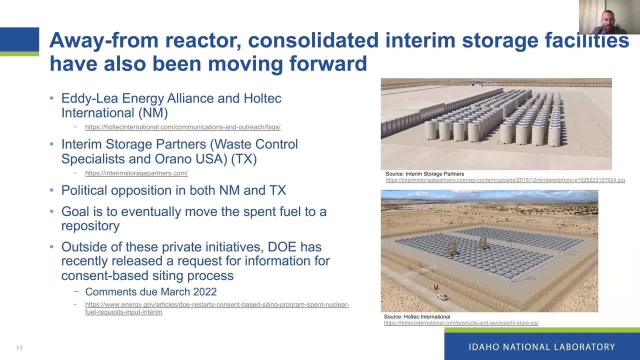 So we're looking at opportunities to site interim facilities that their whole intent is to store this material for the next few decades. Currently, as I mentioned, we have these, you know, 100 or so- a little less than 100 now, unfortunately- operating nuclear reactors and each of them is storing their fuel on their site And the idea is to consolidate that at some location in the future. 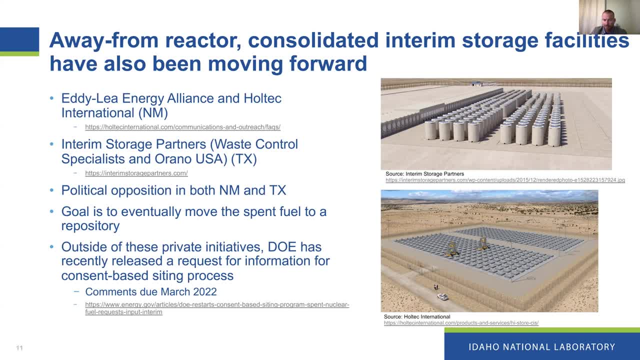 And a wider range of stedes or other types of tanks are available, And we've set up sufficient sabe and some Tit ders about that and to still have a wide scope on those devices. Again, the canisters are designed to be transportable, And so the idea is we would transport them somewhere else. There have been a couple. 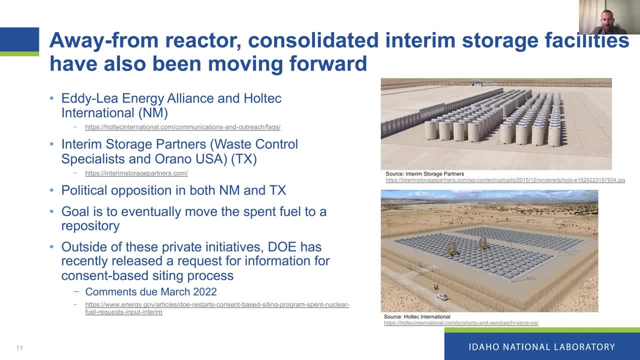 private initiatives, one in New Mexico and one in Texas. actually they're both right across the New Mexico- Texas border, so from each other And those are moving forward. just received uh nrc approval um the. the one in new mexico is still under under review by the nrc. 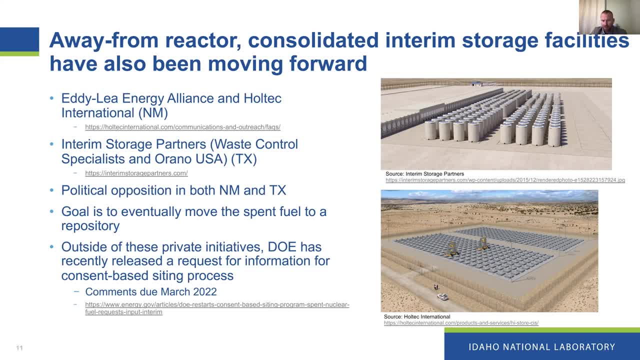 but those approvals are really on the, on the technical grounds, which is, is it safe, is it going to protect the public? um, there have been, there has been political opposition in both of those states, so i think that's important to note. um, and regardless, the goal again is to move to. 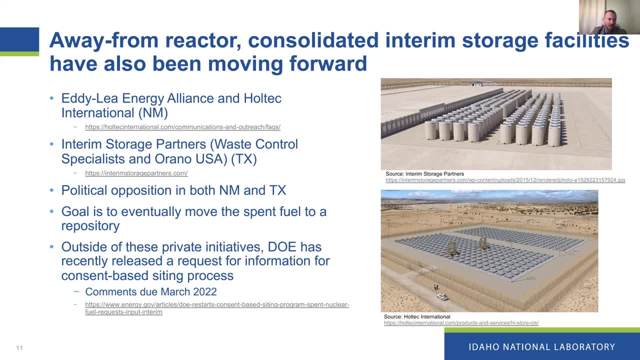 some uh to a repository in the future? one other thing that is of interest is: do we, outside of these private initiatives, has been looking at citing a consolidated storage facility and specifically they just released this last week a request for information from interested communities parties on what citing uh, what the process for citing such a facility would look like. 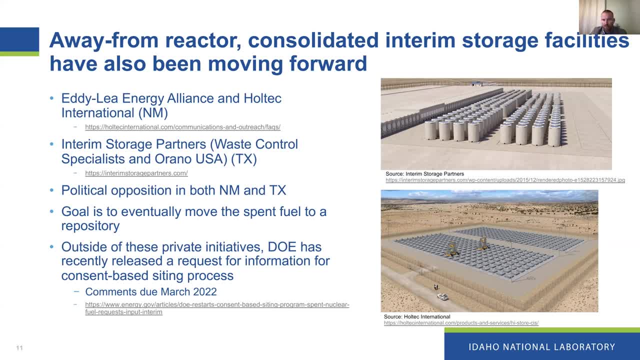 so i uh i did include the link there. if there's uh communities in in wyoming or other places that might be interested, i do encourage you to go and respond to that request for information. uh, comments are due uh right now, i think in early march. so um next slide. 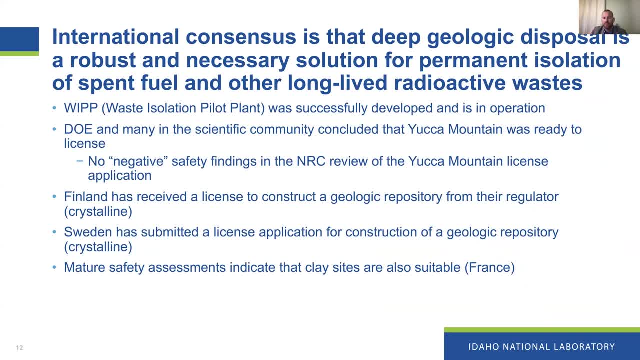 all right, there we go. um, so the. the final step for the the fuel cycle is, is repositories, and that's the deep underground repositories. i'm going to go ahead and show you a little bit more of that in just a moment. but i'm going to go ahead and show you a little bit more of that in just a moment. um, these can be done technically. 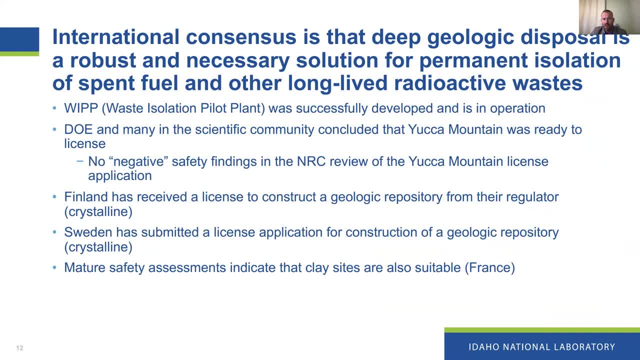 though not for spent fuel. there is a deep underground repository for long-lived radioactive waste- transuranic waste- in new mexico, the waste isolation pilot plant whip, so so that that facility has been operating um for the last couple decades um there have been some some some issues there, but it's now up and operating again. but it is not licensed for spent. 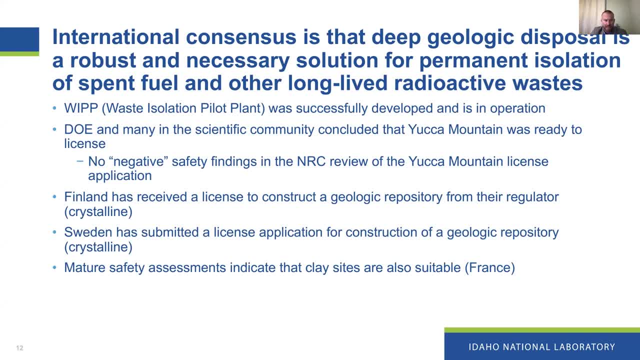 fuel. the yucca mountain site in nevada was the um really technically on the books of still the us repository site um. however, the federal government has basically said this is not a workable option anymore, not for technical reasons but for for more political reasons. the nrc actually. 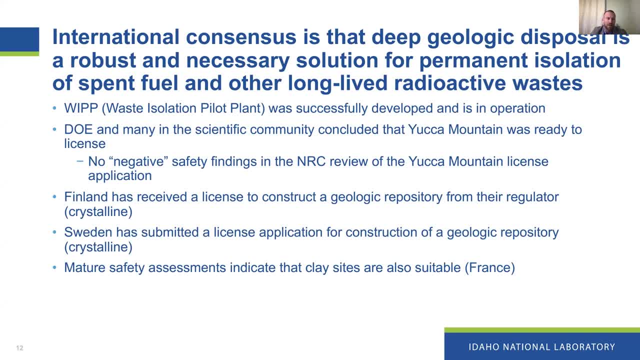 did sort of evaluate the yucca mountain license application and did not come back with any sort of technical show stoppers. uh, there is a lot of evidence that says there's there's sort of展. There's still some other things that have to happen. 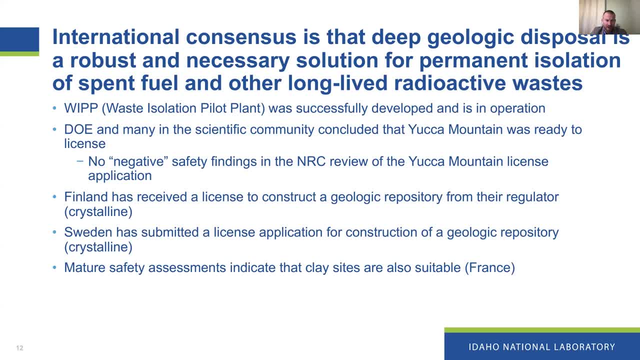 But for now that program is sort of on pause in the country. There have been three other, well several other countries that are moving forward, mainly in Europe, that are a little farther along in this deep repository. So then one more slide. 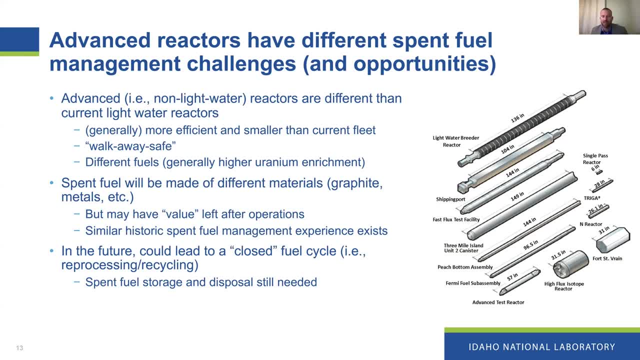 All right, So the advanced reactor. So this is- maybe I'll just tie this back into Steve's talk- But you know the advanced reactors are different sizes, They're different shapes And they have different fuels And you know there are opportunities and challenges associated with that. 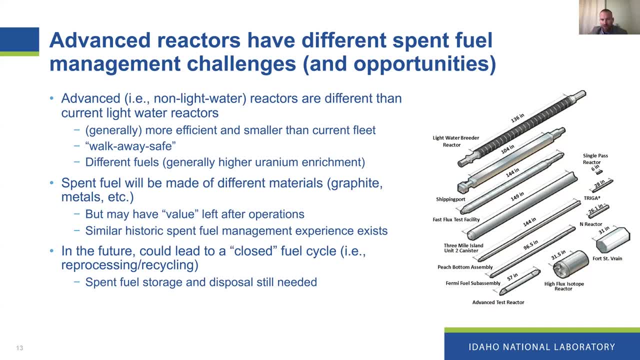 Again, I think some of the discussion on EBR2 and the safety case lends itself to this sort of walk away. safe, I think, is the term people have been using, But generally, as I mentioned earlier, the fuel needs higher enrichments. 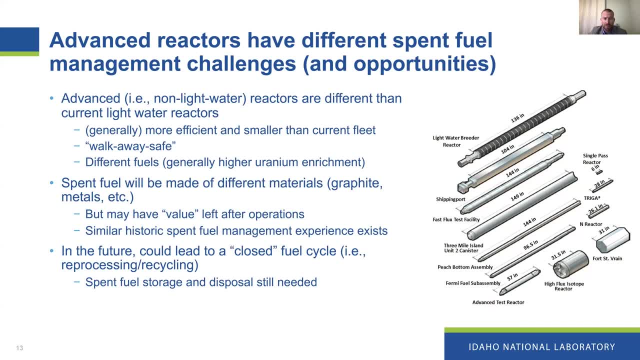 And so, because of that, you may choose different materials and different fuel forms. Right, Right, Right, And so there are several different fuel forms. There's metal fuels, There's graphite fuels, Molten salts are being considered. All of these have different sort of challenges with the fuel cycle. 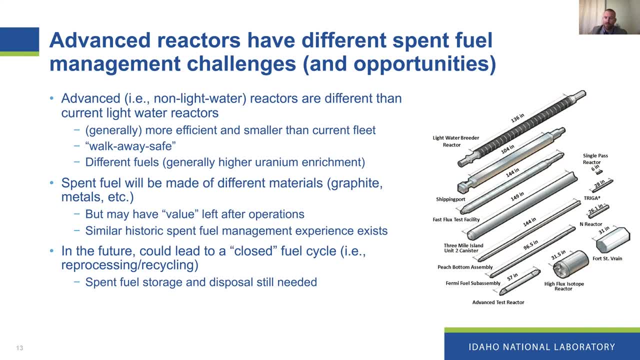 Again, because you know the fuel cycle that we have now, like fuel fabrication, for example, is focused on uranium oxide, light water reactor fuels for the most part, And so you know, looking at these other fuels, we need to make sure that we have that capability to fabricate. you know different fuels. 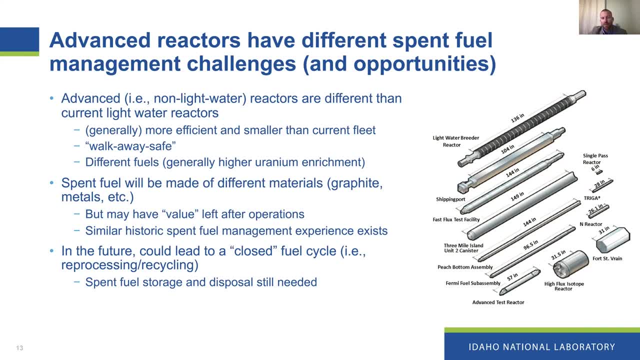 And so that's it. That's something that's a little different. The other piece is: you know that very first slide I talked about. in the US we're in this once through cycle. They call it the open fuel cycle. 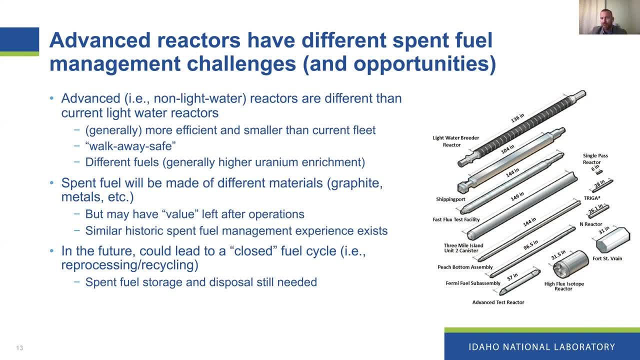 So we don't reprocess Some of the disease. advanced reactors have the potential to really jumpstart some of the reprocessing, recycling conversations. to close that fuel cycle, A lot of the fuels you know at 20% enriched, you know after discharge they might, you know, be 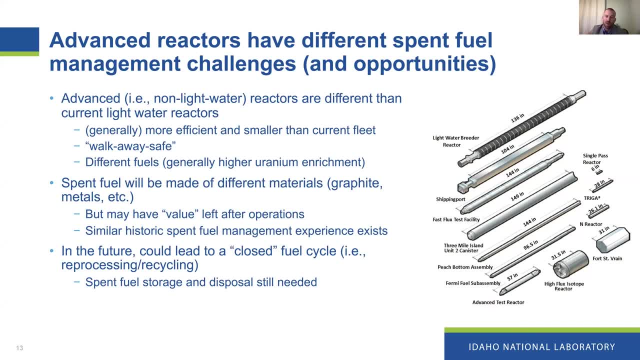 Be very useful for other uses, And so we are seeing, by the way, that this recycle, specifically looking at getting access to fuel for advanced reactors, The EBR2 reactor that was mentioned earlier. actually, we are recovering that uranium and down what we call down, blending it to about 19 to 20% enriched for future advanced reactor needs. 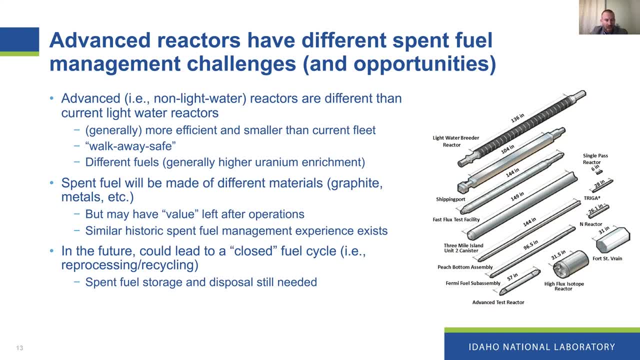 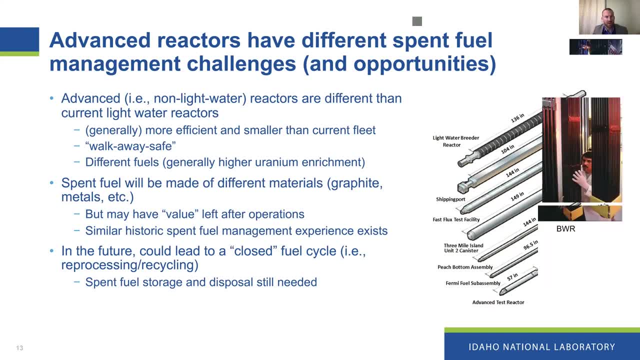 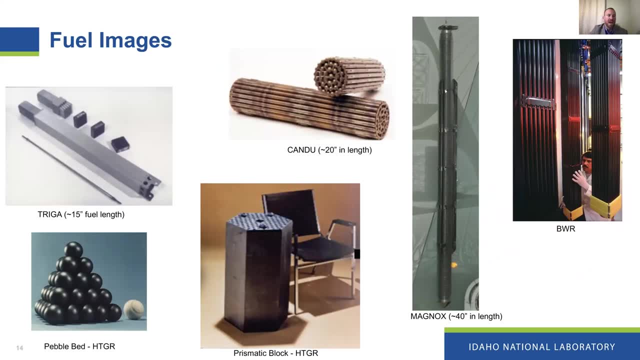 Maybe go to the next slide See here. I'm still There, we go, And just maybe I'll just leave you with some of the different images. So so the far right one is is a light water reactor. So these are very square, thin, tall uranium oxide, Zirc clad fuels. but we have extensive experience actually with several reactors that have 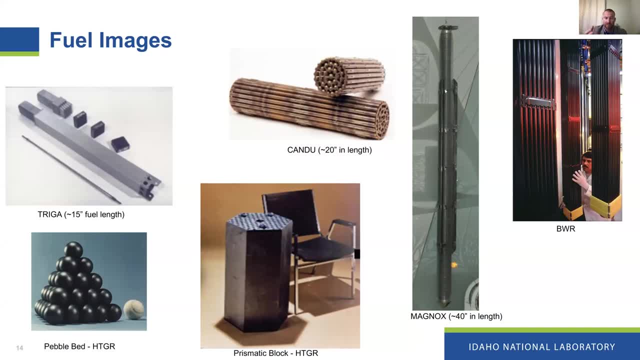 other fuel forms And there are lots of different sizes and shapes. The bottom left is actually a pebble bed reactor, So those are actually spheres of graphite that have uranium- what they call triso particles- inside them. But we at INL, and specifically the National Lab Complex, have been 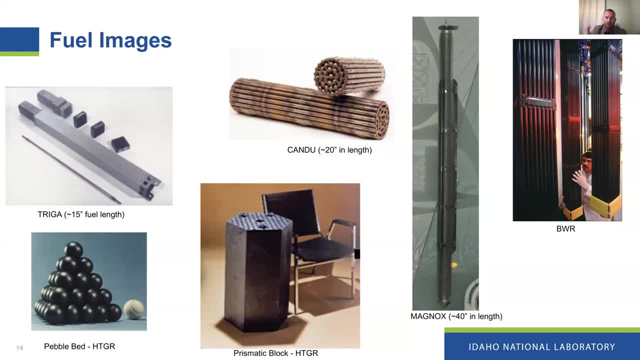 looking at different reactors. All these reactors that have been proposed as advanced reactors have some basis in research at the labs, whether that's a fuel development, whether that's performance, material and corrosion capabilities, those sort of things. So these have been looked at for several decades across the complex and national labs and through DOE and others. 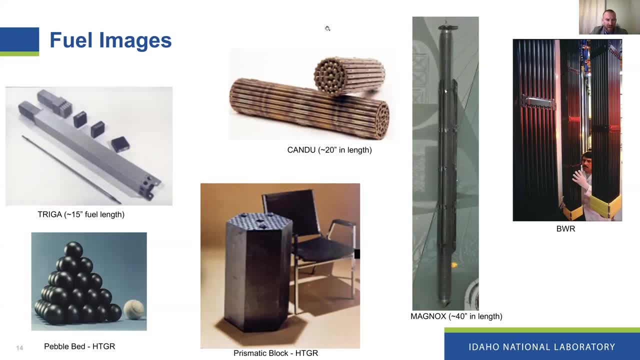 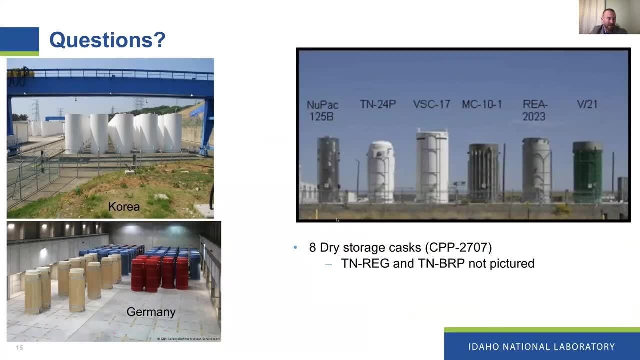 So I think that's it. If we go to the last slide, I think it's just images of the spent fuel cask at different places. The one on the right is actually at INL. But I won't answer questions now. I want to leave time for the next speaker and then I'll be happy to answer questions. 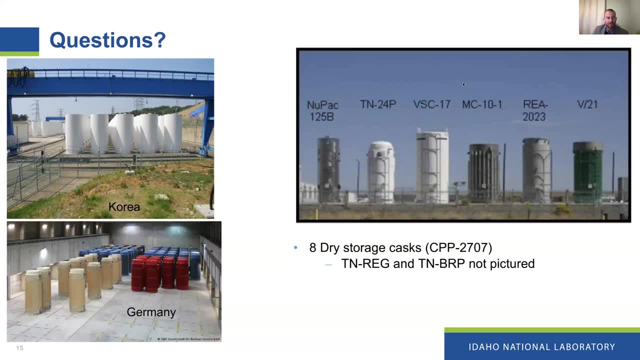 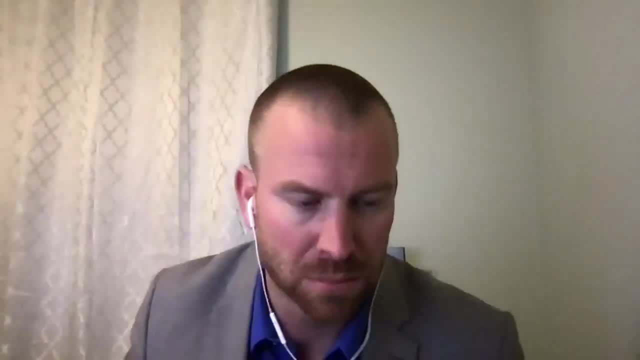 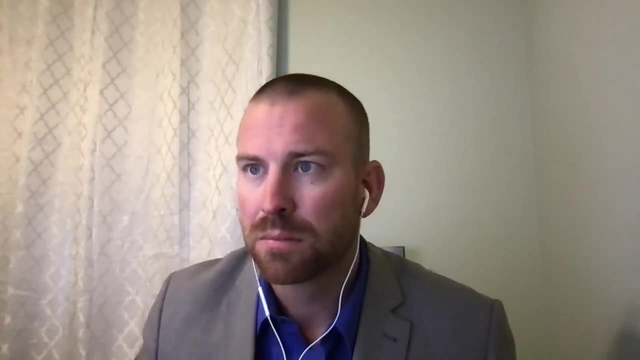 at the end. So thanks very much. Thanks, Josh. There was a question come through about posting that link to that consent-based citing RFI. Everybody, if you're still interested in that, go to the Q&A, open up that Q&A box and go to answered. It was a question, a request, by Emily. 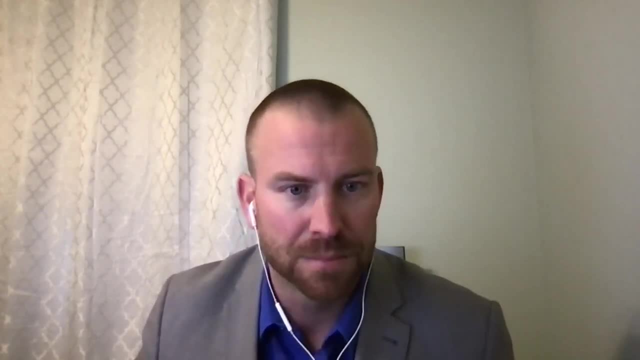 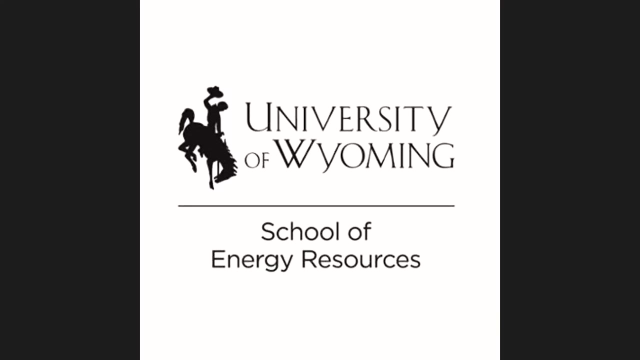 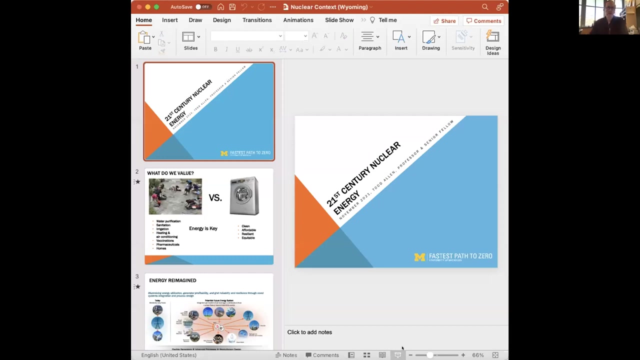 Nichols and I have posted that link released. That link should get you started, I hope. Okay, Thanks a lot, Josh. Our last speaker today is Professor Alan from University of Michigan. Over to you, Professor. Thanks a lot, Glen, And thanks Steve and Josh for the presentations. A little bit history. 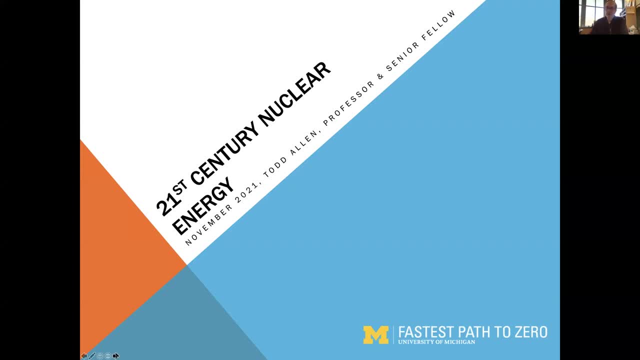 I'm currently the chair of the Nuclear Engineering and Radiological Sciences Department at the University of Michigan, Sort of going backwards through my career. i've taught here at michigan, i've taught at wisconsin, i've worked out at the idaho national lab site where steve's at first as a early career researcher and then later as the deputy lab. 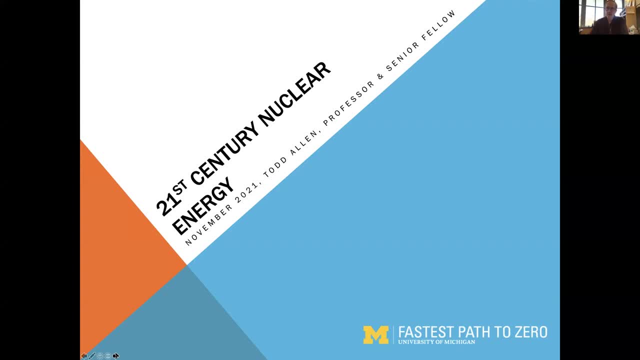 director for science and technology, so i have experience with the national labs. i've worked at a think tank in washington dc and i started out my professional career as an officer in the us submarine force. that's where i actually learned how to run a nuclear reactor. so my 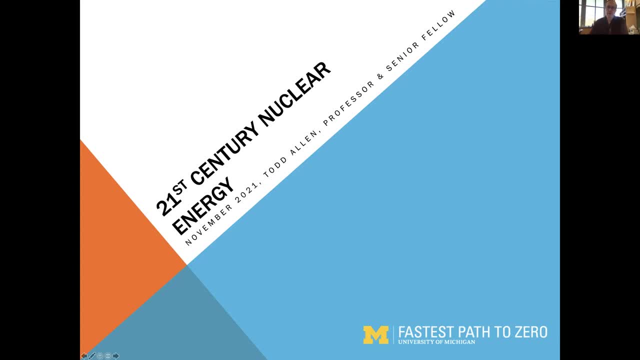 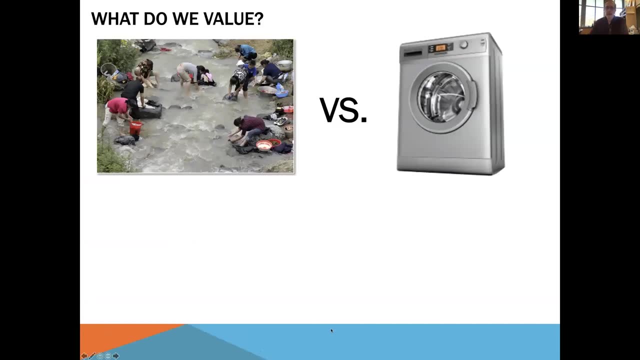 remarks really to talk about where we are in the 21st century with nuclear energy. so next slide, please, and go ahead. click one more. all right, thanks. so i'm going to start out my talk by saying that energy is important, right? energy makes our lives better. the two pictures at the 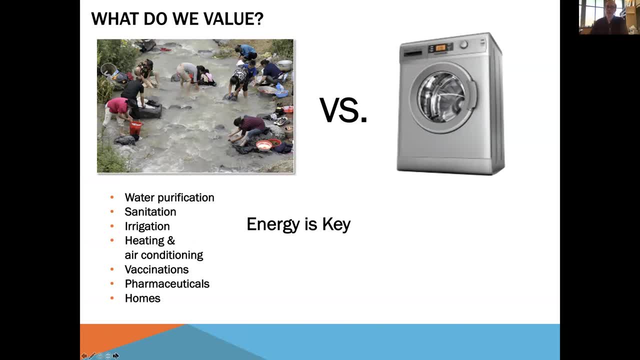 the top demonstrate differences in life. that's available or possible due to energy access, and it's- it's more than just you know how we clean our clothes. it's, it's how we get water, irrigation, heat and cool our houses, vaccinations, everything right if you click one more time. 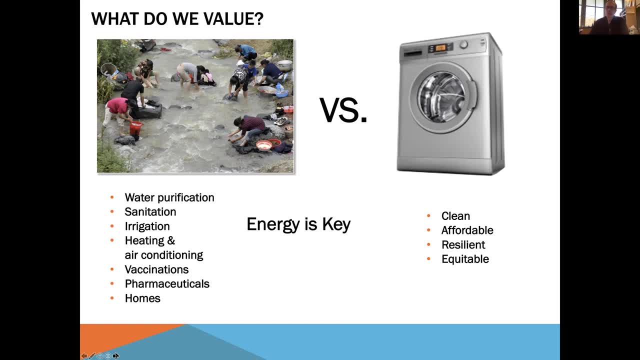 what we keep demanding as time goes forward is that energy gets cleaner, that it gets more affordable, that it gets more resilient- right, it's, it's always on, or when it does go off, it returns quickly and more and more. that the benefits and risks of energy use are distributed more equitably. right, so i think that's where we are, where we are. 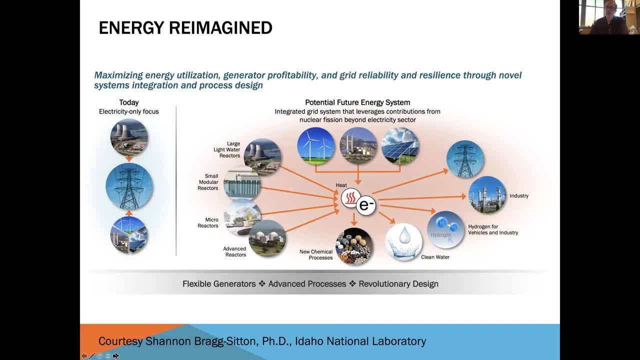 next slide and um playing off a slide that that steve also used. this energy system is in a an amazing transition. so i look back at to when i was a kid and the electricity system was very simple. right, we would make electricity at large central station power plants and we would 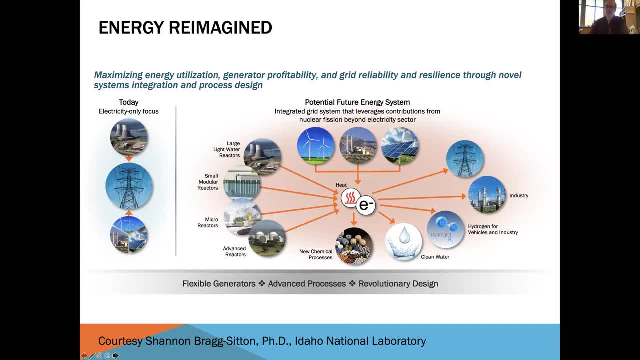 send it via transmission and distribution lines to people's homes. right, it's very simple. now it's much more complicated. right, we've added variable sources like wind and solar. why? well, because the fuel is free. right, we don't have to pay for sunlight, we don't have to pay for. 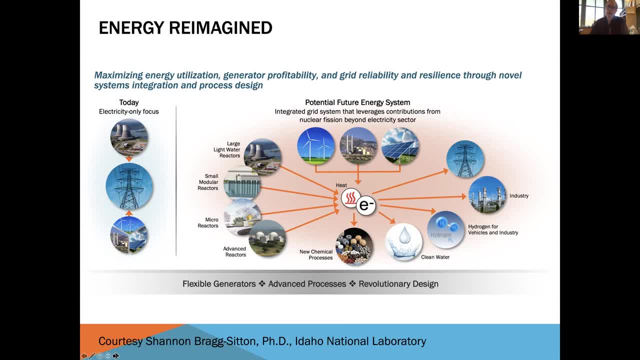 wind, and we brought the costs down for those energy sources, so they're being added to the grid. computer information technology allows us to ramp up up and down on a real-time basis the amount of power we use in our homes or in our businesses, industrial facilities, and so, in the context of nuclear energy, we've gone from a system that 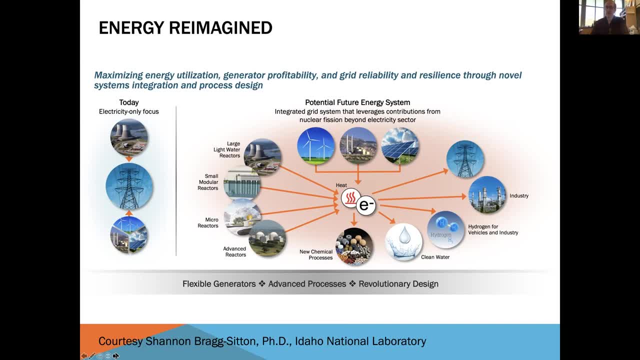 really encouraged us to build very, very large electricity generating machines and we're moving into a world where there's an opportunity for a lot of different products, right, and i think you saw that framed out in steve's talk, so that's sort of big picture. item one is the opportunities for 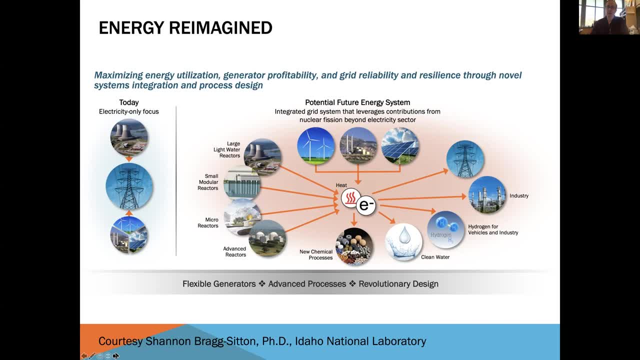 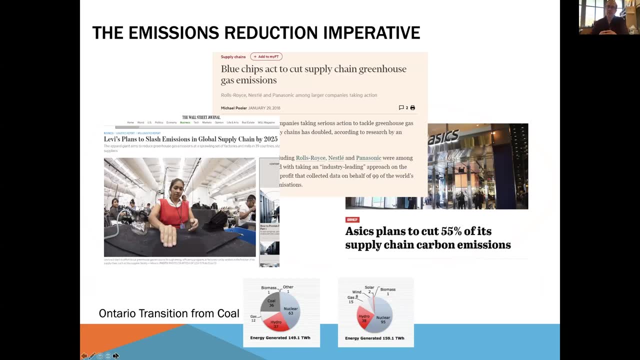 all energy technology, including nuclear, are changing, right. okay, next slide. and i think you know that the things that people care about that drive energy choices, including nuclear energy, are driven by things like emissions. right, i mentioned we constantly want our energy to be cleaner, right, a lot of discussions now where cleaner means less carbon. 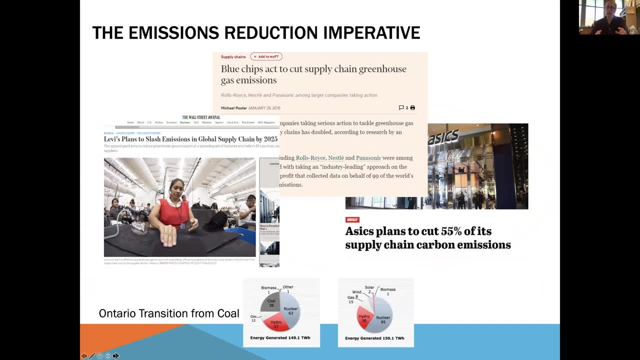 but you know, over time it's also meant less particulate and a lot of other things, right? no one really appreciates, uh, when their neighbors burning a lot of stuff in their backyard if the wind's heading towards you, right, so we're driving towards cleaner systems, whether you're the user or 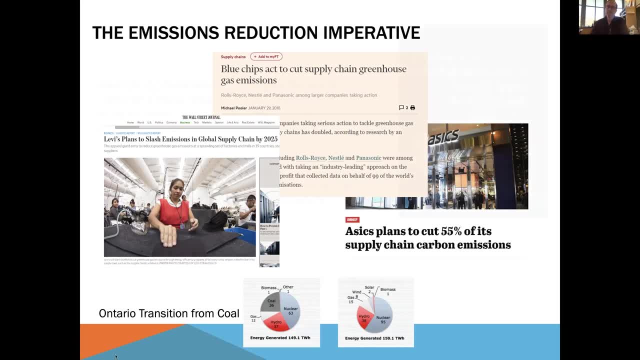 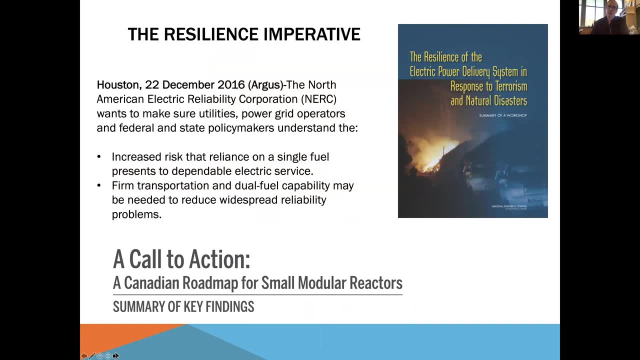 whether you're the producer. okay, next slide. we want systems that are more resilient. uh, use the the cold energy event in texas this last winter where lots of things went wrong because the system wasn't resilient. right, gas, gas lines were freezing um. some of the renewable sources were taken offline. one of the four nuclear plants in the 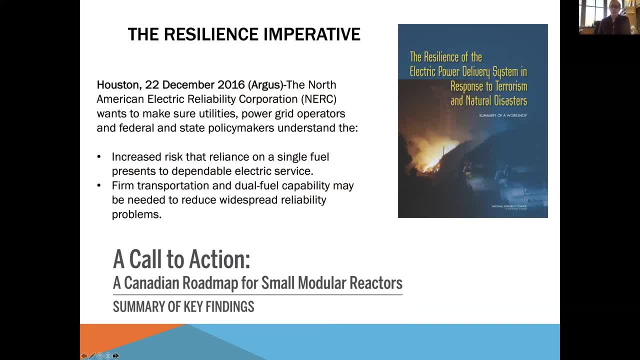 state uh had to be taken down right. so, as we're looking at new opportunities for energy systems, it's also: how do i create energy products right that not only deliver that clean electricity but make sure, right that it comes to people's homes or their businesses in a very consistent? 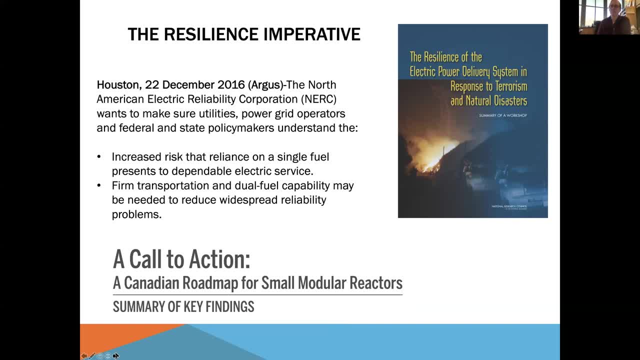 manner. i think that drives us to using systems of energy technology rather than sort of single types and um, you know, i personally believe that's why nuclear has a strong future in a clean energy world, because each different type of energy production system does something well and is not not as good in other things. all right, it's the system that matters, okay. next, 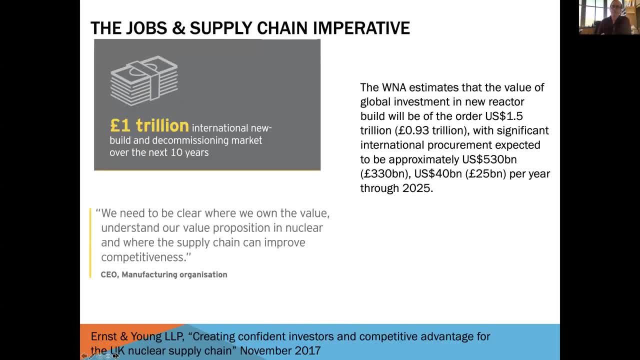 slide, please. um, the jobs and the supply chains matter, right? this is just one estimate from the world nuclear association that says: you know, we're talking about trillions of dollars over a decade in new jobs associated with growing the nuclear supply chain. right, where is it growing right now? 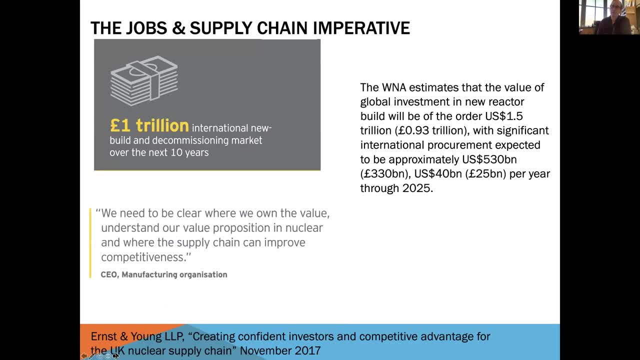 it's growing very fast in countries like china. united arab emirates has recently built a lot of plans, india has plans, and so, in addition to supplying clean energy for domestic uses, there are jobs and supply chain initiatives associated with that, whether that's domestic or international right. so 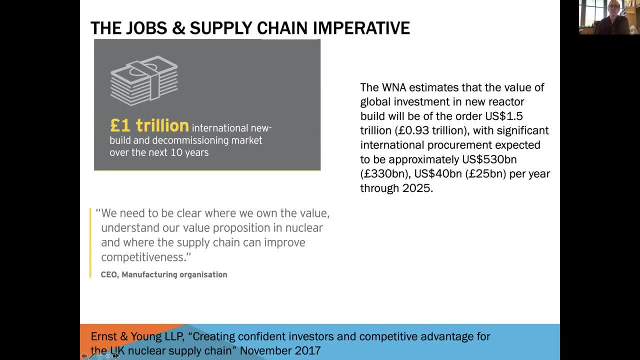 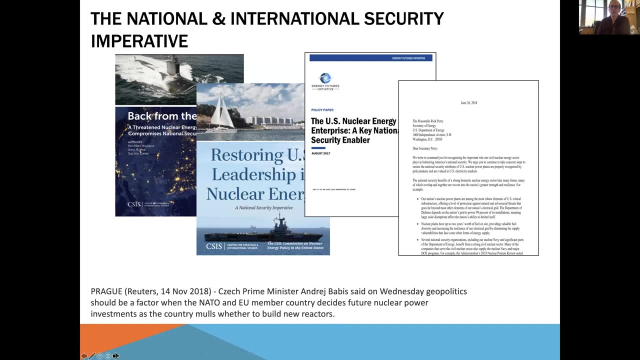 there's a lot of value right placed on the jobs that are associated with with um being the, the communities that host energy technology. all right, next slide, please. and then in a lot of cases there are national and international security- uh questions around the holders of energy. this is true in the nuclear world right, where we talk about the ability to control or influence. 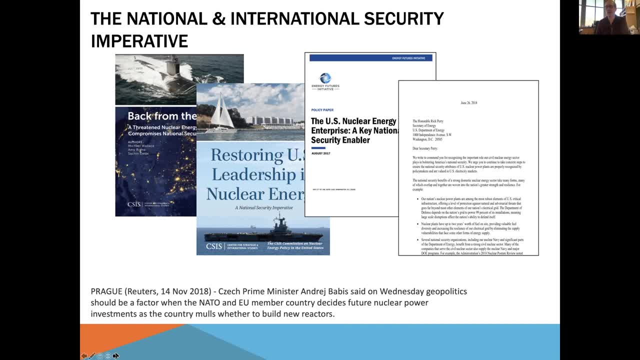 international norms on safety and security and safeguards and how. it's very difficult to do that if you are not part of the international or national nuclear commerce. i think national and international security issues are bigger than just nuclear. i mean you see this in questions like national natural gas pipelines that come from russia into europe and whether or not that's a 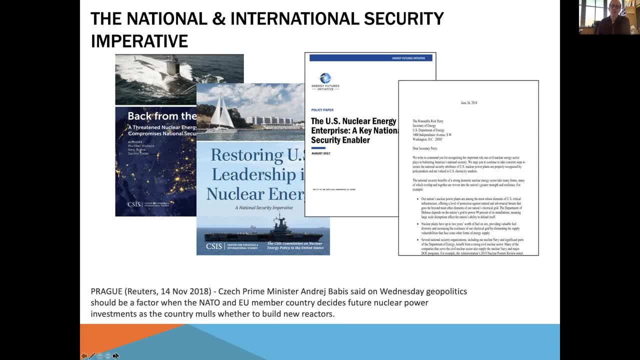 stable platform for energy security needs in Europe. right So lots of different values associated with how we create and use energy technology And the choices made around those values are also opportunities, right In order to provide clean energy, resilient energy, the jobs associated with that and the national. 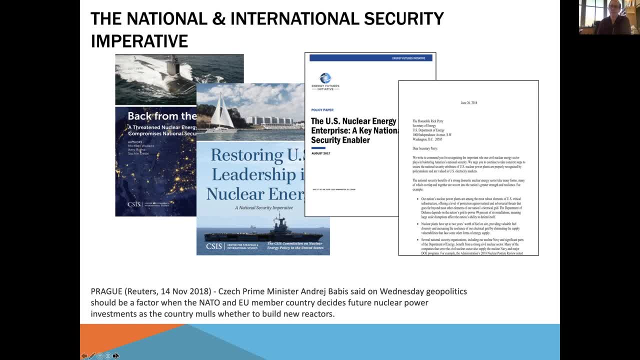 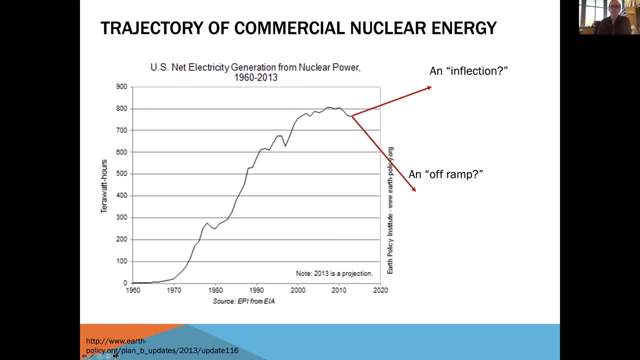 and international security implications of the types of energies that we use. All right, next slide. So where are we in commercial nuclear right? So we started building nuclear power plants in earnest in about the early 1970s, late 1960s, And we built them at a pretty rapid clip. 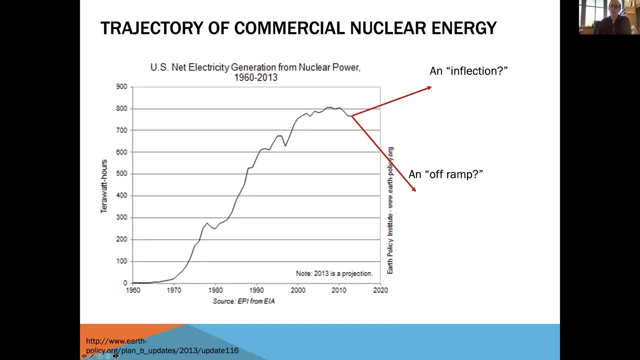 for about three decades. So we were building about 30 big nuclear plants And as a thumb rule, a big nuclear plant is millions of homes in one plant, So you had a tremendous amount of electricity out of them- This one over about three decades- and we leveled out at about 20% of the US electricity. That's. 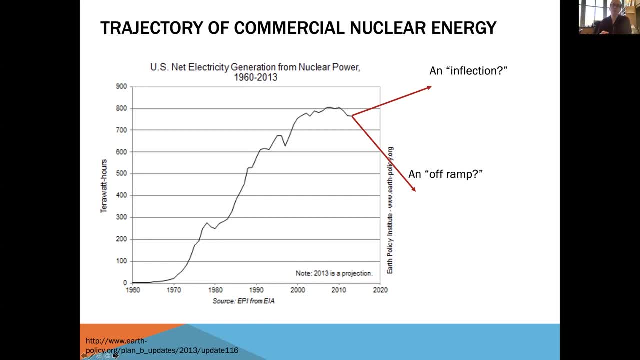 over half the zero carbon electricity in the US right now. So nuclear is a very significant portion of the zero carbon electricity in the US. Over the last 10 or so years we've changed the markets, we've changed the way we reimburse, in a lot of cases, energy producers And in some cases, 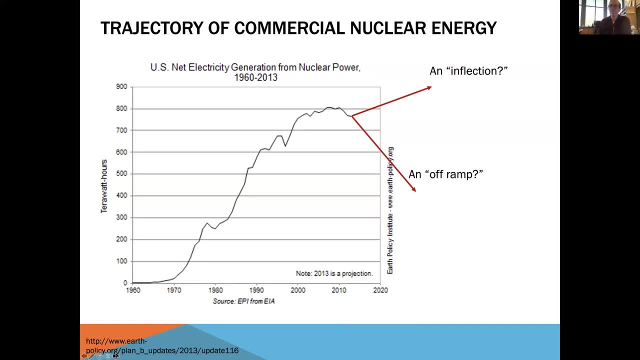 we've started to build more and more nuclear plants And we've started to build more and more wind farms and we've started to shut down some of the earlier nuclear plants- Still around 20%- partly because we're getting much, much better at operating the first-generation plants and 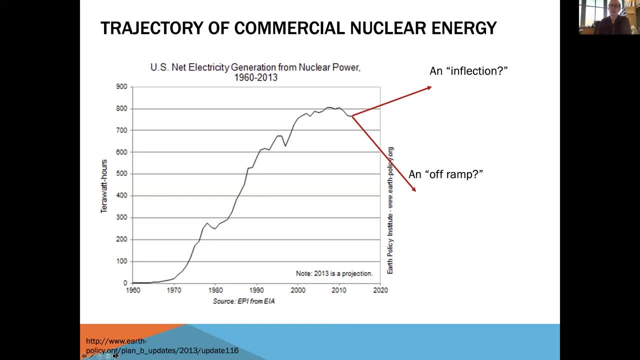 therefore they're down less for maintenance and therefore we're getting more electricity out of a single plant. But we are at a point where we've started to lose some of the plants. And there's this question: right, Are we at an off ramp or we'll slowly shut down the rest of the plants? 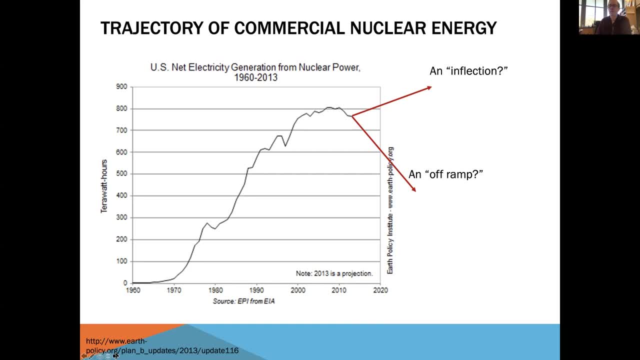 Some of these plants could run another 10,, 20,, 30,, 40 years. Or are we at an inflection point where a new generation of nuclear products that fit into that more complex energy picture that both Steve and I used come into the market? 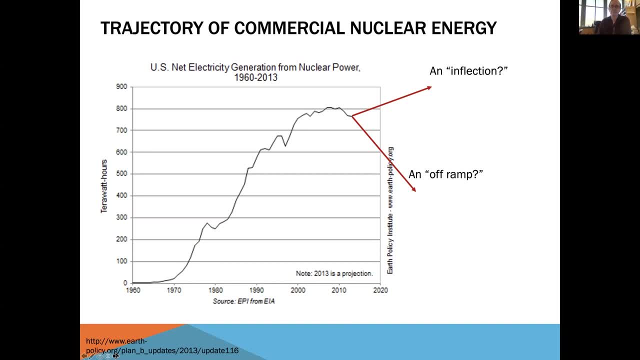 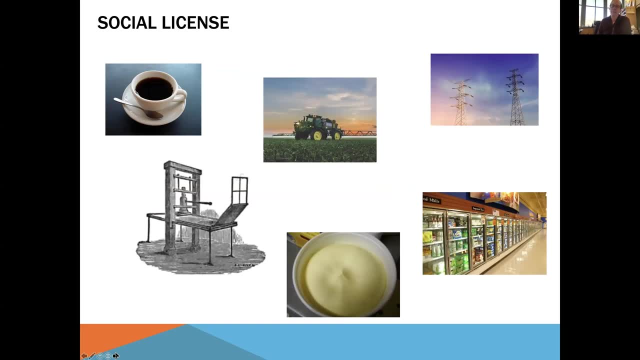 So that's where we sit right now We go to the next slide, And it's a really interesting discussion to me. because I like this slide? because I've grabbed six examples of products that now we take for granted that the benefit we get from those are more than any possible risk associated with them. 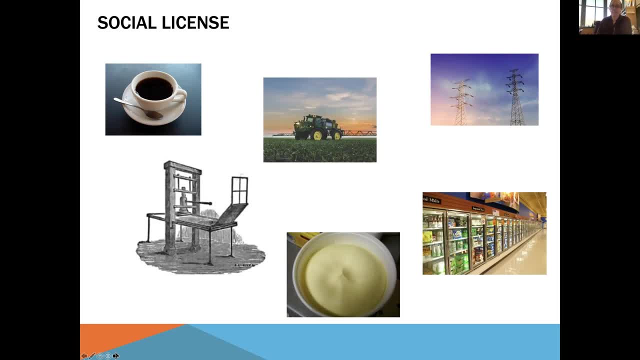 And sometimes, if you haven't read the history, it's surprising that these were ever controversial. So, starting in the upper left-hand corner, I've got coffee, I've got mechanized farming, I've got electricity, mechanized refrigeration, I've got margarine and a printing press. 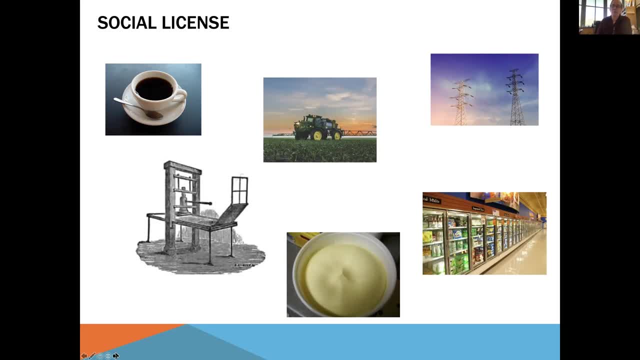 And in their day there were big discussions about whether incorporating these technologies were an advantage or whether the risks were too much, And I'll use the lower right-hand picture of mechanized refrigeration as my favorite example in this story, because there was a time in the US and worldwide where we were 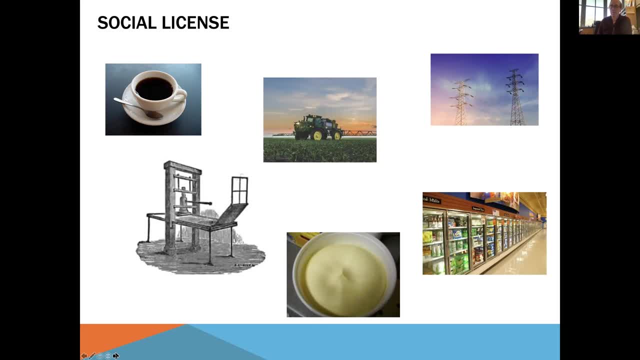 arguing whether refrigerators or ice was a better option. It's a better way to look at it. Let me give you a second. So there was a time in the US and worldwide where we were arguing whether refrigerators or ice was a better option than a conventional method. 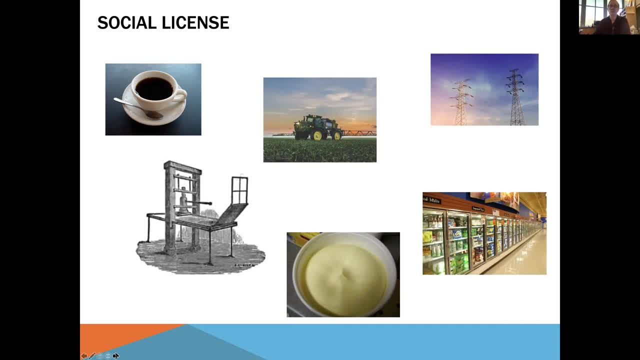 way to cool our food and there was a big commerce associated with with transporting ice right around the country and there were big arguments about whether, um uh, mechanized refrigeration was unnatural in some way and changed the properties of your food, and that that ice was more natural. 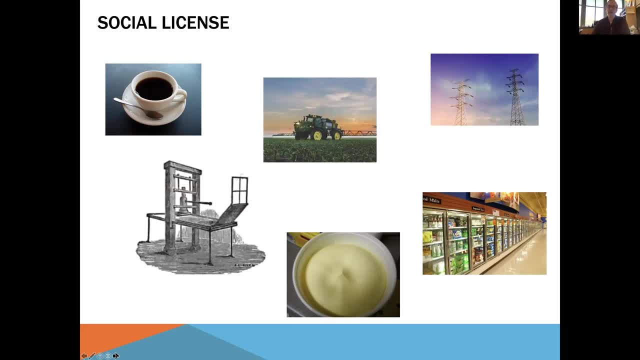 but over time, right, we've sort of evaluated the risk and benefits of these, these various technologies, and they've been common and i just i think it's interesting history because we're at the end of the first discussion around nuclear power, right, we're looking to see what improvements. 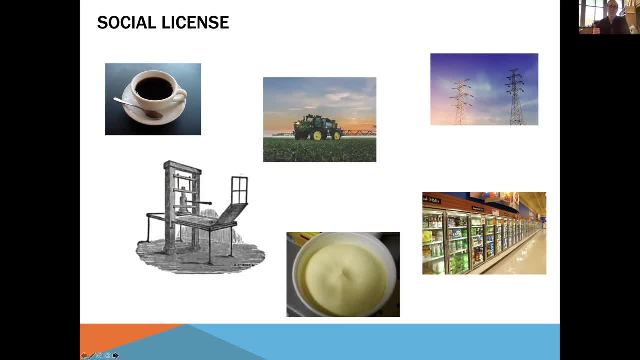 to the technology will be available in the second generation, both in what they do right but also in some of the characteristics like steve and josh talked about. so i think it's a fascinating uh time in in nuclear and i'm pleased to be part of that discussion. so next slide. 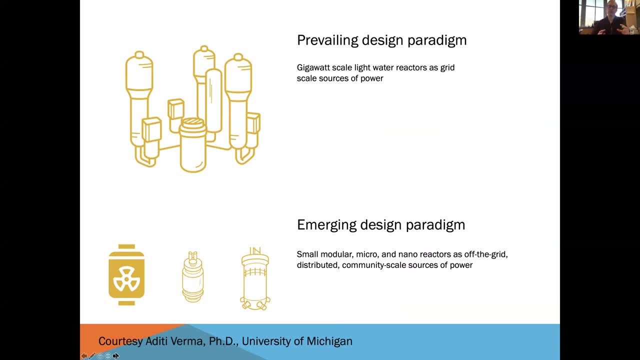 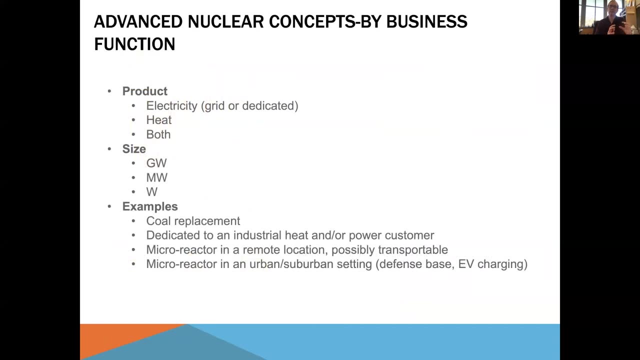 and, as steve mentioned, we're going from a sort of a design paradigm where we had one type of reactor right, we this the system in the 70s. um, uh, stay on that. pass on for a second. um really incentivized us to build these very large, complex systems, and steve talked to you. already about some of the consequences of going to that size relative to safety systems and other things, and now, as we look forward, we've got a new paradigm that's saying maybe big is not the only way to design a product. clearly, some of these big reactors are still of value in places. 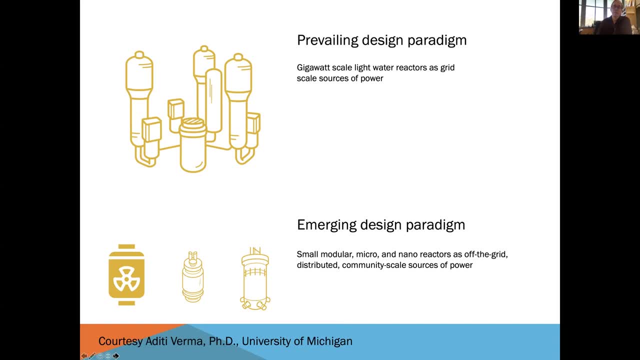 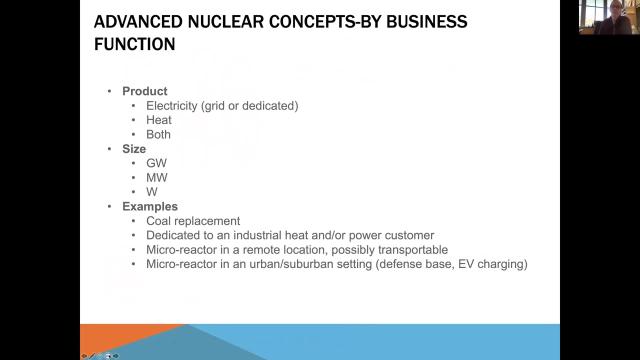 like china, where they're building them, but internationally, a gigawatt scale reactor may not always make sense, and so we're looking at things that are smaller and modular and maybe off-grid. okay, next one, and a lot of times you'll get you'll hear people talking about next generation. 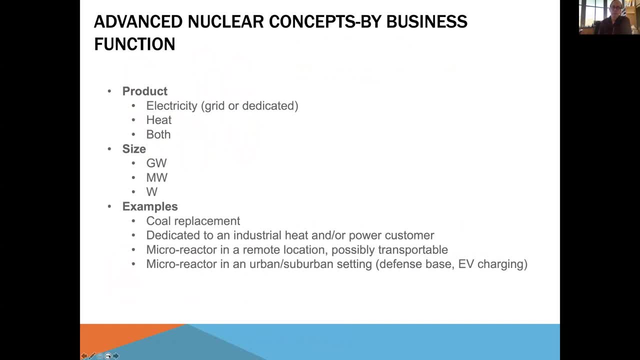 nuclear in terms of technologies. right, it's a sodium-cooled reactor, it's a gas-cooled reactor and that's interesting from the technologist perspective. but i think from an average person perspective, what's more interesting is the business functions, the things that people are, are aiming to develop these. 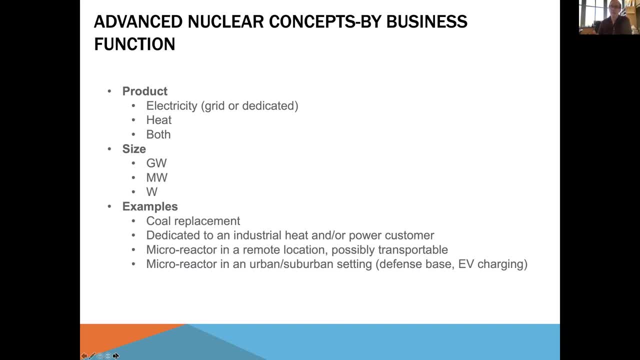 products for. so, yes, still electricity. maybe in some cases electricity on the grid, but some cases it may be off-grid uses or dedicated electricity to a specific industrial user. it could be heat: high temperature heat for industrial processes, low temperature heat for heating homes and businesses or agricultural use, or sometimes 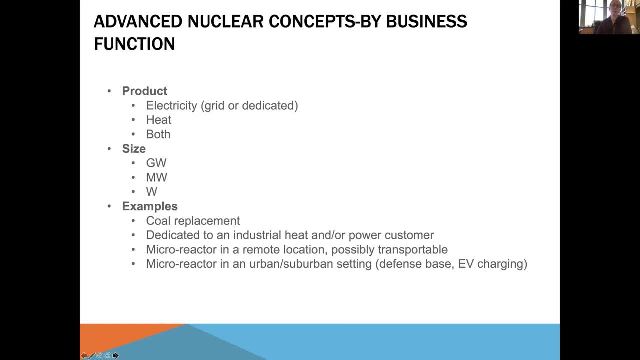 it's both right: a single system that can transition back and forth depending on where the energy is most effective and useful at a specific time. the size is different: first generation, all very large designers now looking at everything from a gigawatt to things that are about one thousandth the size of a first generation commercial plant. 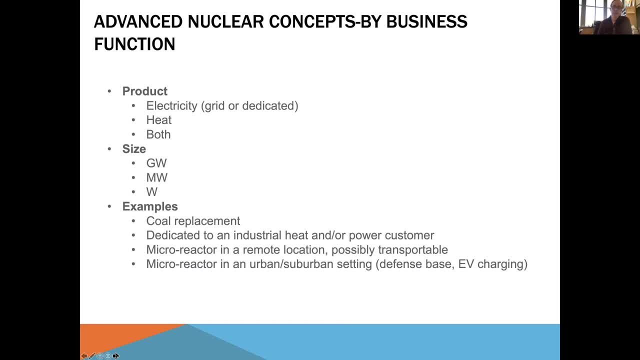 and this includes opportunities, and these are just a few examples. it's not meant to be exclusive, but replacing a coal plant with another electricity generating nuclear plant, dedicated industrial heat or power to a consumer. you may have read things in the paper about nuclear companies signing agreements with bitcoin mining companies right bitcoin, whether you like. 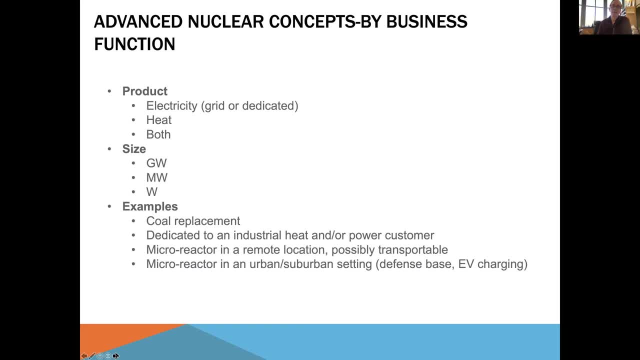 it or not, if you think it makes sense or not, it uses a lot of energy, right, and if so, and you want do that in a clean way, nuclear may be the answer for that. dedicated power, Off-grid, remote locations that may currently use something like diesel, which could be expensive and needs to be transported. 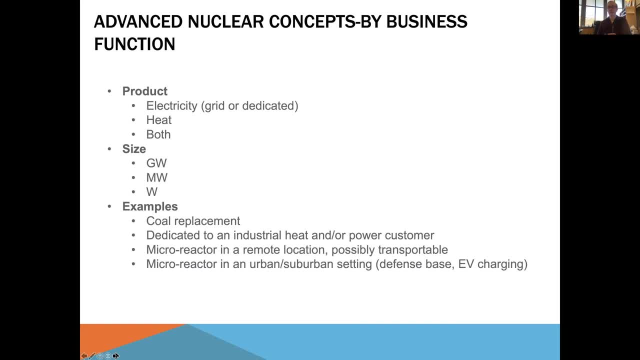 maybe a very small reactor fits in a place like that. Similarly, maybe a very small reactor makes sense in something that's more urban or suburban, like EV charging- right, If we're going to go towards large numbers of electric cars, they've got to be charged by something, right, Maybe? 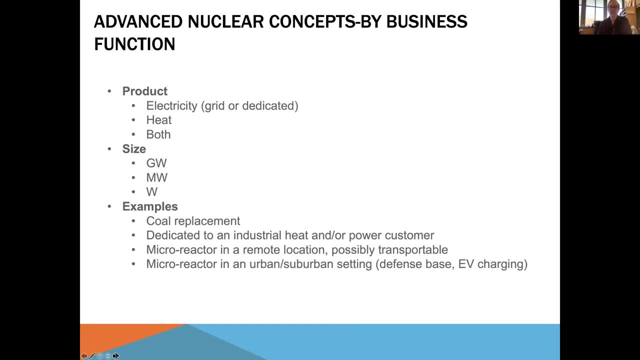 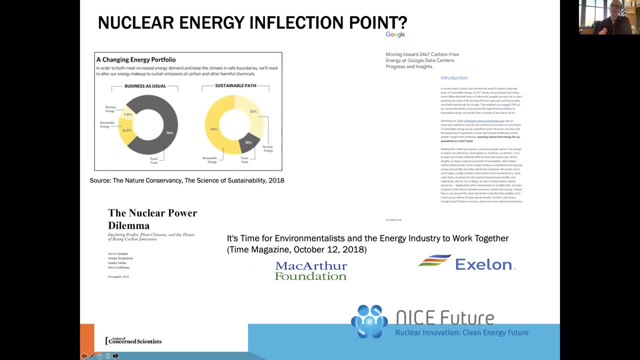 a micro reactor would make sense in that case. So it's different business functions, All right. next slide, And at this inflection point I at least notice the conversation pivoting some right, In the sense that, and in a lot of cases the discussions are around climate change. 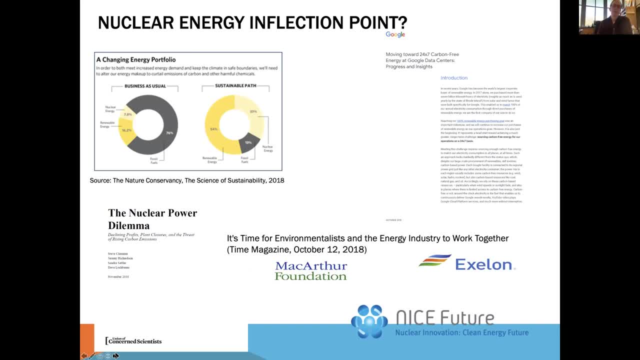 but it's not always- But organizations that you traditionally might not have thought of as standing up and saying publicly that there's a value to nuclear energy becoming visible, And I just I'd list a few here, right, So the Nature Conservancy. 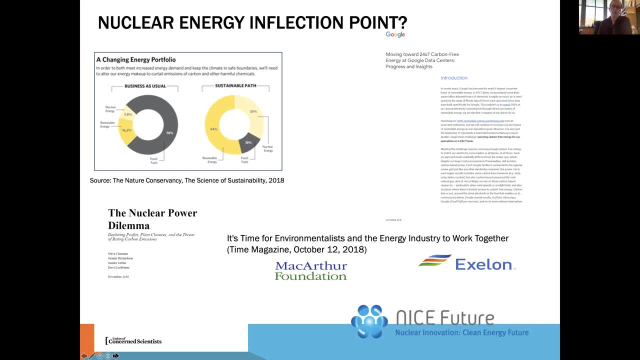 big environmental organization. their long-term plan says: you need nuclear as part of the future. Google says to power their server farms 24-7 carbon-free. you need nuclear. Even organizations like the Union of Concerned Scientists, which have never been big fans of 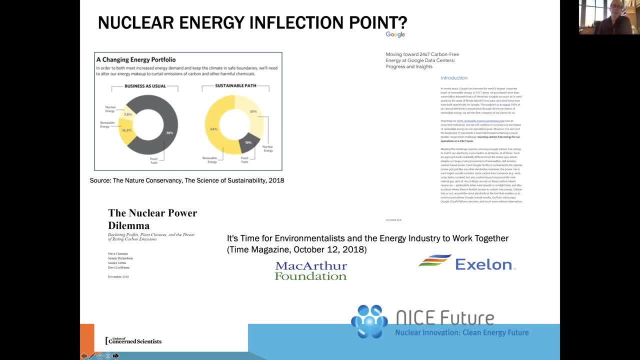 nuclear have at least come out and said: please don't shut down the current generation of nuclear plants. And they're not going to shut down the current generation of nuclear plants, All right. so I think in the technology sense it looks like we're it may be at an inflection point. 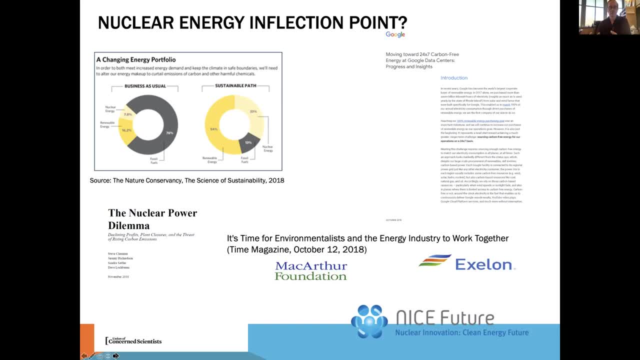 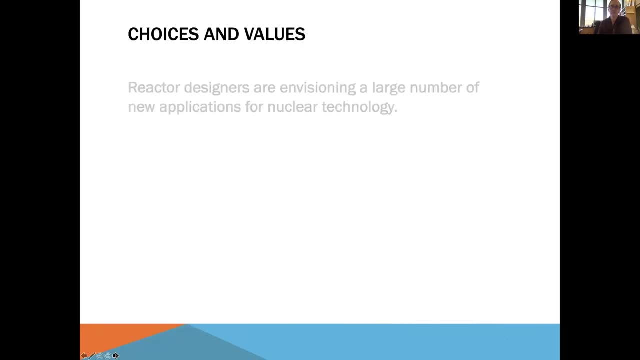 There's certainly a lot of companies looking at different opportunities in the public discussions, right? In some ways it feels like we're having a different discussion than we might have been having 20 years ago. Next slide: All right, so it gets back to sort of choices and design. 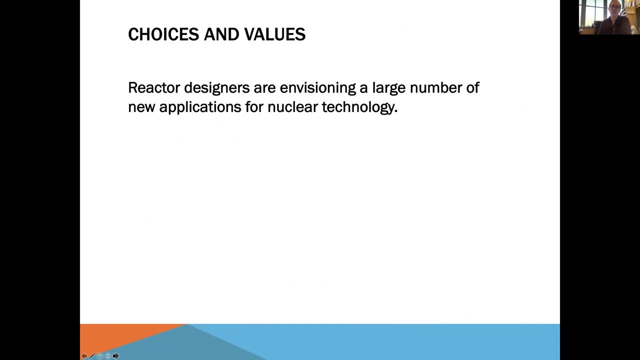 choices and values. right, The designers are envisioning a large number of new applications for nuclear technology, right, But what's that mean for a community? So, if you go to the, I would argue that communities are in a position to envision a large number of deployment scenarios. 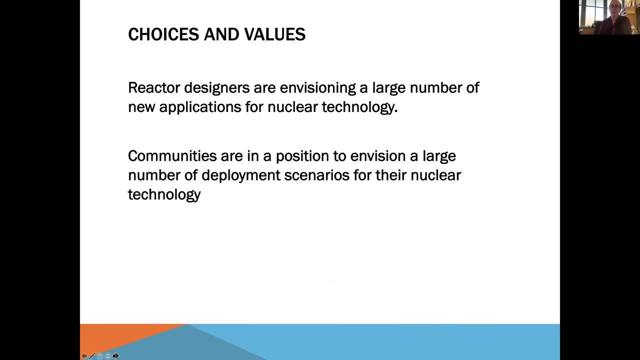 for their technology right. In the past, communities were typically a host for a technology that someone else designed and brought to the community and said, hey, would you like to be the host of this right? I think now communities are in a position to say we would like to be the host. 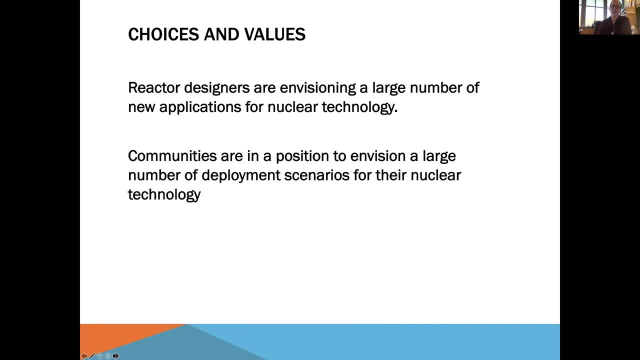 but we would like to get a lot more out of it. right, that aligns with our values. right, that might have been the case in the first generation, 1970s deployment, So click one more. I mean, my suggestion is communities should lead rather than react. 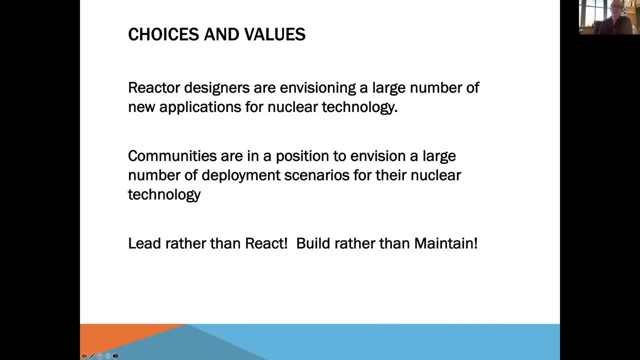 right, Don't wait for somebody to come to you and say, hey, I've got an idea for a power plant, are you interested? And second build on it, rather than just maintain what you have. Steve talked about this a little bit. I'll talk about it some more. I think there's more value in just 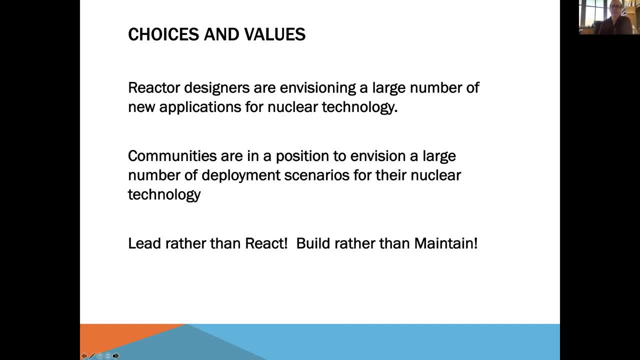 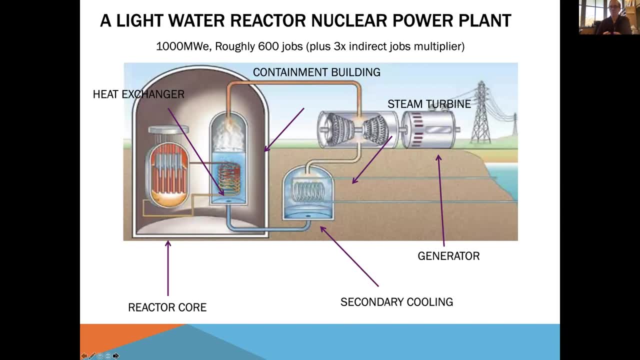 the electricity or the energy that you're putting out of the plant. Okay, next slide For a little context. this first generation nuclear plant: a thousand megawatts, one gigawatt. right, It's a very simple plant. I mean, the whole point is. 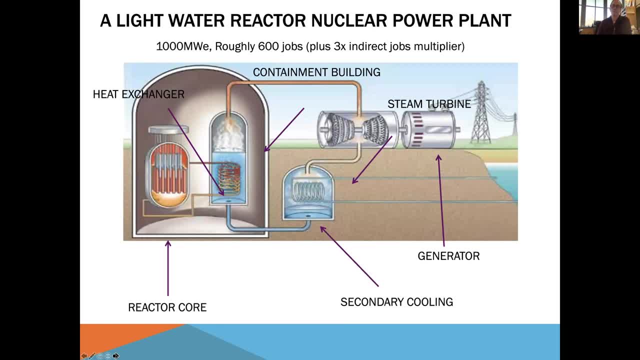 you use a nuclear process to generate steam. you use steam to turn a turbine. the turbine's connected to a generator. you make electricity right. Those large plants are good job creators in communities. So roughly 600 jobs. typically people talk about a three times multiplier. 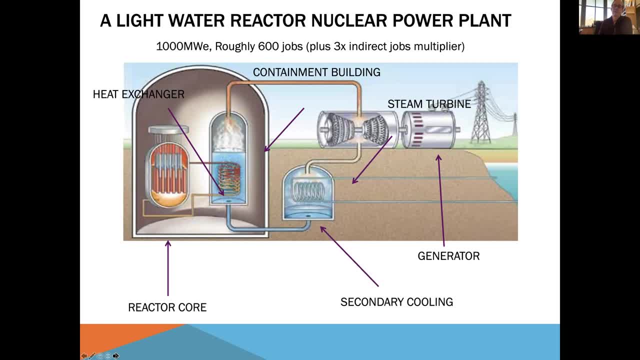 right: Three jobs in the community for every job that's at the plant right. So that's why for a lot of communities that have been hosts of nuclear power plants, one of the values direct to the community right are the jobs and the associated. 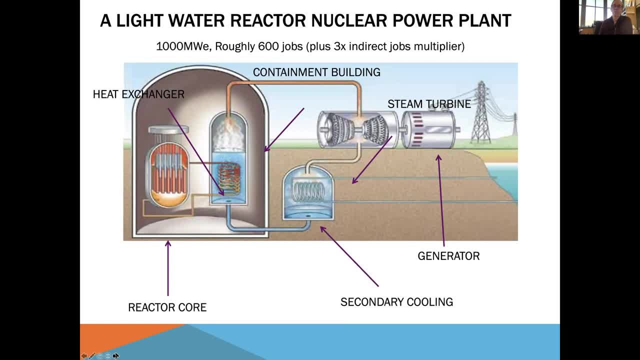 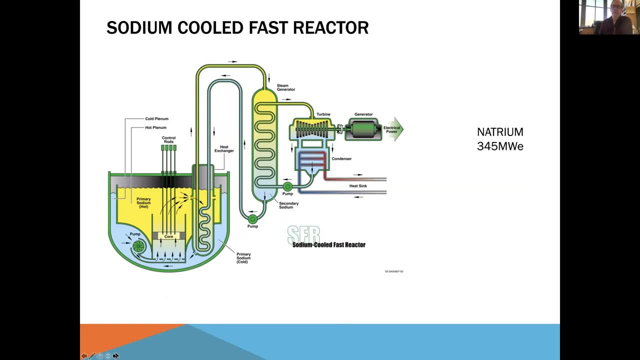 value that comes with that If you click one more. this is just a cartoon. it's not meant to be exactly the matron design. But one thing to note about a lot of the advanced reactor concepts is in some ways right: they mimic the past generation plants and that we're trying to make steam or at 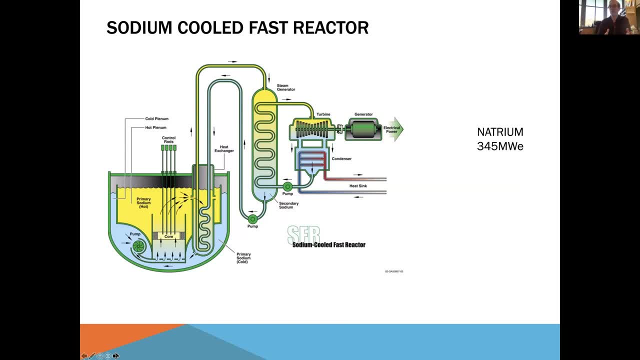 least generate some sort of heat. So if you look at the NETRIM site they say they're about a 350 megawatt plant, right, Not quite as big as a large reactor, but big right And a significant number of jobs for a community, right? So the things that you can do with advanced nuclear at a minimum right for these size plants look similar to what a community can have from a traditional light water reactor. So if you go to the next slide, 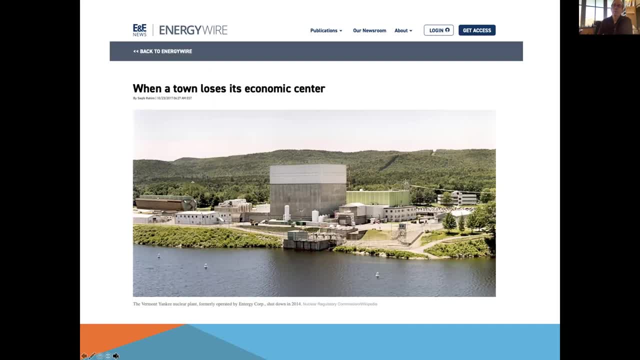 But I think it's important to recognize that in the first generation of plants right, in many cases we built the plant in a fairly remote place and it was great jobs until they went away. And in some cases, these first generation nuclear plants that are shutting down. 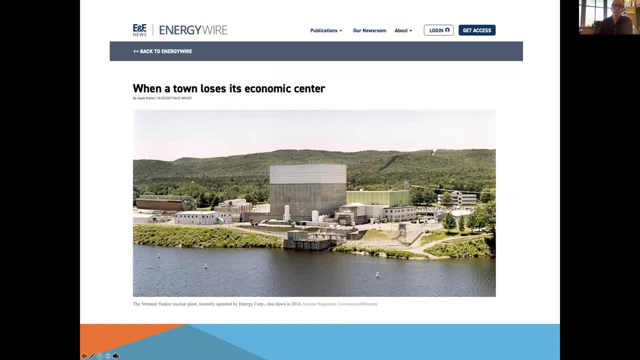 the announcement of the shutdown came very suddenly or unexpectedly to the communities And there wasn't a lot else built up around, right. So this is a major loss of time, Tax revenue, a major loss to sort of the center of a community, And so I think, in looking forward, it's really really important right to think about what else you can do if you're the host of a major energy technology production plant, like a nuclear energy plant. 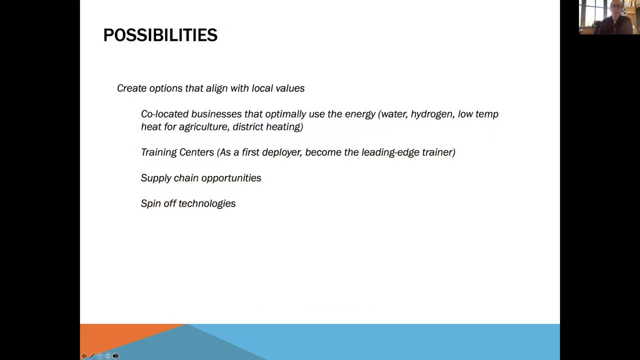 So if you go to the next slide, So I think what's important is to think about other options that align with the local values. right, What can you do and what do you want to be? And these are just some. It's not meant to be. 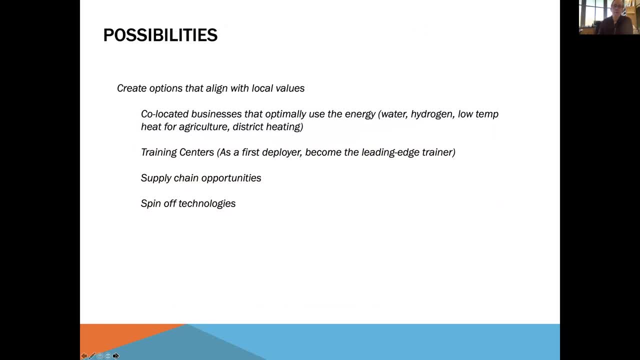 Exhausted, But can you co-locate other businesses that optimally use the energy right? Don't just be an exporter right, Figure out how to do things. make water, make hydrogen use low temperature heat for various local things. 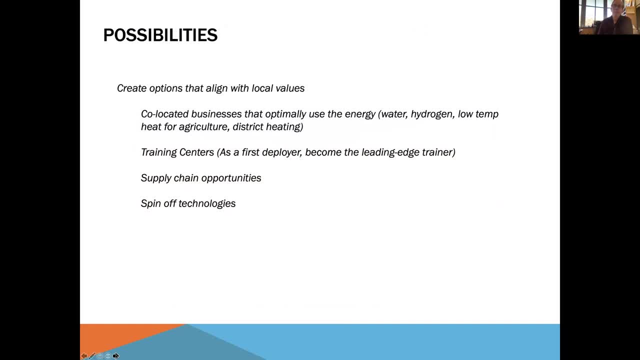 Maybe become a training center, right? If you're the first deployers of a new technology, you suddenly know more about that than anyone, relative to how to build, how to operate, how to get value from a plant, And so people will. 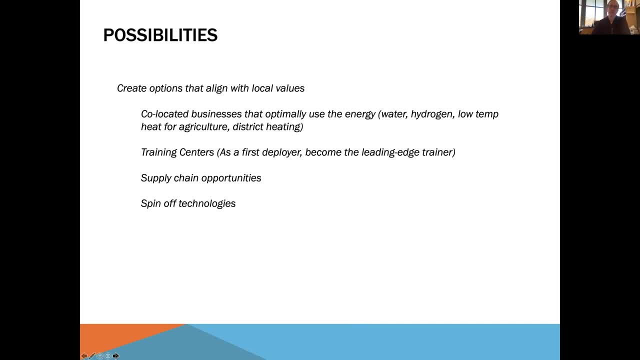 Value that knowledge. Why not take advantage and become a training center? As I mentioned and Steve mentioned, there's supply chain opportunities right in building these plants, especially as version number two and three, and they become deployed internationally right. 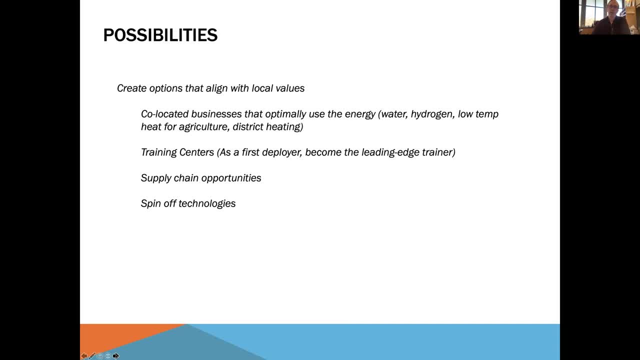 There's business opportunities associated with these plants that are bigger than just the electricity or the energy that you can sell, and there may be spinoff technologies. I'm inspired by the history of nuclear energy in Korea, where they talk about after the Korean War, being a fairly poor society who made what was a very large investment for them to get into nuclear, but the knowledge learned from operating high technology systems they then developed into things like big manufacturing and now, if you look at Korea, they're very good at big manufacturing and other things. 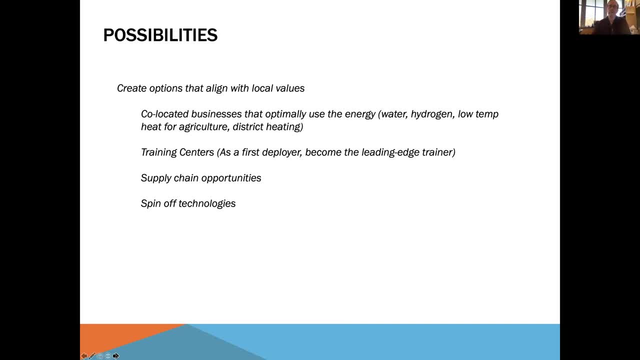 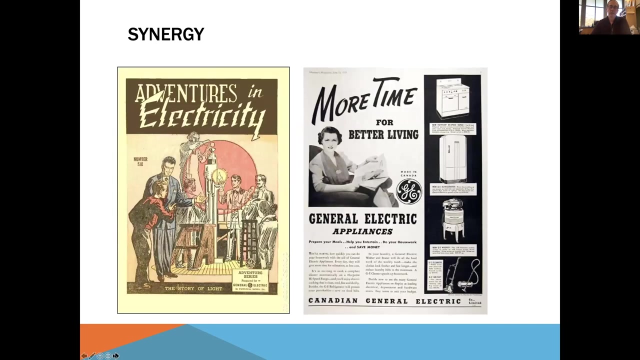 Right, Right, Right, Right, Right, Right. So there's a lot of money that's taken and burning from the manufacturer's auctions and from other thoughts on the technology that they will point back to their history. It started because they made a decision right to build and host nuclear power plants and all the spin off opportunities that came with that, just because you learn more and you've got a highly educated set of employees that you can build on. 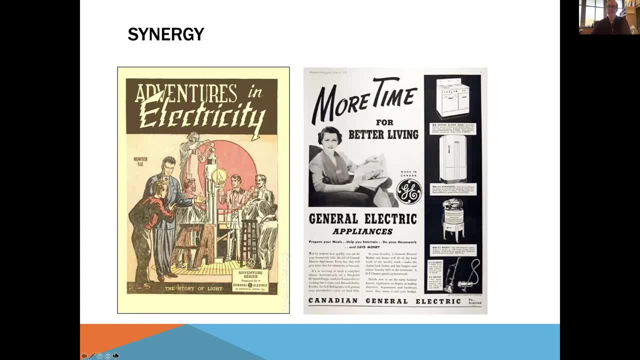 So next one- I think it's my last one, Yup, As inspiration, I'll leave you with these two pictures: Yep, Yep, Yep, Yep. Okay, But you know when General Electric was one of the first big design and builders of first generation nuclear right. so they're selling electricity right. But General Electric also was smart in that they made and sold appliances that used electricity right. 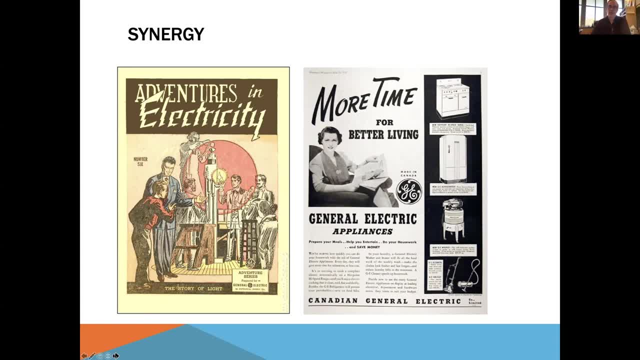 So all sorts of ads about how, with electric stove, electric refrigerator, electric washing machine, electric cleaner, right, your life gets better, right? So think about this synergy between the product that you're making and the use of it, and how to get more value from it. 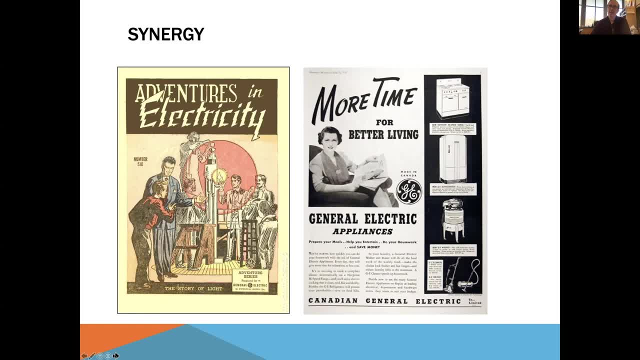 And you know, if you want an inspiration for a system that uses the energy from nuclear more than just selling electricity, I'll go back to my bio. you know where I started my career: on a nuclear submarine, And basically we use that reaction. 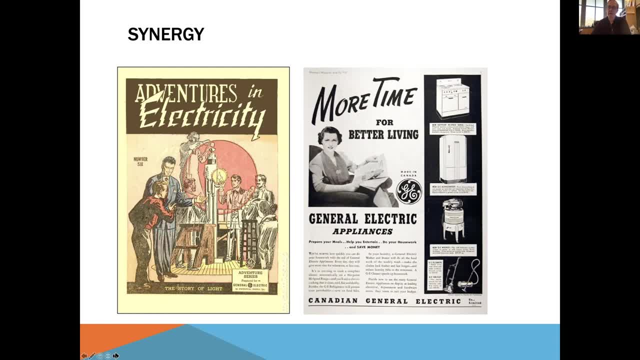 So for everything, it moved the ship through the ocean, it made our electricity, we used it to make water, we heated the sub, we used it for basically every function. we were on board right. So these systems have been demonstrated in very complex ways And I think that's the kind of thinking that people should think about in this next generation of nuclear energy. 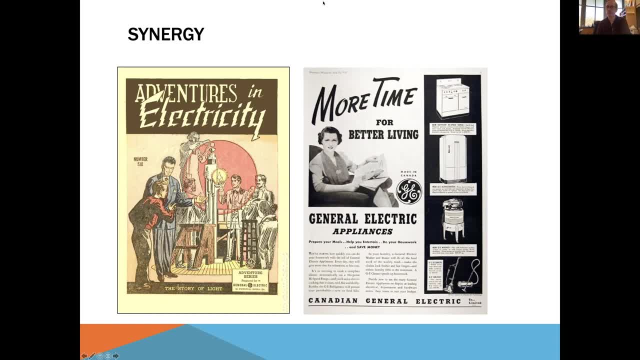 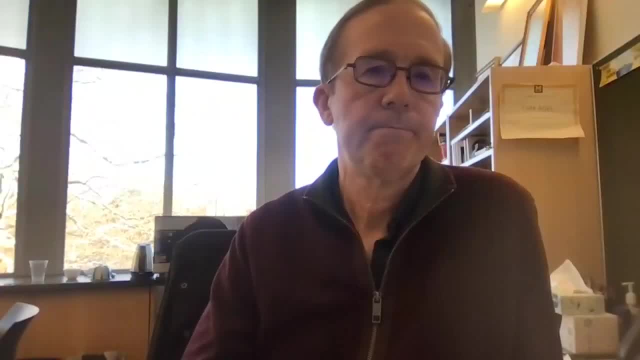 So I'll stop there. I'm looking forward to the conversation with Glenn and Steve and Josh and hopefully answering any questions we can from the audience. Great, thank you, Todd. if we could just stop sharing. yeah, and panelists sort of turn their videos back on, including myself. 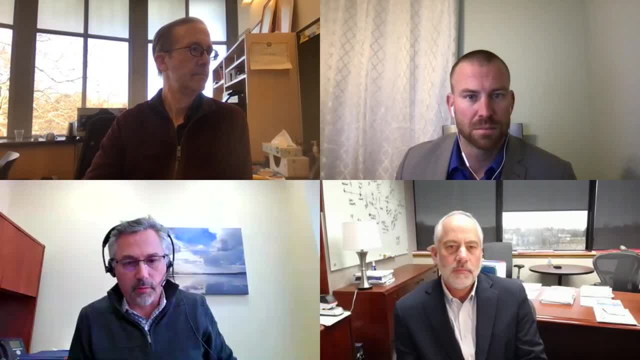 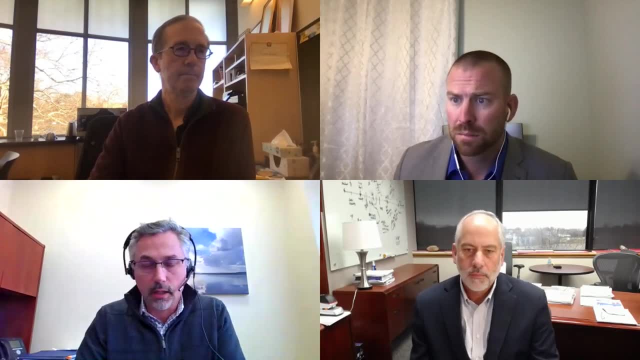 That was a pretty broad session, right. We talked about technology, we talked about fuel cycles and we talked about the industry as a whole. I've got a few questions here, but I'm going to go straight to the participant, the audience questions, because there are a few and there is something quite fresh in our minds already. 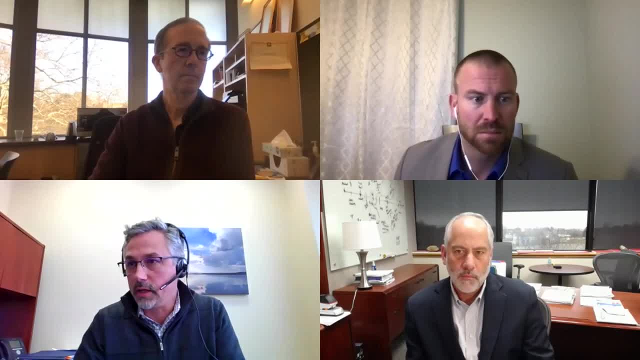 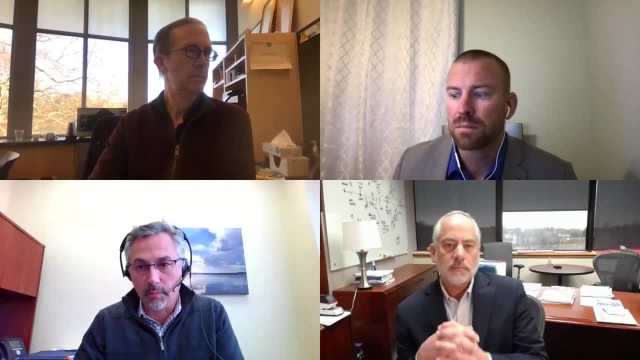 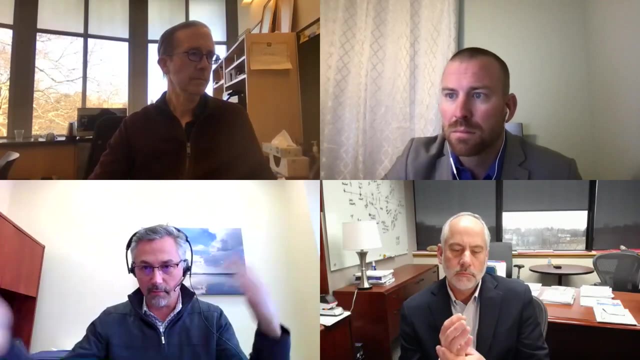 So the first one is- I think it's for you, Josh, but it's from Sina- And it regards the movement towards smaller modular sort of systems and the potential implications of that for treatment of spent fuel. So does that, if you're having a dispersed sort of system right where you have multiple small reactors all over the place, does that imply on-site storage for the spent fuel? 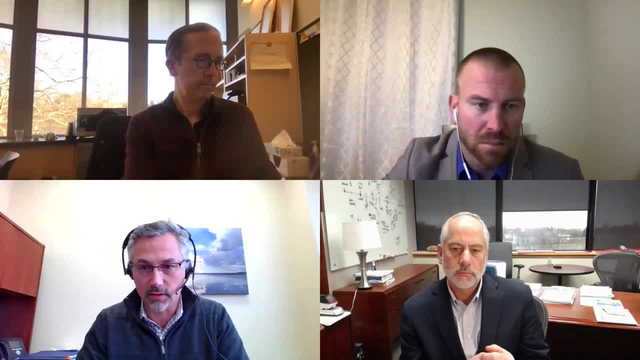 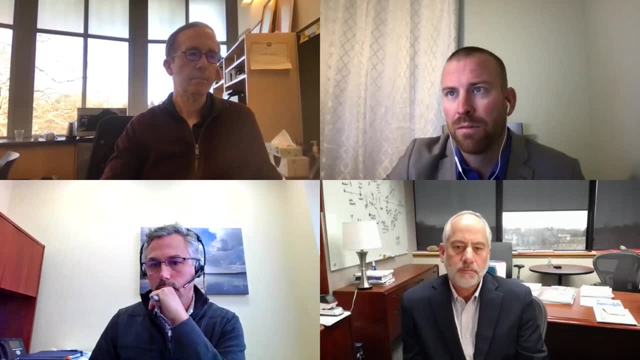 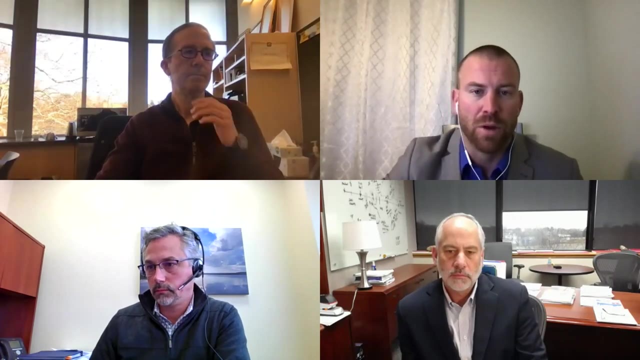 Or is there? how is that going to be managed? Or how would you address the implications of that model? Sure, So I mean I can speak to it. you know, Having looked at what we've done in the past in this country with spent fuel management- and that is we, and I think it's very important to be upfront about this- is we do not have a, you know, a repository solution ready to go right now. 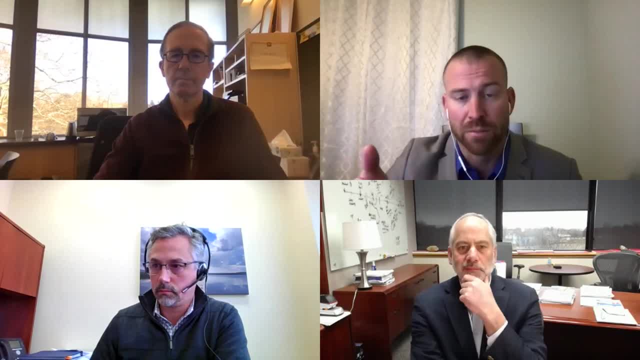 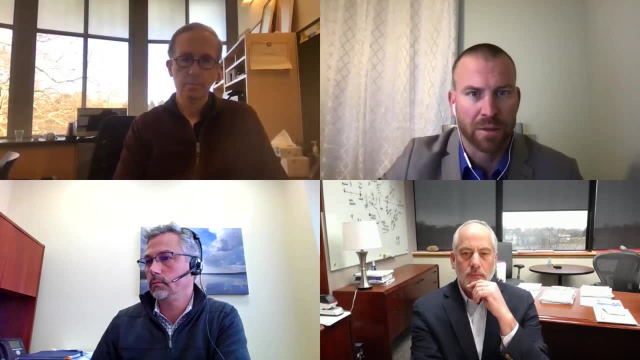 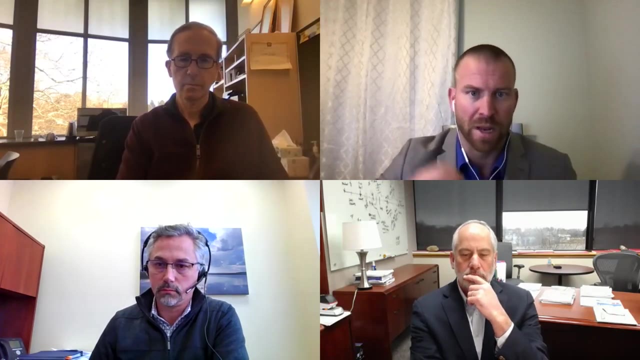 And so I think that any reactor that's being deployed needs to be thinking about how it would manage its spent fuel on its site. I think there are several- I guess I brought up- Consolidated storage facilities that are quote in the works. you know both New Mexico and Texas, as well, as the Department of Energy is looking at opportunities. 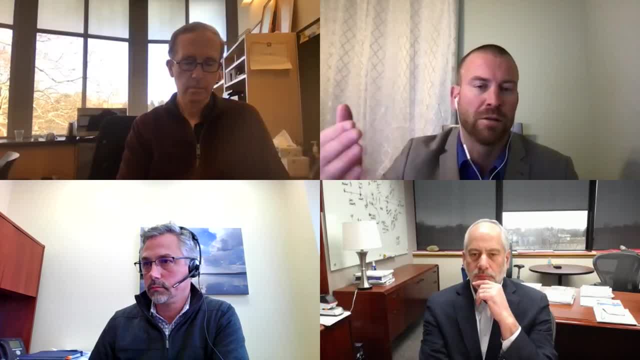 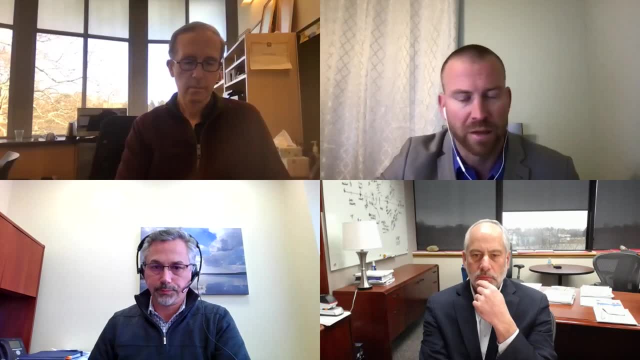 But that's a that's a in the future and there's no guarantee of success for those facilities. We've historically had trouble siting and actually getting these things operational, And so I think that any first off any reactor needs to be able to plan for managing its material, probably on-site. 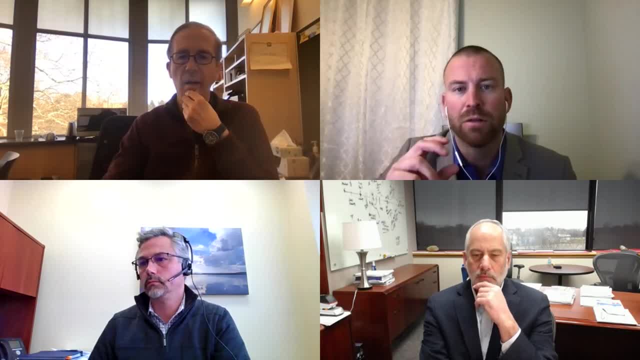 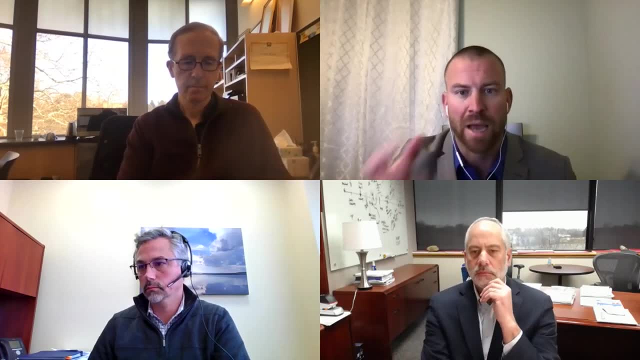 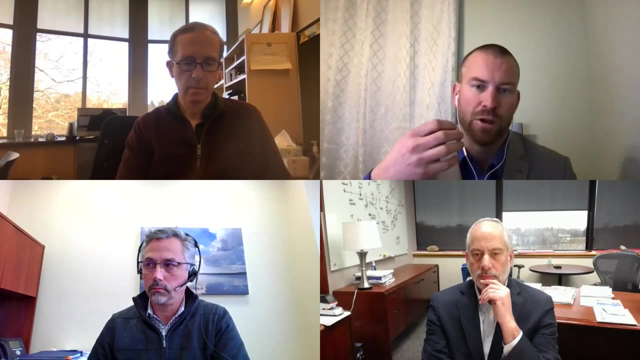 And you know that's the first thing. Now I will say that there are some, some opportunities with that though, too, in that some of the reactors, especially the very small ones, like the micro reactors, those are sort of the nuclear battery you drop, you take them, you drop them in and you bring them back somewhere. 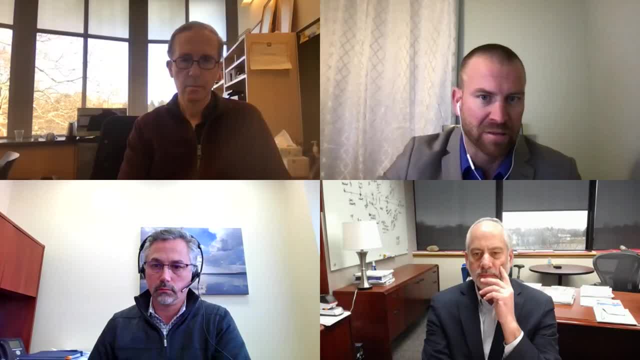 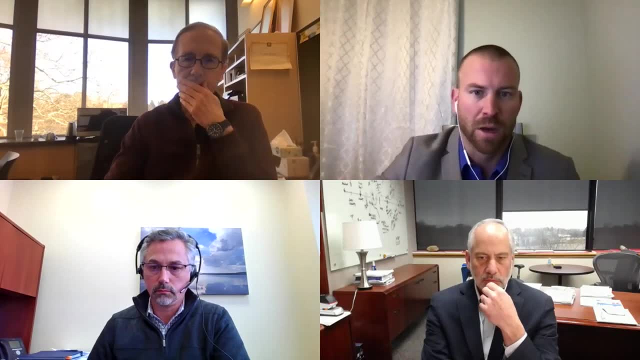 You wouldn't theoretically just leave those where you know on that site, And so you know, if you're the first one into an industry, there's the potential that you could think about a business model where you take, you know, micro reactors back. 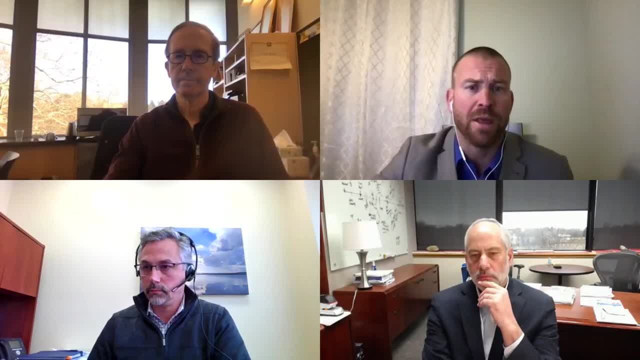 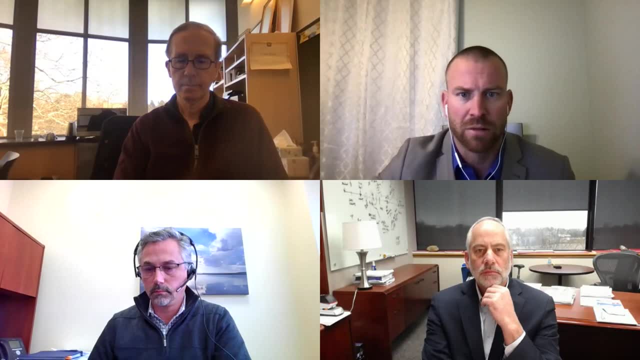 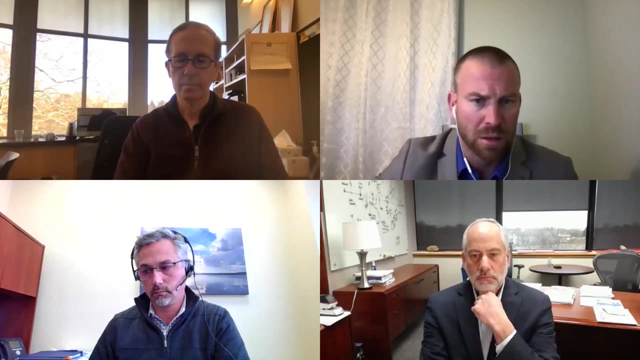 I mean that's definitely in the works, But I think you know, you know to be transparent and truthful- any reactor needs to think about managing its spent fuel on-site. I mean, to be honest, we at INL have spent fuel and have had it here from our, you know, 40 or 52, I can't remember the exact number of reactors. 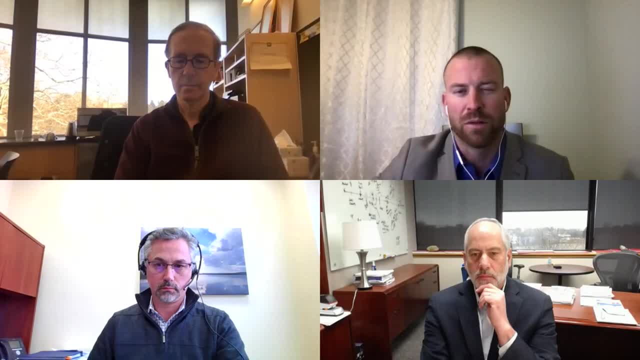 And we've safely managed that material for 50 or 60 years. So it's not really technically challenging, It's not really a you know, We've never had safety issues- but it is something that you have to think and plan for managing that material on your site because there is no confirmed pathway going forward. 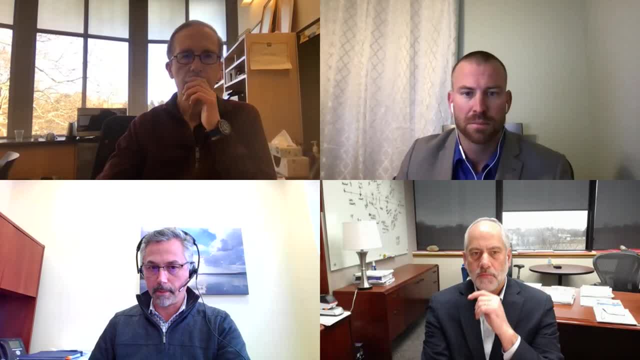 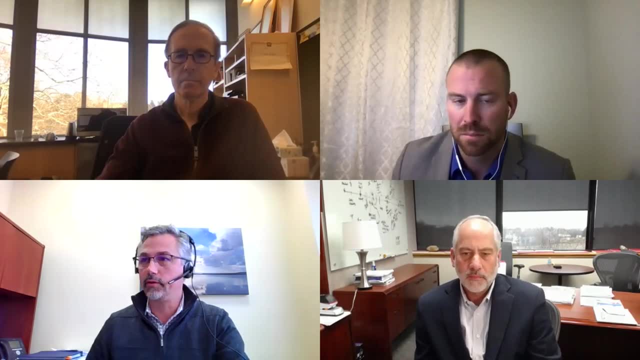 Thanks, Josh. Anybody else have comments to make on that one or we'll move on? Good, Okay, So the next question is from- and I apologize if I mispronounce your name, Louis Luong: what is the progress in developing commercial thorium reactors in the US? 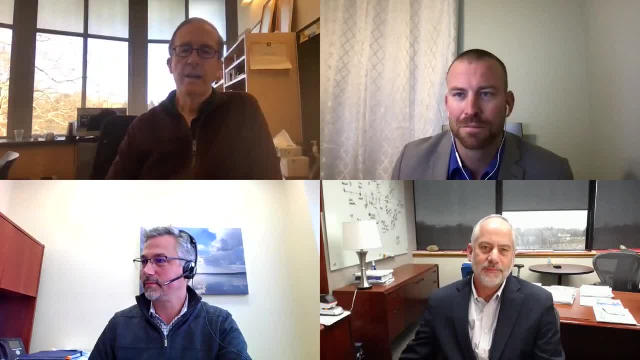 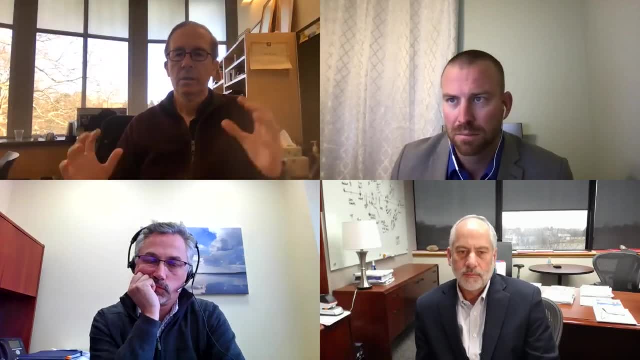 I mean I don't know if this is open to anybody. I'll give it a try, Glenn. I mean I think that if you look across the country there is order of magnitude about 50-ish what I would call private entrepreneurial nuclear engineering companies, privately funded. There are a few of them that are targeting thorium reactors as their product. That said, right now in the US we don't really have a thorium fuel cycle, right? We don't have a commercial way to make fuel from thorium. 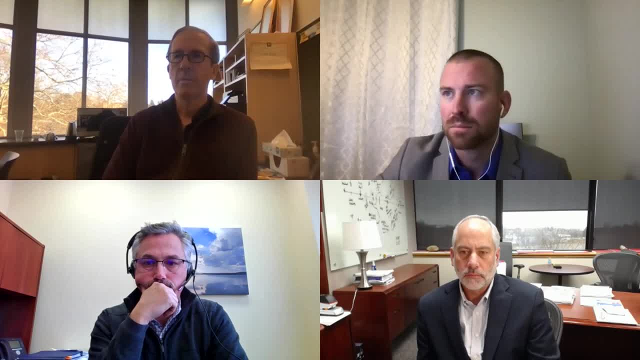 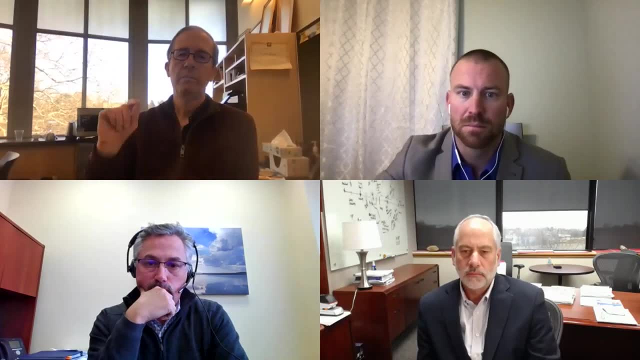 Thorium reactors. So I view these as there is some dedicated effort. The designers are clearly advocates of that. I just think there's a bigger hurdle right in order to get to commercial, because there's just not a history of using those reactors. 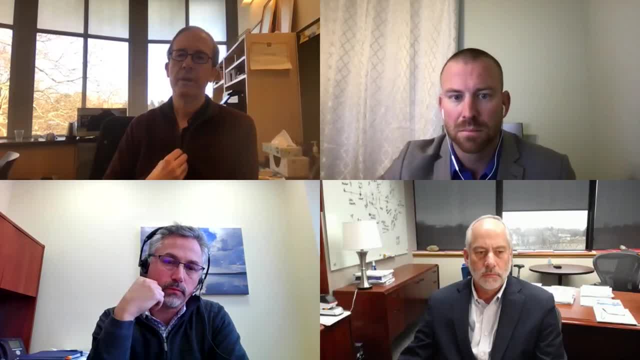 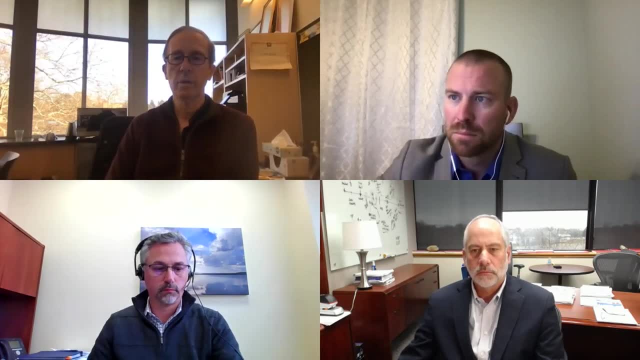 My personal view is: it's not that there is enough advantage to go through all that cost to build up a thorium fuel cycle, But you know it's like all the other companies. Yeah, There are companies that are out there and they'll prove or disprove. you know whether I'm right or not, but I'd call it pretty early in the commercial sense. 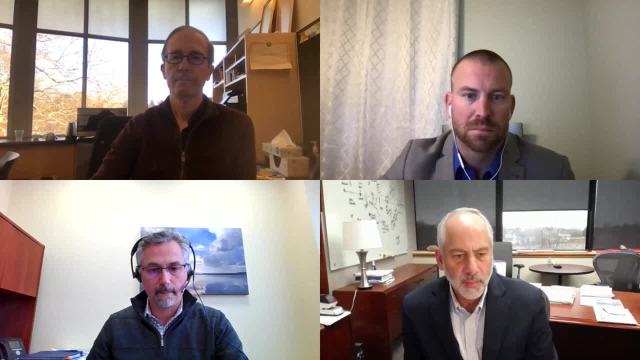 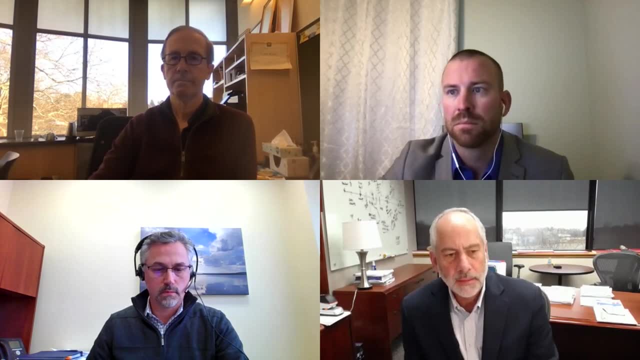 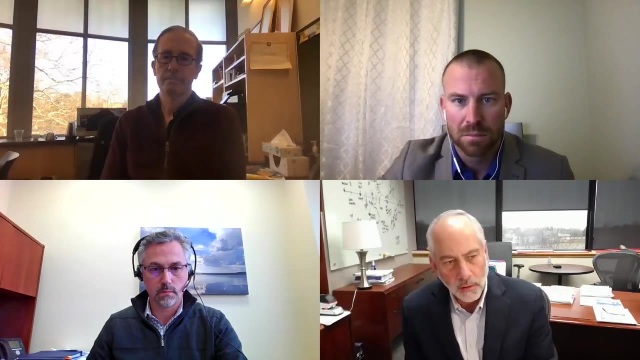 Yeah, Steve, And I just amplify a bit of what Todd said- Not just in the US, but globally- the fuel cycle. there is not a thorium-based fuel cycle, So that provides a great hurdle when you begin to think about. 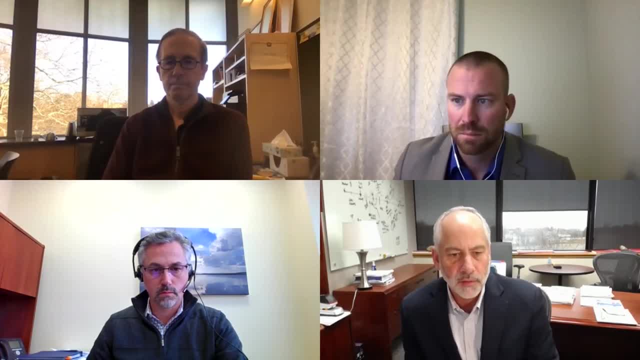 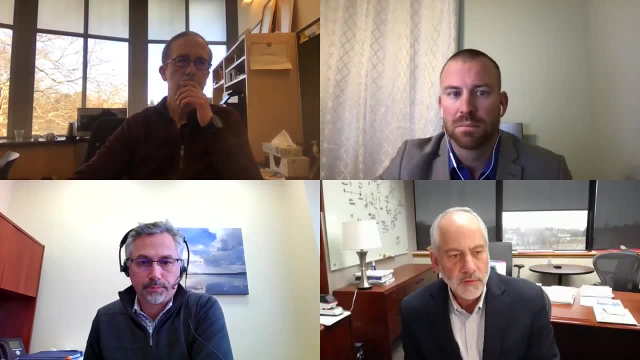 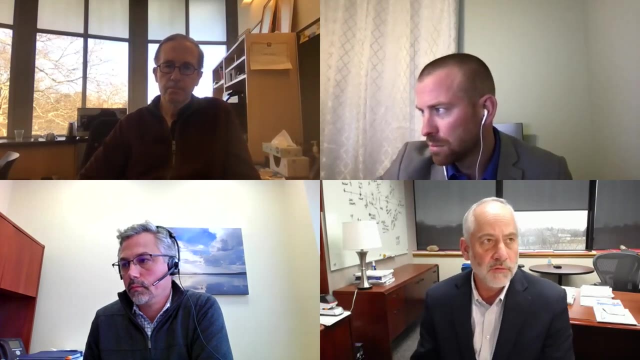 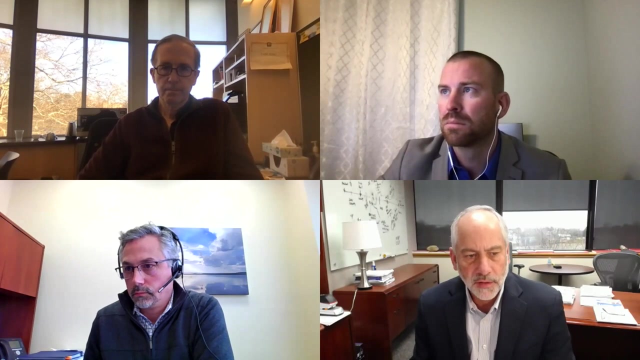 The supply chain leverage that we talked about. So an example of that leverage is- again I'll reference the Korean example that Todd gave. They sold four large reactors. helped construct the reactors just recently, over the past 10 years or so, in the United Arab Emirates. So the total price on those reactors That was about $25 billion. Well, the fuel supply, maintenance and operations contracts that went along with that, in other words helping manage that whole enterprise going forward, was valued at about that same amount, an additional $25 billion. 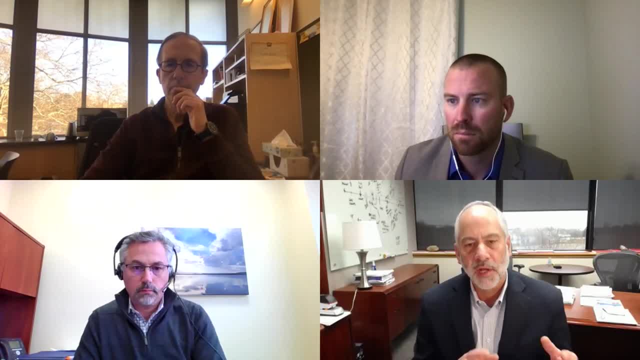 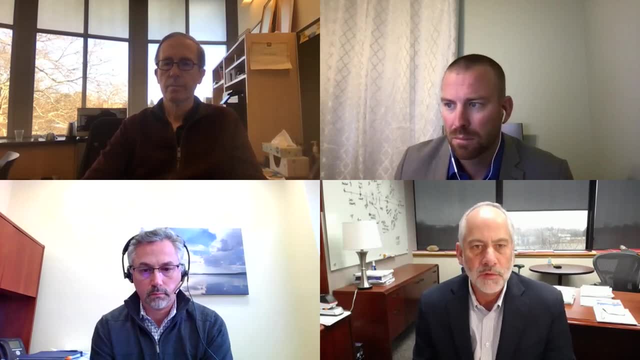 That's an example of you know, it's not just about the fuel cycle in your country, It's about what you can help manage Elsewhere, And that sometimes is where the greater value is. So you know, I think Todd's exactly right. 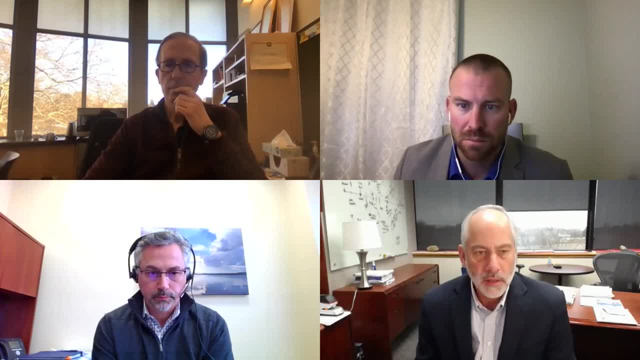 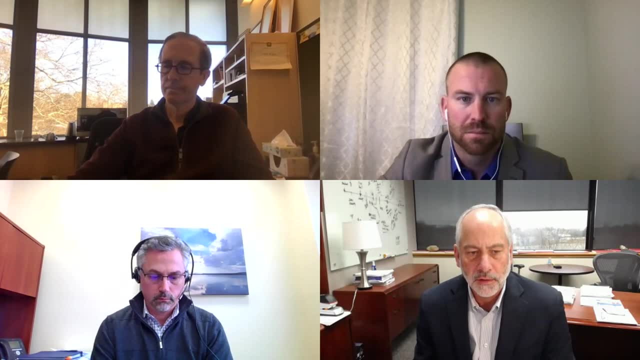 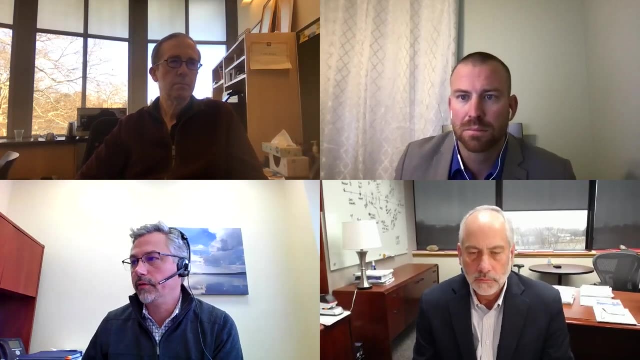 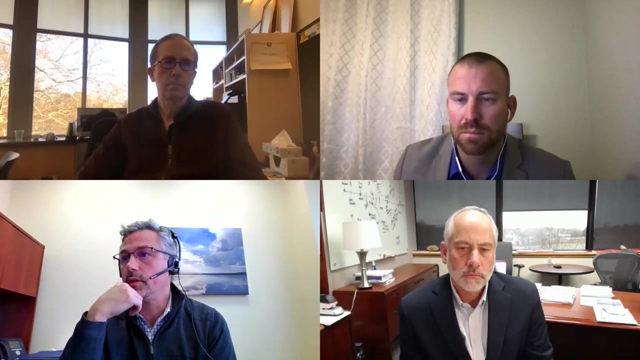 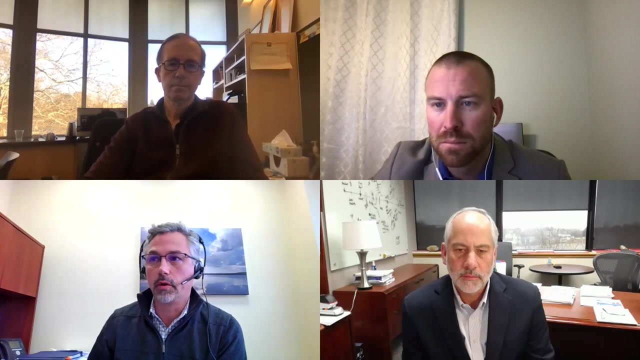 The hurdle in developing another type of fuel cycle. the economic hurdle is certainly significant. Thanks, guys. The next question is from Richard Jones. It's kind of an interesting one because I'm not Educated enough to know what he's referring to here. but it seems to me that much of the resistance to nuclear power, besides a misunderstanding of the technology, stems from problems with historic mining processes that provide fuel. 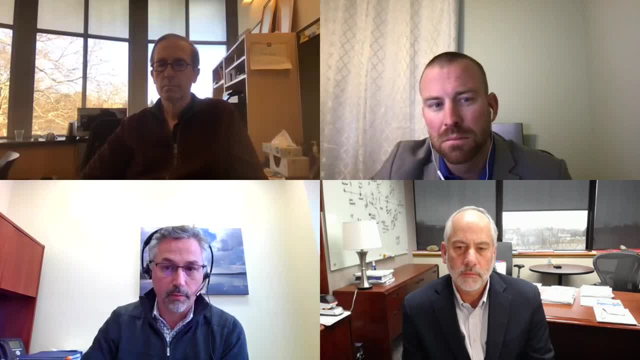 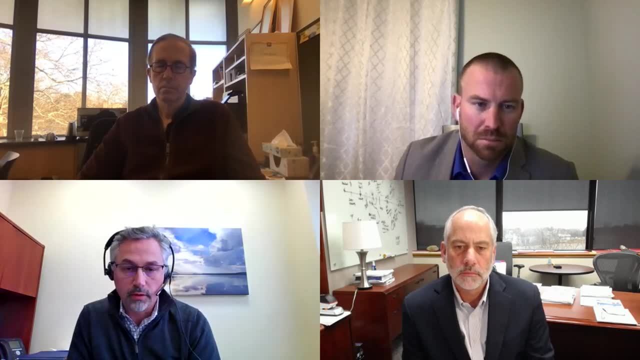 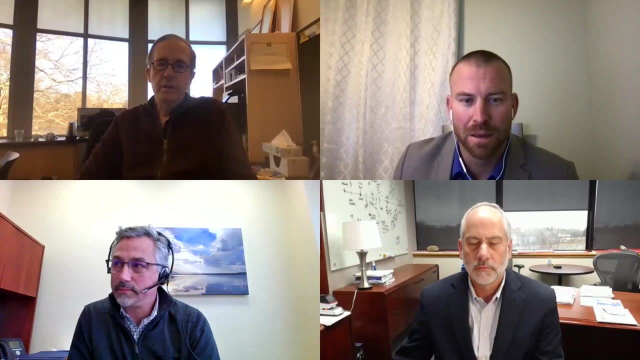 How is this addressed Now? as I said, I was not aware of that, but perhaps somebody take a swing at explaining what those potential problems were historically and if they've advanced Any takers, Well, I'll give you a start and then Josh Josh may have some more details that he wants. 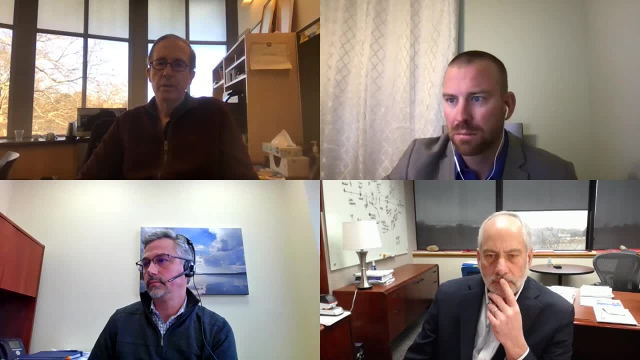 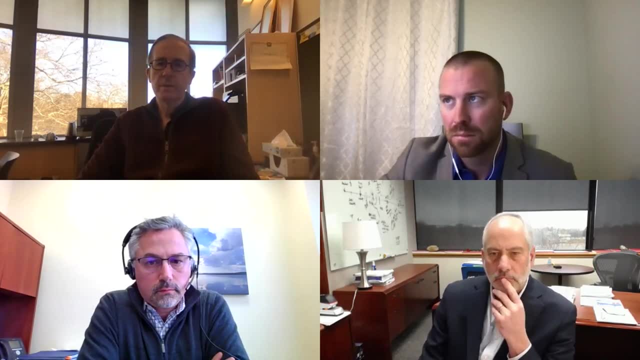 I mean, I think historically the things people point to were in the early days of nuclear right And a lot of these were associated with the weapons programs. but at some point, you know, commercial nuclear diverged from that And I think for most people they don't care where it started. 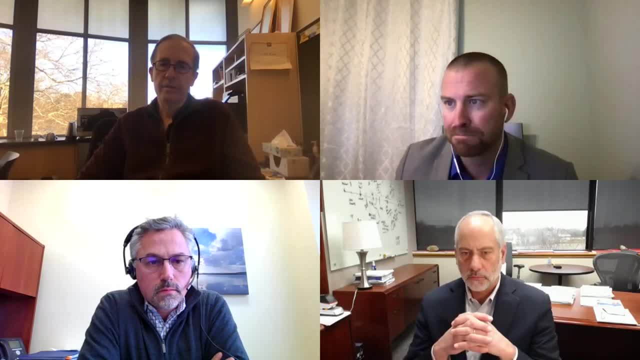 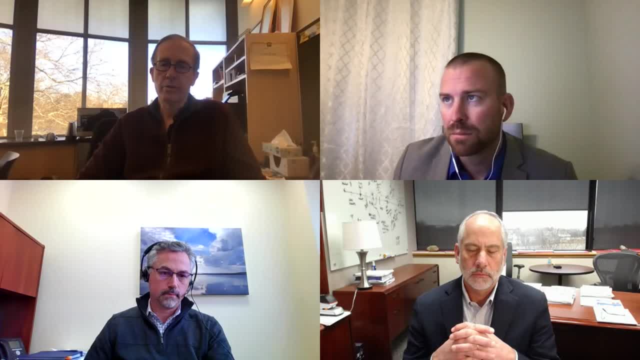 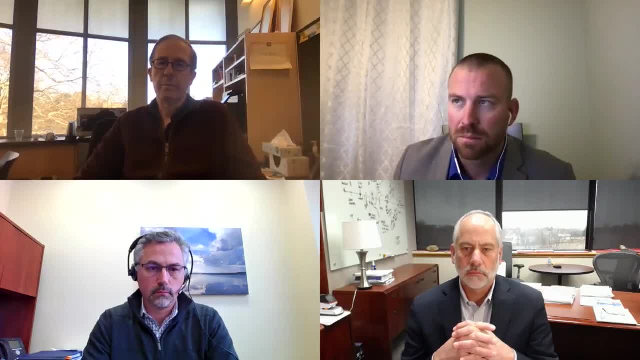 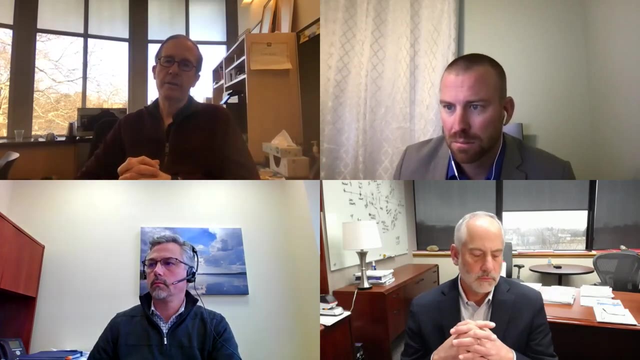 And now we have these very complicated things that need to be cleaned up, right? So So I think some of those decisions to rush in the name of national security left environmental impacts, and the mine tailings is one of them, right, I think, if you look at- and this is where Josh can help me, because he may know more- 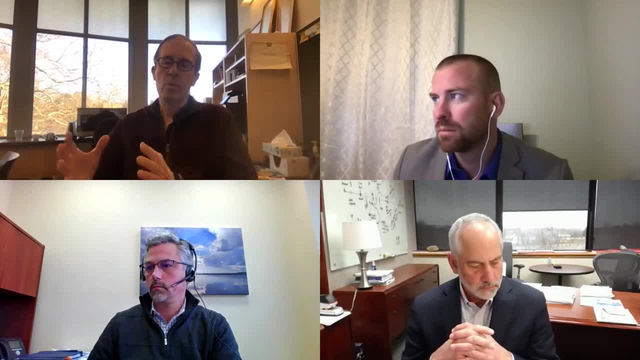 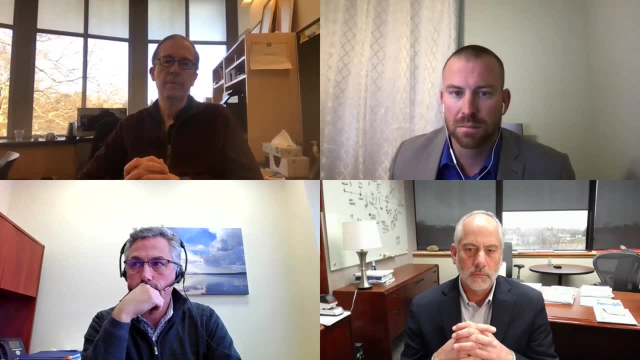 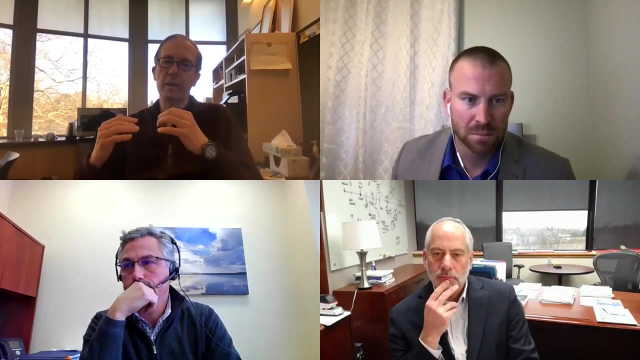 I think if you look at modern mining techniques, they've done a lot more to improve how we do that. That said, I do think until we go back and actually finish remediating some of those sites, there's always going to be this historically accurate concern that we haven't cleaned up. 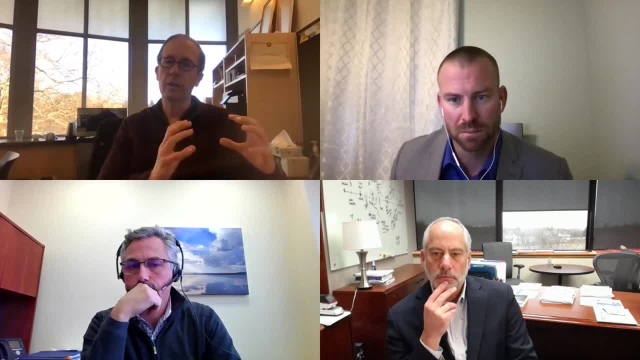 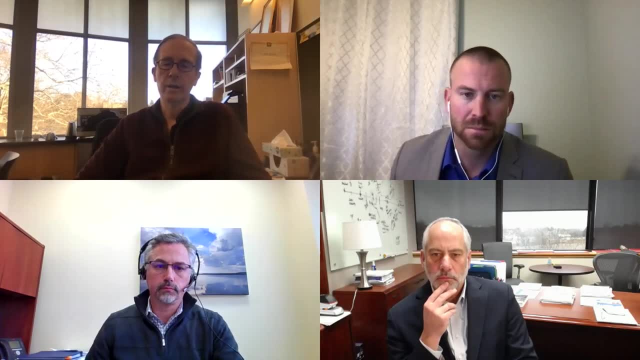 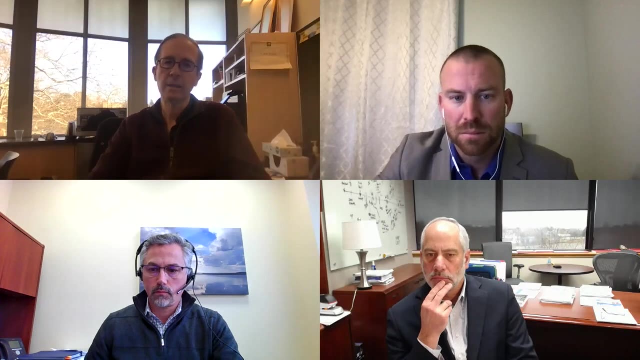 some of the sites and that they're particularly in lower income or disadvantaged communities right, And it makes it appear very unfair or inequitable. So I think that's some of the politics and history behind it. Josh may know more about the transition between mining techniques. 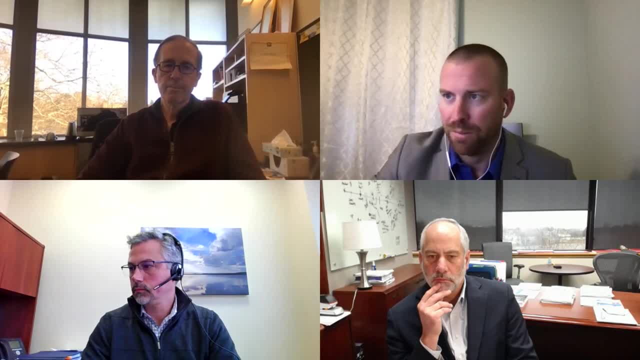 Yeah, I can speak to it a little bit, But I think Todd's probably Dead on. based on the way I read, that question is historically yeah, the weapons program and the way that the US went about the weapons program left lots of environmental issues. 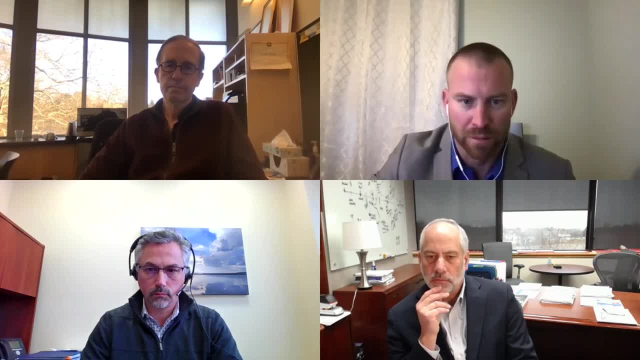 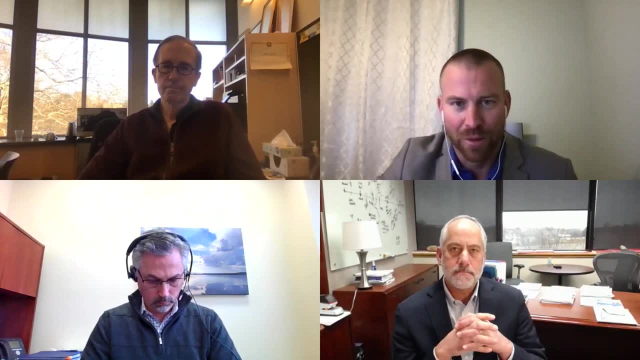 cleanup concerns that we continue to. The federal government continues to struggle with cleaning up and has a several billion dollar a year budget to do some of those cleanups. But again, I think there's always been concerns on how fast and where that goes. 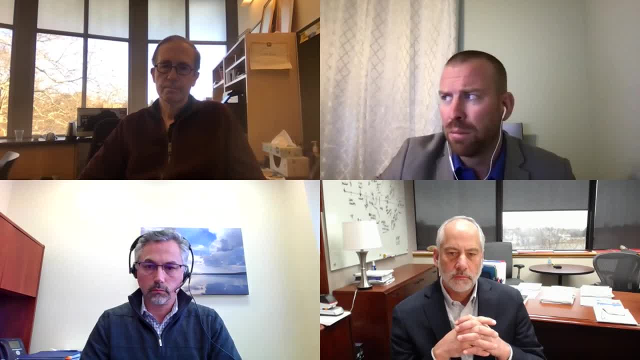 As far as the mining, I think originally I think a lot of it uranium was open pit mining, which I think is it's- maybe not it's maybe- the least clean sort of mining approach. I'm not a mining expert. 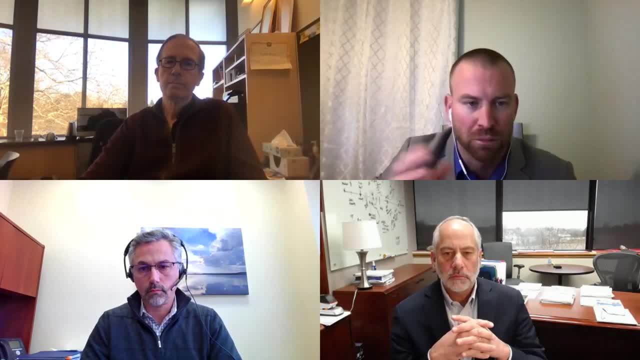 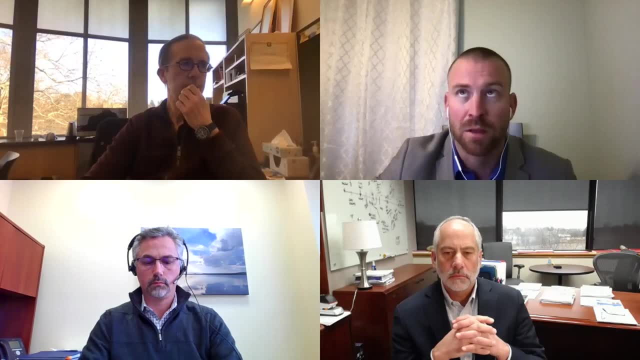 Since then they have shifted more to the sort of in situ leach mining which does minimize some of that. But I think Todd's dead on as far as the historical issues with mining And I think ultimately it's about the supply chain and the whole thing and the 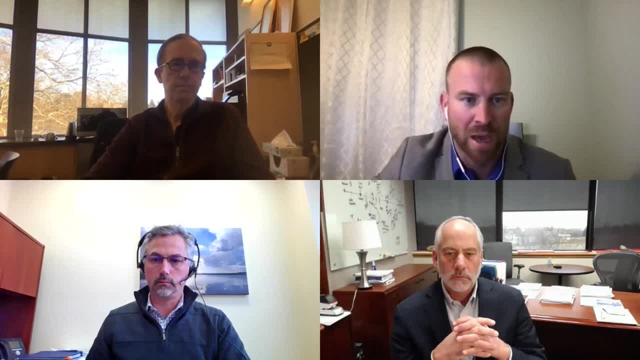 past and the construction and the other side of that, And I think that really has dealt with sort of the byproducts and the restoring the locations back to what they were before. So Right, Got it Okay. So thanks for that. 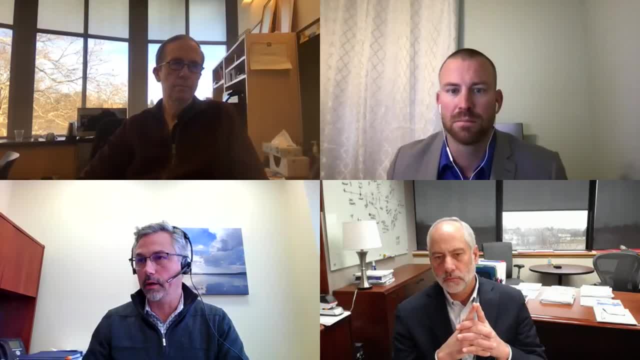 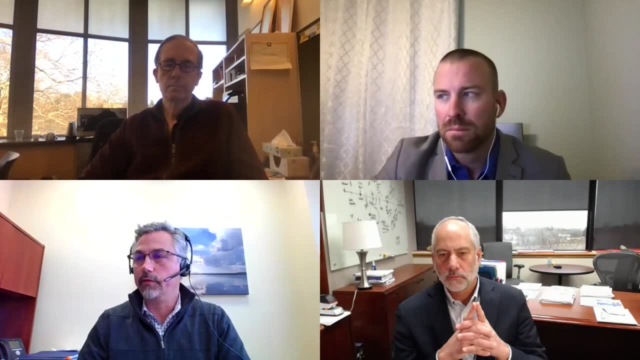 So the next question is: I'm going to combine two questions from our audience and one of my own here. actually It's around the economics of what we're dealing with, the advanced nuclear opportunity, the economics thereof. First question from Thomas Seawald: how will the economics of SMRs or micro reactors ever 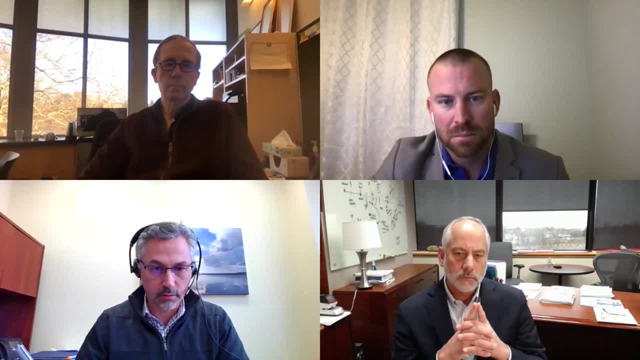 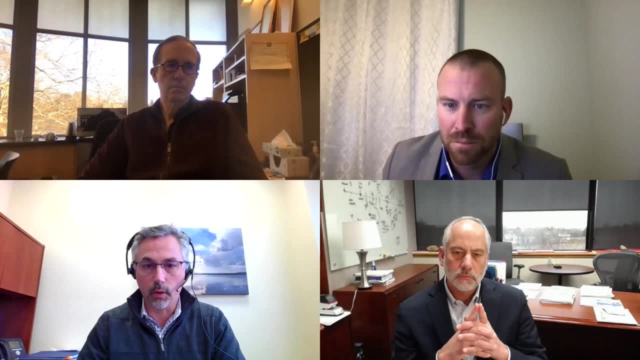 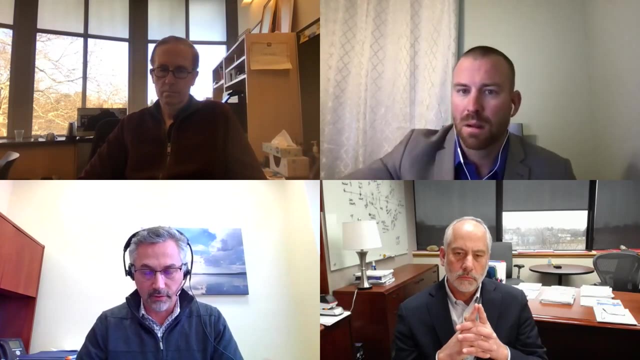 make sense, Not the absence of a standardization. uh, good question. um, mike harman is asking literally what the cost, the production cost per megawatt hour for micro reactors, that sort of question. and, um, my question is simply regarding the competitiveness there is with the thermal. 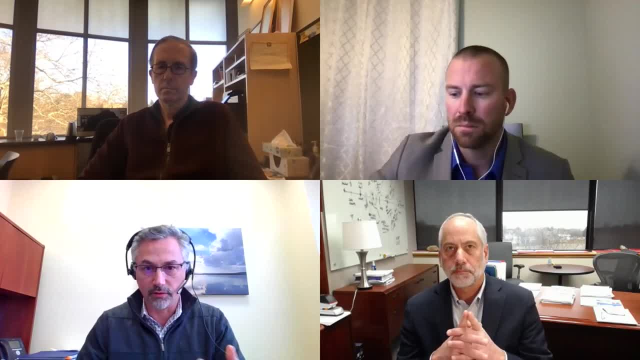 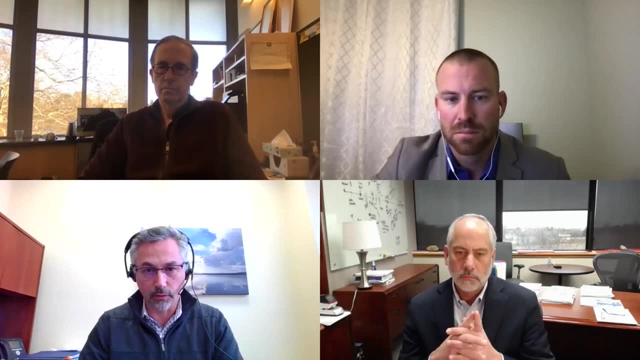 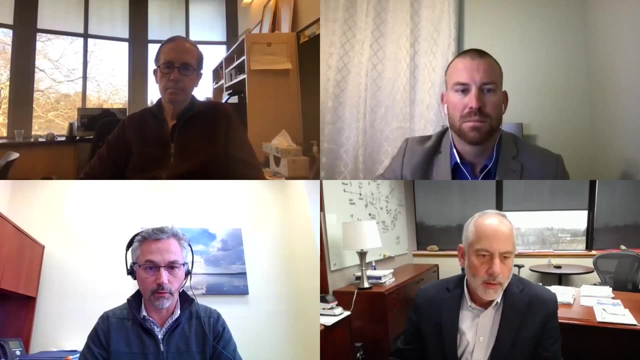 base load of generation, um levelized cost electricity. it's challenging in today's market and today's energy markets for that to be competitive with renewables and so on and so forth. so anybody want to have an open discussion around the, the general economics of these. uh, this opportunity, steve, you're waving your hand, so you first. yeah, so those are those. 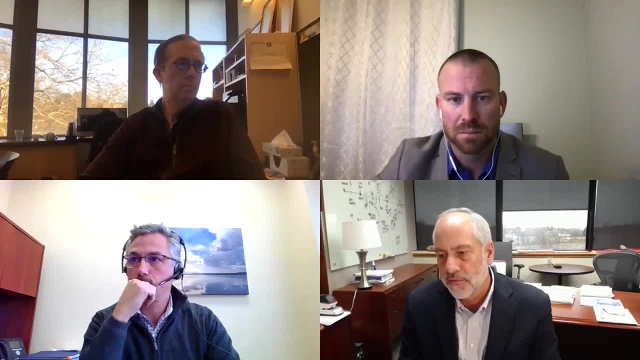 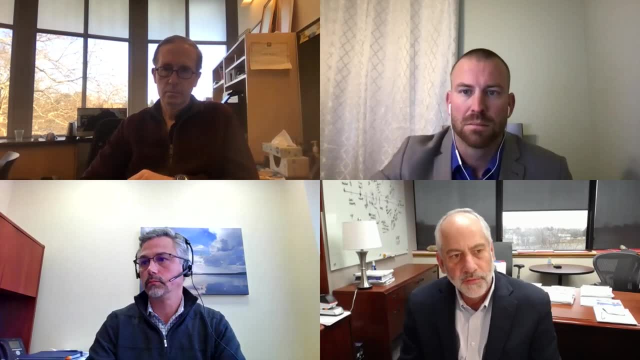 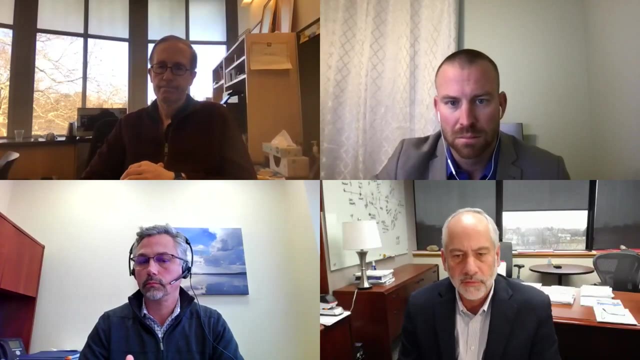 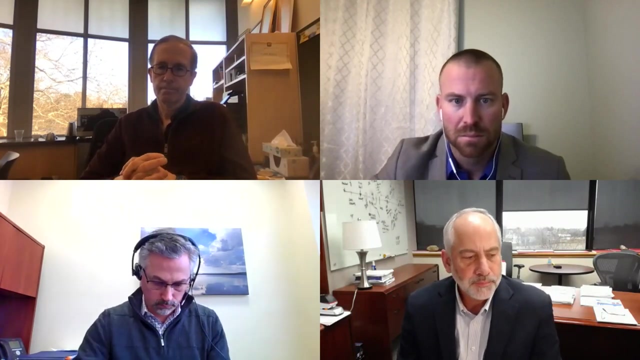 are really good questions and the answers, uh really are varied. so so look to uh todd and uh and josh as well. so so, with very large uh commercial nuclear projects, there's been very good experience in terms of of cost, construction cost, as well as certainly operations cost um and really abysmal uh examples, and that 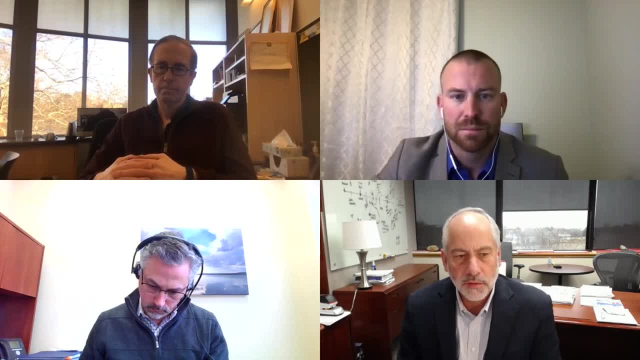 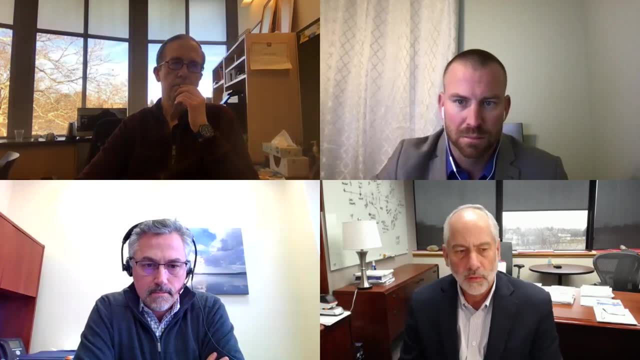 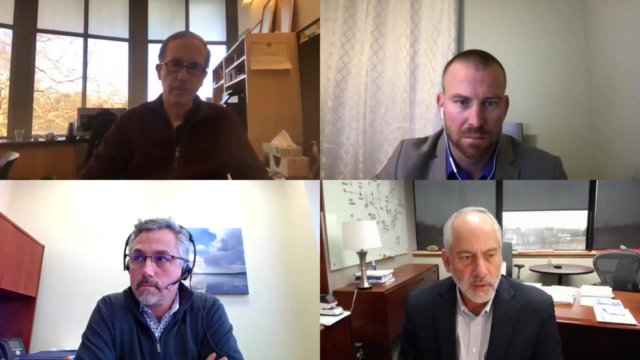 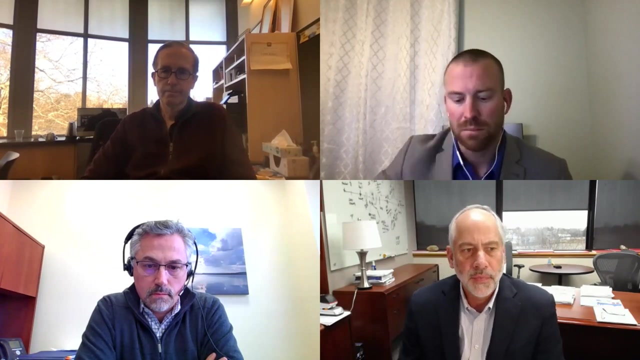 goes for, uh, i think, both the us markets and in global markets. so one can look to, um you know, gross overruns in in constructability schedule which takes uh construction costs from. you know three to four thousand dollars kilowatt installed to. you know, um, the unfortunate examples are, you know ten and twelve thousand. 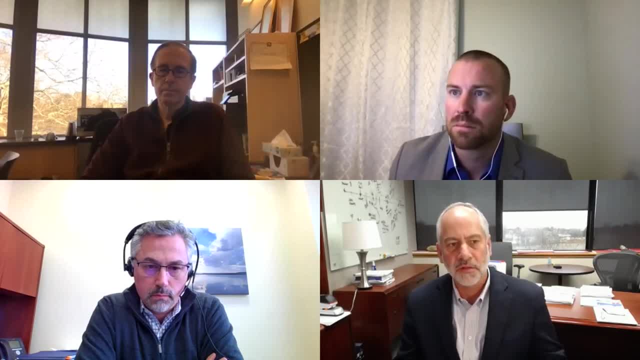 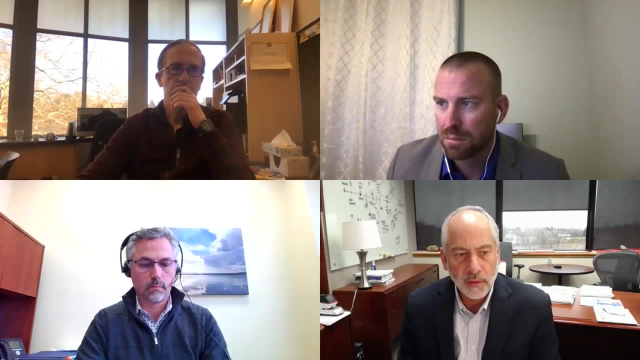 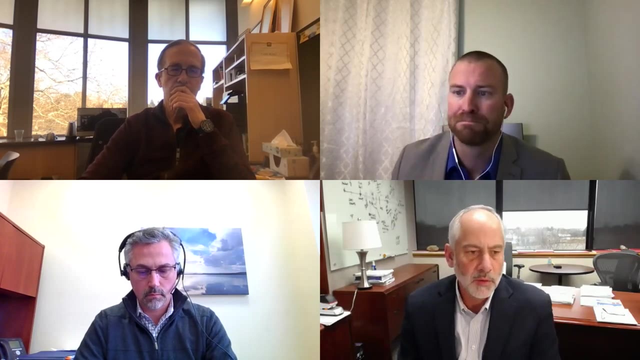 dollars a kilowatt installed. so that's the cost of of constructing something. um. but uh, recent examples: uh, globally you can find bad ones and good ones on the good side. uh, the uae example is is probably one of the more recent uh and that those, those systems come in at. four thousand dollars a kilowatt um, and- and some of the worst ones are examples for the finland example, and of course, the? uh the reactors, uh, the vocal reactors which have gone. i think they're 10 or 11 000 uh projected kilowatt installed. now i'm not sure where they're at. uh, small reactors, uh, since we're not building uh any of those yet, i always look at the cost estimates, constructability cost estimates, with, you know, appropriate uh, hesitation, but but i think the the numbers on those are, you know, 2,500 to 3,500 dollars a kilowatt installed. then you have to. 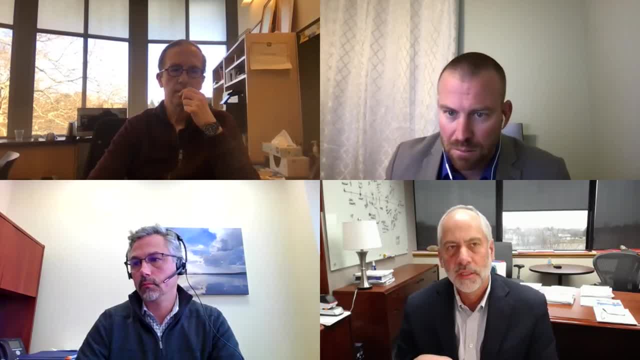 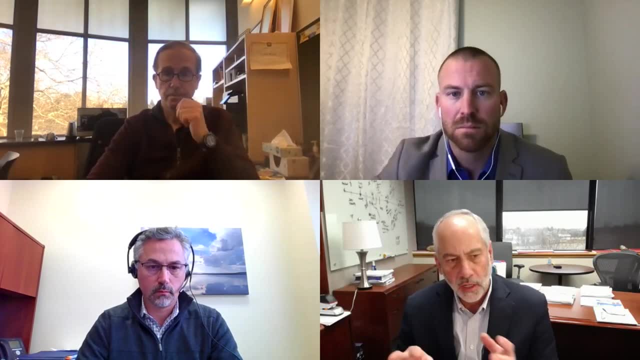 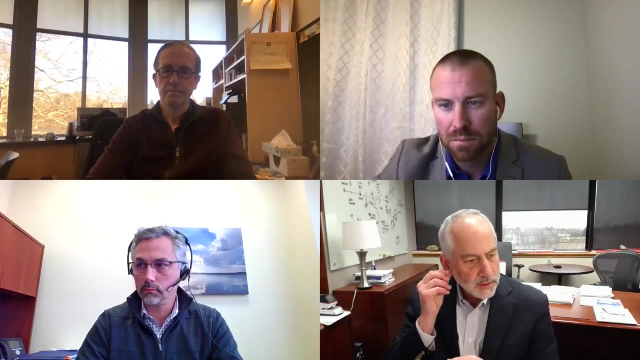 look at it, at the value or the price, um, of the electricity or the heat, uh, that you're getting off those. and so, to channel a bit of my inner Todd Allen, then it really depends on the application space you're looking, uh, you're looking at, so, um, keeping a current nuclear plant operating. um is uh what? maybe 35 dollars. you're selling, uh, you're producing electricity for uh 35 dollars megawatt hour, which is a really competitive uh rate if you look at uh projections, uh for the the future. i've seen projections for advanced nuclear on a dollar per megawatt hour. so the price of electricity, uh, not the heat, everywhere from. you know, on the low side, maybe the 50 dollars, uh. and then i saw one outline estimate: it was like 160 dollars a megawatt hour, but most of the estimates are in the 70 to 90 megawatt hour range and in a in a in a mission constrained world, uh, that looks pretty. 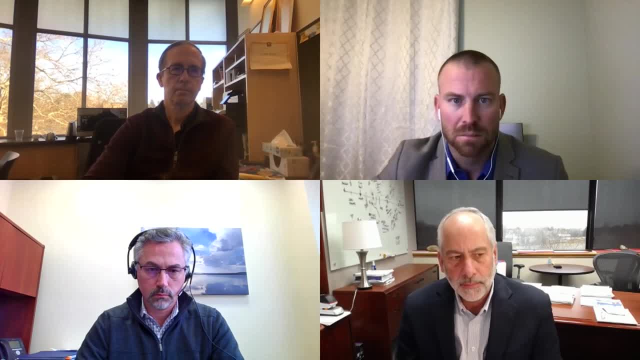 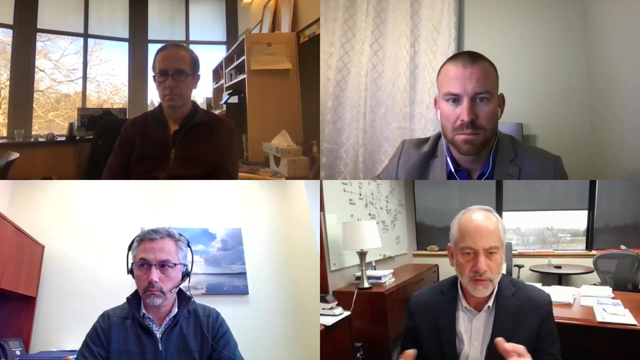 good now. i want to point out, though, that um nuclear produced heat or on-site electricity uh in certain markets. uh, some of the better analyses that have been done for use of heat and power in constrained markets, like in Alaska, actually show nuclear, uh advanced nuclear, coming out far, uh far in advance, far better than any other available option. um, and then, when you start, 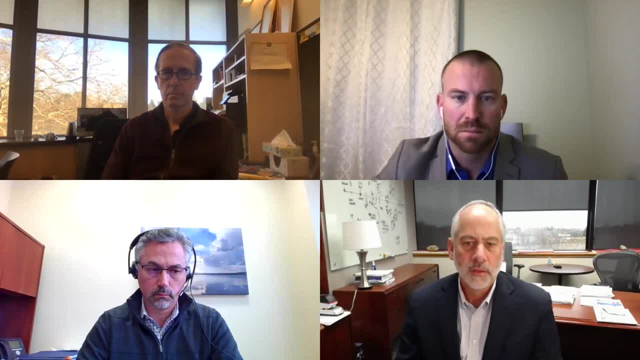 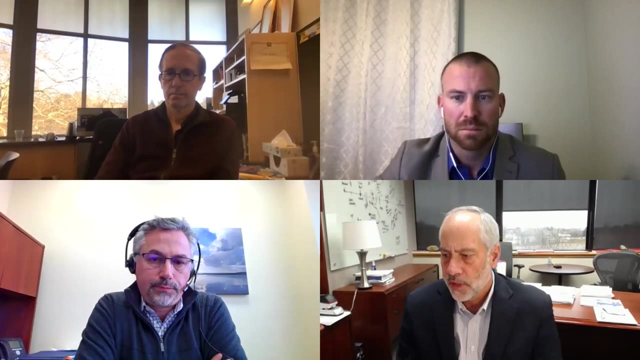 uh, looking at what kind of products you could make with a a high density, zero carbon energy source, the value of the products can go up quite a bit. and in one example i'll give you just because i was reading about it this morning, uh is the analysis that's been done on on green steel. you know low, low emission steel products where, uh, even 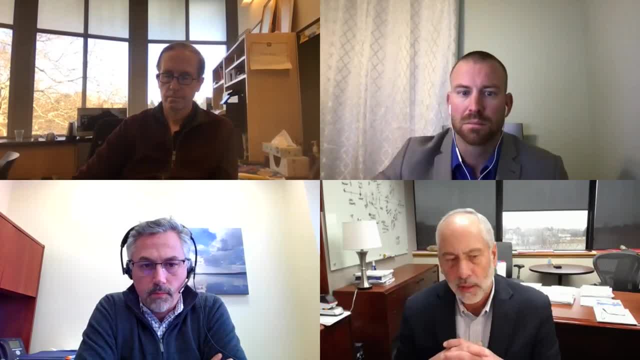 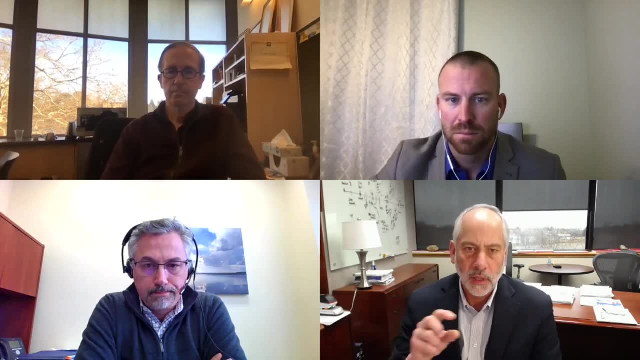 absent any sort of emission mandate. um uh buyers are willing to pay a 25 premium for a low emission tag that goes on that product. so that's a very long answer to a very simple question. but it goes back to your question about uh production. you know what you want to do with the energy where you're. 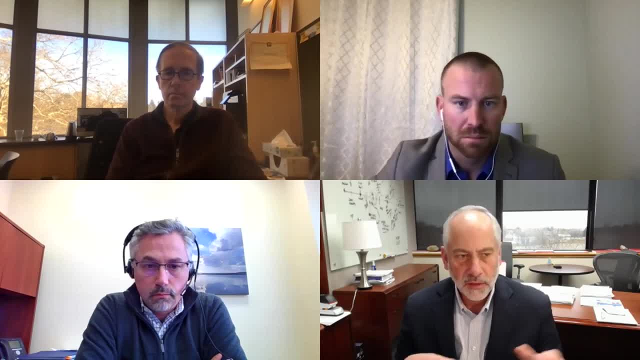 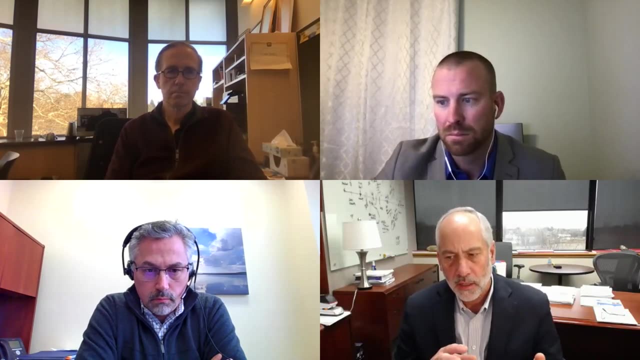 at and what kind of market we're in uh in the future. so does it look uh? does it look uh onerous? no, i think, and i'm a. i'm a skeptic, uh by heart, but but actually the the analyses that i see recently on on the potential value or the cost of producing energy, heat or electricity, uh is. 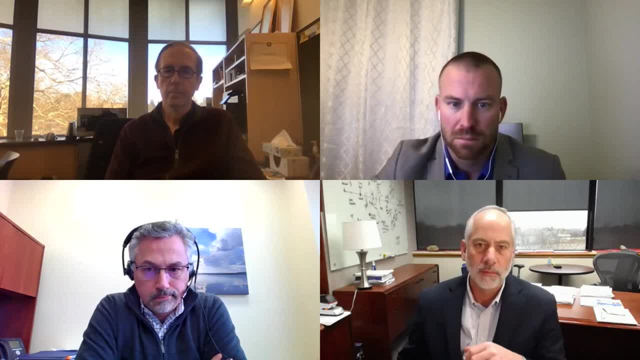 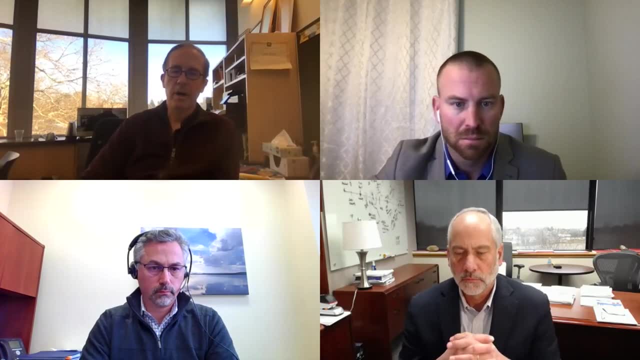 better and better for nuclear. So I mean, Todd, what do you think? Yeah, I think that's a good answer. The other thing that I chime in, but the other part of Tom's question, was: how are you ever gonna drive down the cost? 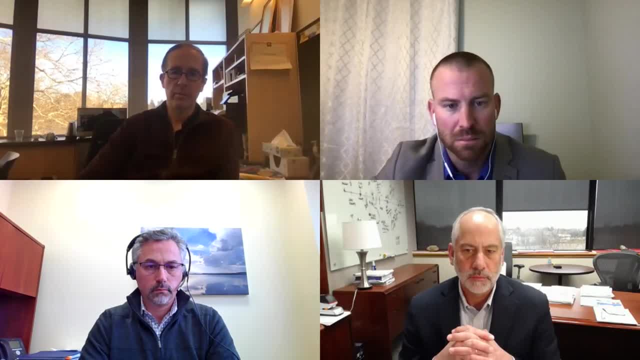 through manufacturing efficiencies, unless you get to a smaller number of products. I think that's right. I think you do need to get to a smaller number of products, but I'm personally willing to be a little patient, right? I'm nervous about the nuclear community. 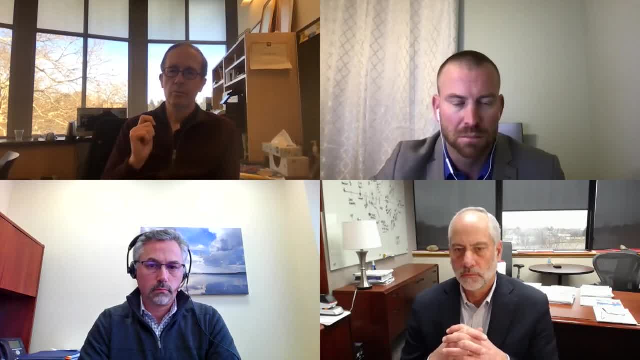 or the federal system who's providing support, rushing to pick the concept they think is the one that's gonna be the best right? I kind of like this: let them duke it out right And set up federal support systems that are milestone-based right. 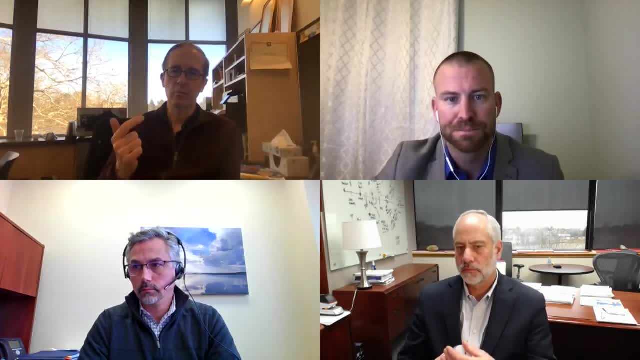 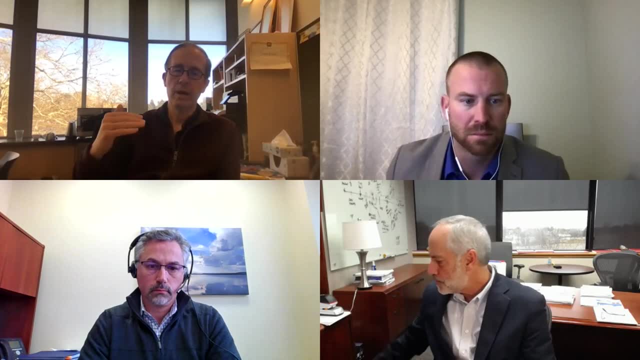 And if a company can't meet the milestones, and whether that's technical, regulatory community support, then you drop off right And let somebody else move up right, So you end up with sort of the best product, right, And then let them drive the costs down. 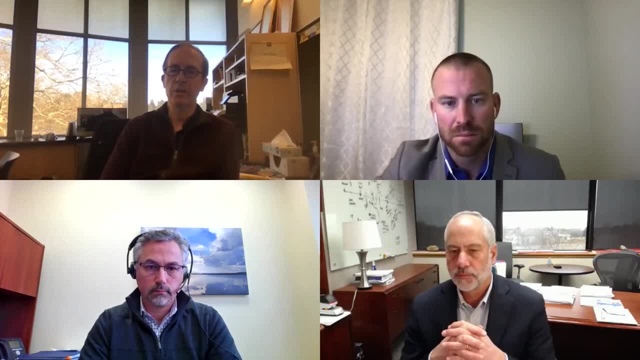 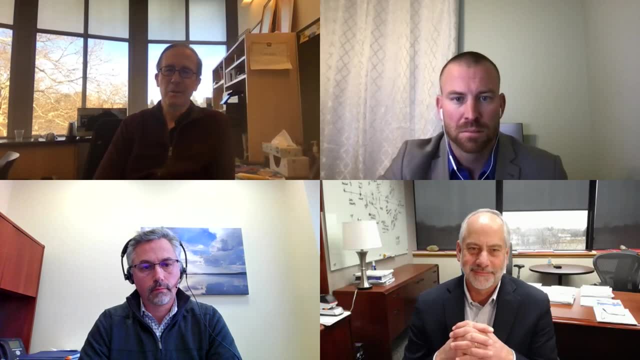 But I just suspect, given on past performance, if we get nervous and we jump and ask a bunch of federal technicians right to pick the one they like, we won't get the best answer right. So there's sort of some strategic patience. 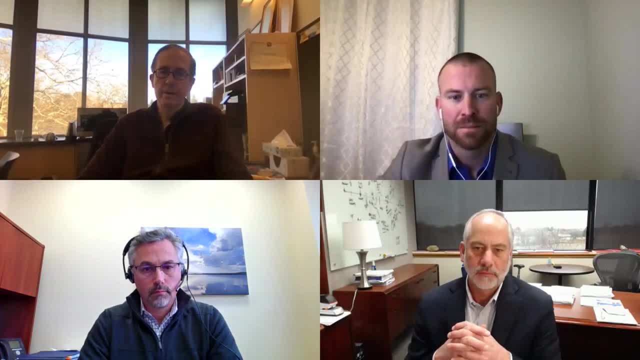 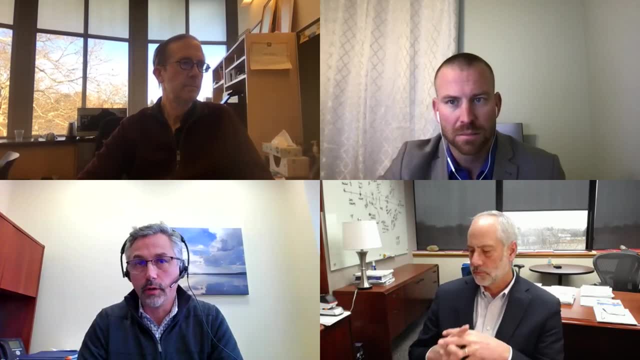 in letting them get to the best product. I think it's really important. Yeah, yeah, good point. Next question- and I apologize if anybody who's submitted a question we don't get a chance to answer it- I'm trying to pick the ones that cover the most ground. 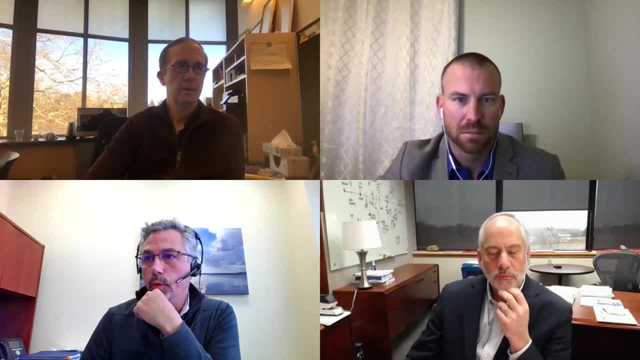 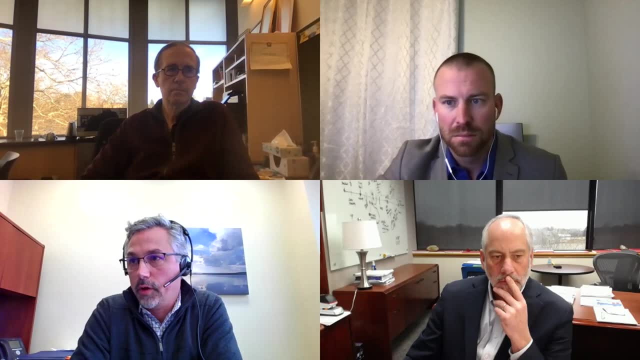 So the next question is about licensing, And Larry Wolf has a question here. Do small and micro reactors require NRC licensing? How long does that process take? Has the sodium design been approved by NRC? And I'll add, you know, many comments that I've received. 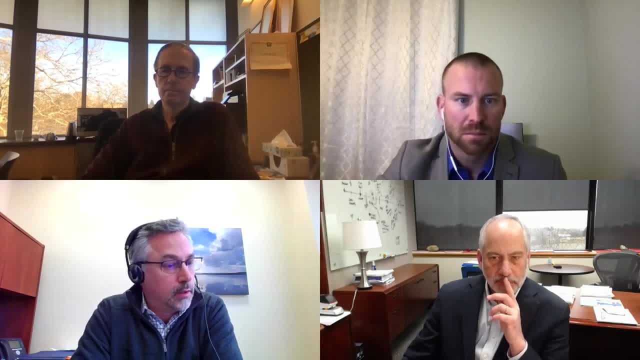 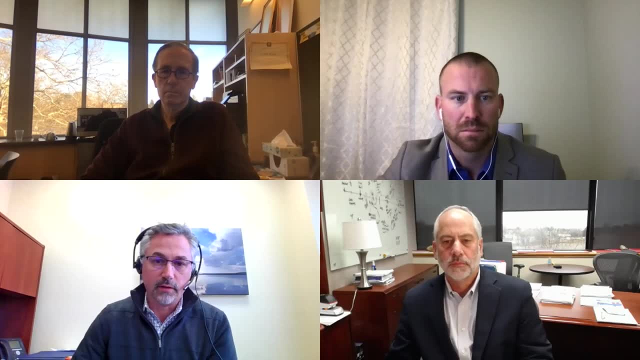 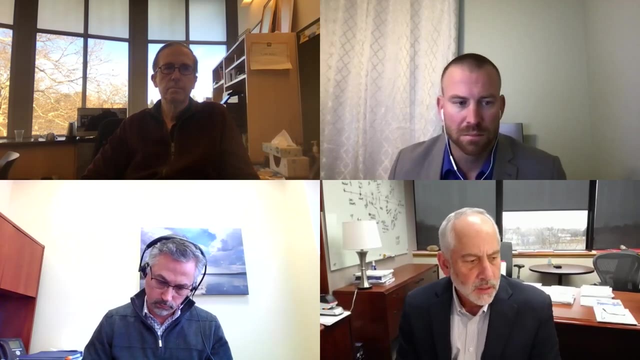 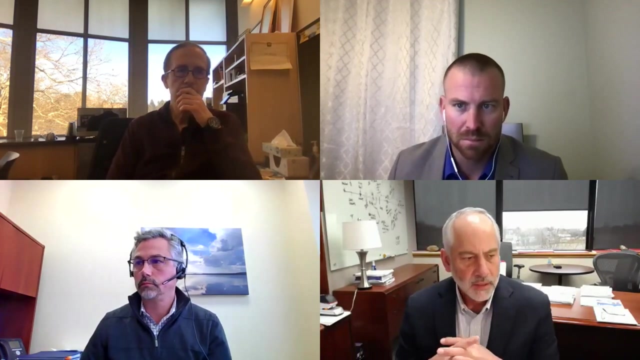 over the last few months regard to the, let's say, challenging timeline associated with terapower and atrium and any commentary around the licensing aspects of these reactors. Yeah, so maybe one brief reply. So the challenging nature of the atrium licensing timeline. 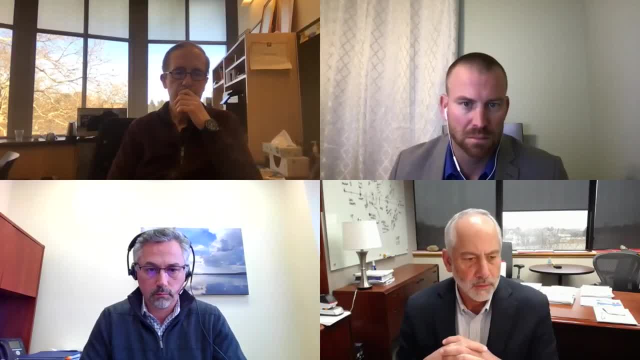 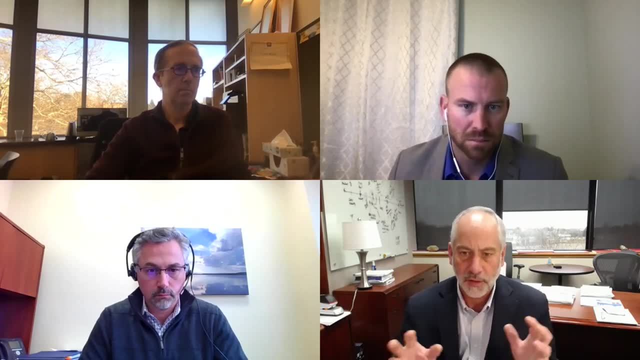 you know I don't pretend to speak for the project, I'm not a part of the project. I'll just you know, I echo the project developer statement that, yes, it is an aggressive, very aggressive timeline. I think what's important, yes, the NRC, you know. 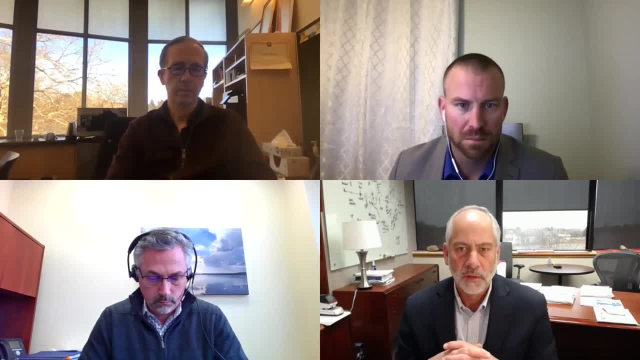 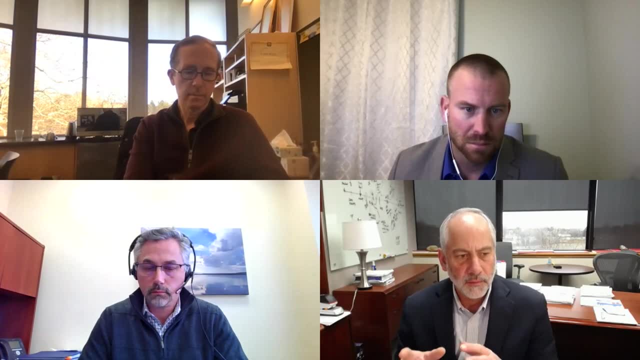 NRC does have to license any of those, any of those reactors, to one part of your question. But the what I would encourage people to look at is the record. what has been licensed, how long did it take? So developers, can you know? take one of. 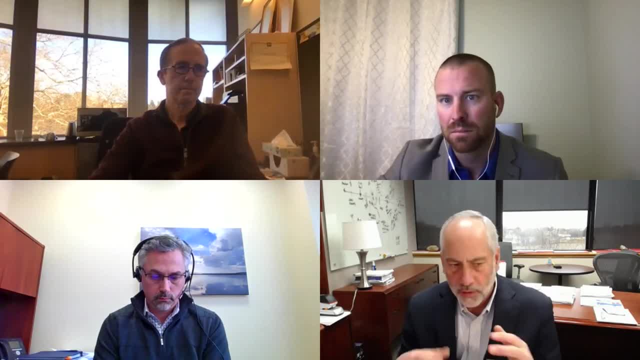 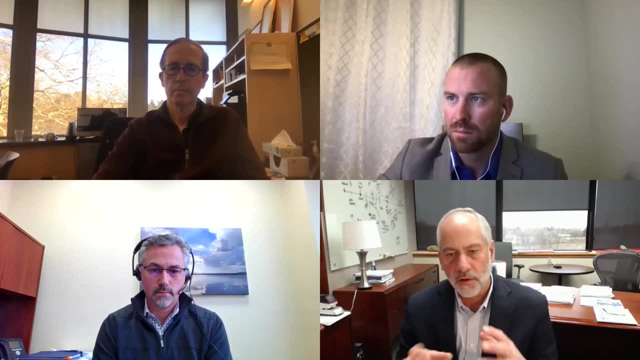 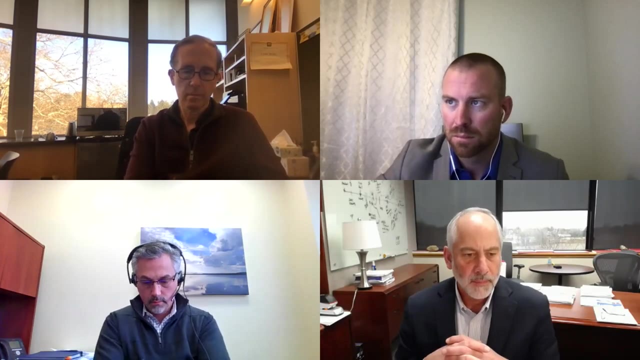 one of two different licensing approaches. You know you'll hear people talk about part 50 and part 55.. part 52, licensing um, which actually starts with the design certification in part 52, if you're, if you're going down down that route. the history then is: if you look at the new scale, the small. 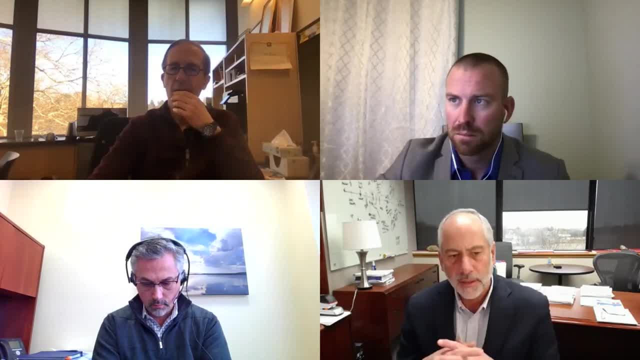 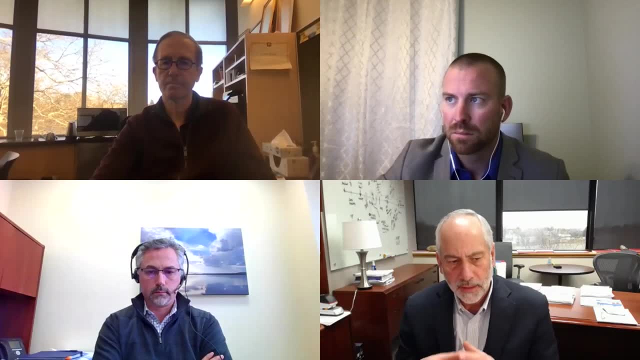 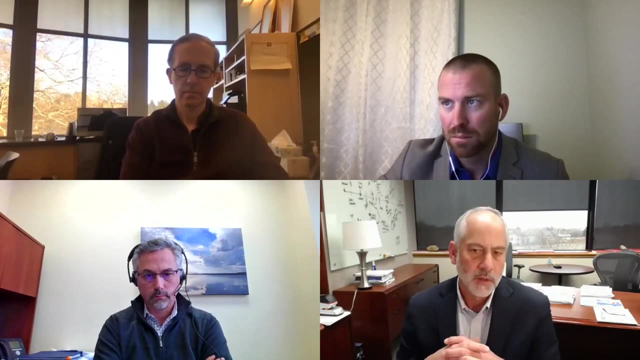 modular reactors. you know they were in development um in in testing programs for a number of years but when they, when they uh submitted their design certification application, the nrc it took. it took a little under four years to get that design certification. um nrc, i'll point out also- is considering um a new- i think it's called part 53. 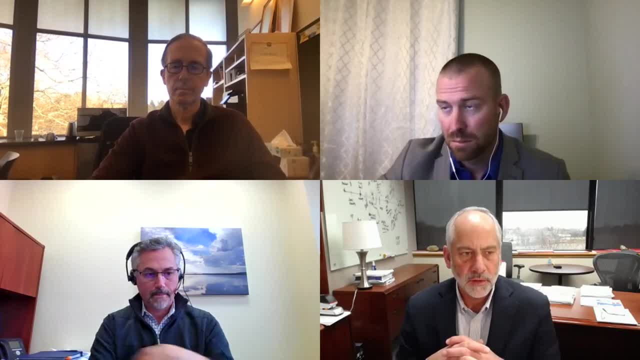 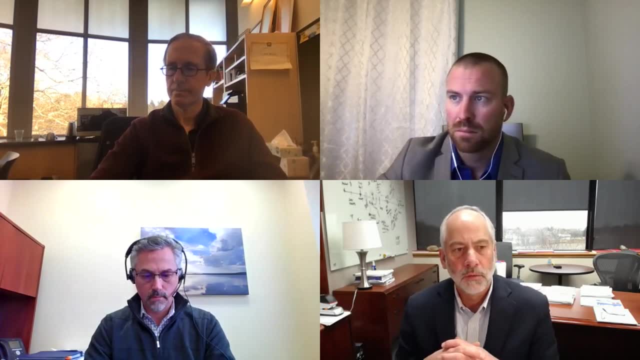 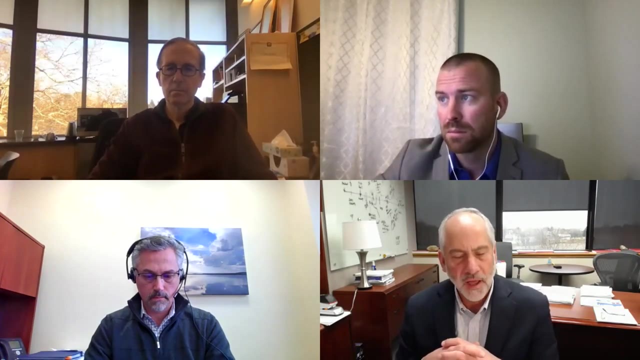 uh regulatory uh process that uh is more amenable is is better tuned, i guess i should say to um- to advance reactors in the safety uh state of those reactors. how that pans out, i don't know, that'd be a topic of maybe a good seminar if you invited an nrc person to talk about what they. 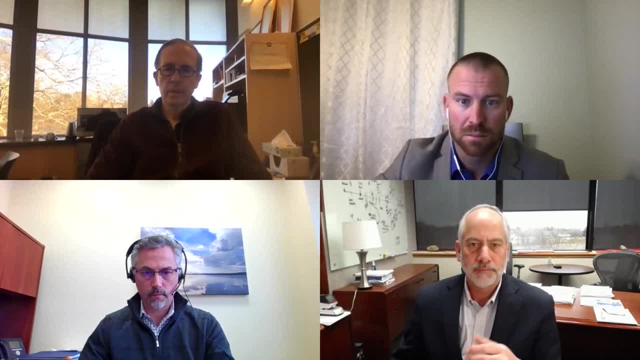 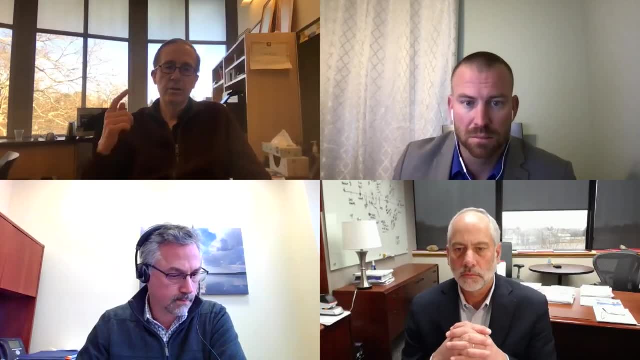 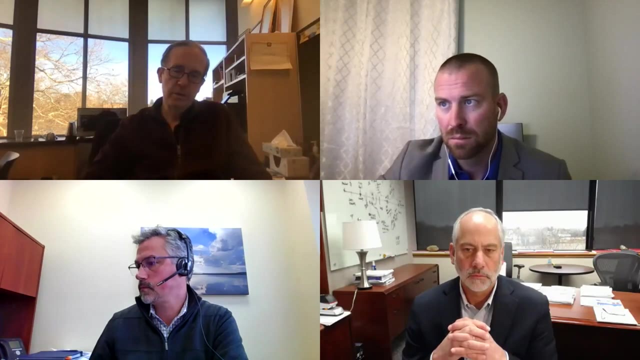 expect and and what the history has been. um, so yeah, steve, just a slight bit more on this part 53, right? i mean the nrc is trying to move expeditiously. congress gave them seven years to come up with a new process, the the nrc originally told its staff to move it down to 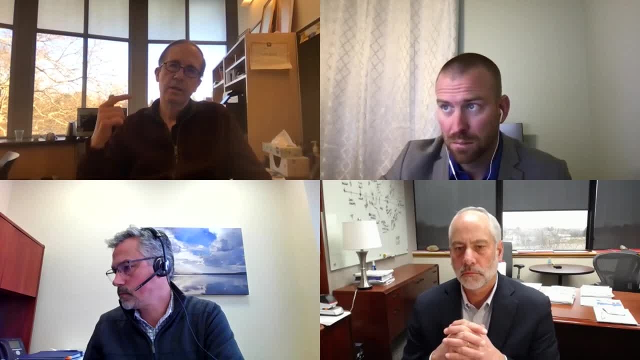 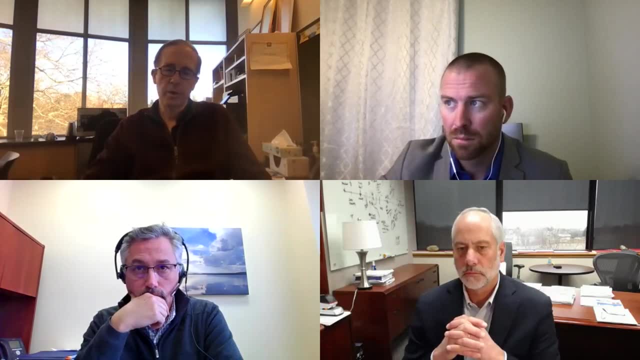 four, i think they backed off a little bit, um but uh. to steve's point. some of the reactor developers want to go faster than that, right? so they're not waiting for this new process. they'll use one of the two original ones, right? so the part 53 made maybe more influential on deployments that are a. 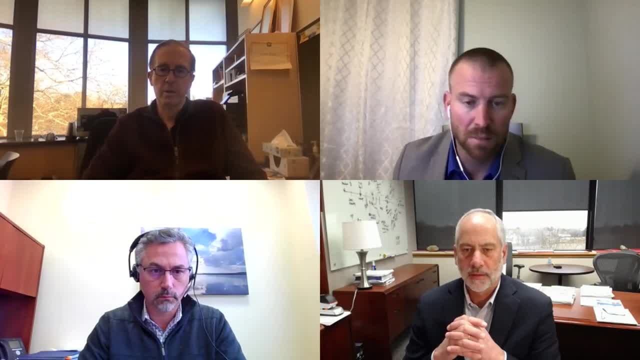 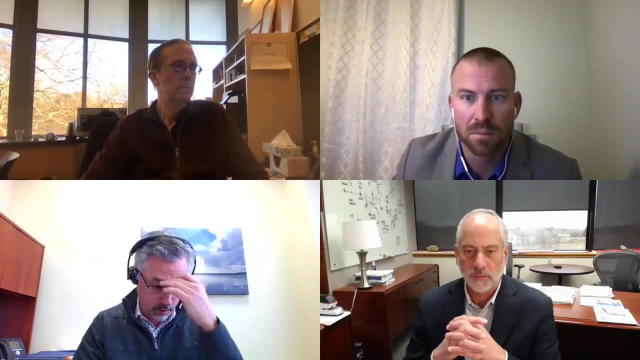 little further down the road than than the, the most immediate ones that people are talking about. so i think the the the the point of the report is that they're going to be able to move the nuclear plant out of the way for when they're going to move it back up, and so i think that's. 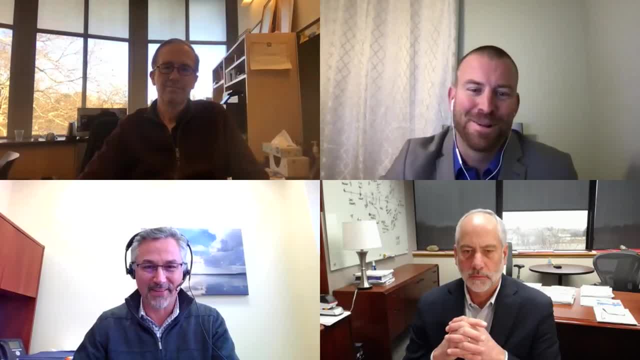 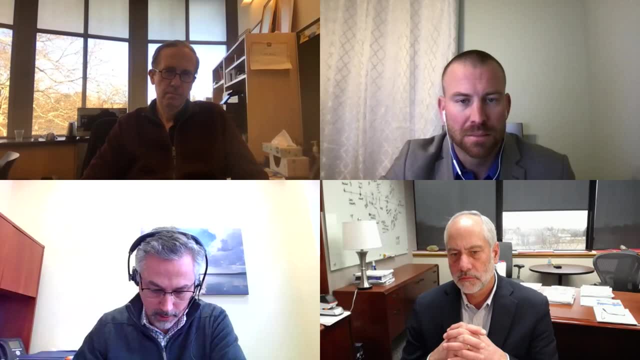 a really good point and i think it's a really good point to make. okay, thank you, we gotta. i think we have enough time for one more question here and, and it's, i'm gonna, it's, i'm gonna ask it since, uh, since i'm the moderator, i can do that, i have the power, but it's a good one, right, so you can hear. 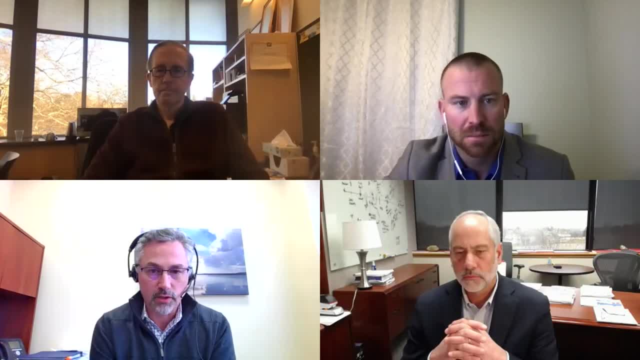 this a few times. uh, is it's with respect to the, the um, the report of 2021 by the union of concerned scientists. uh, titled advanced isn't always better- and that report raised a few interesting points regarding safety and proliferation and other things, and i think that's a really good point, because 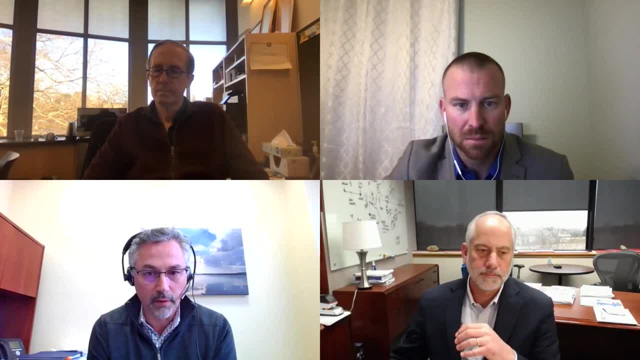 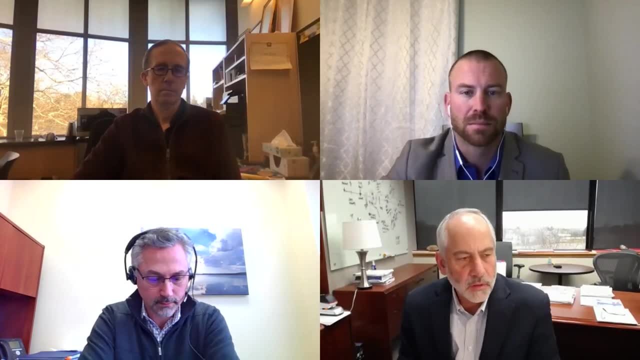 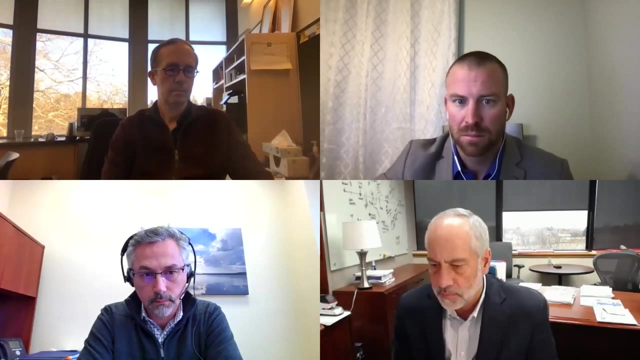 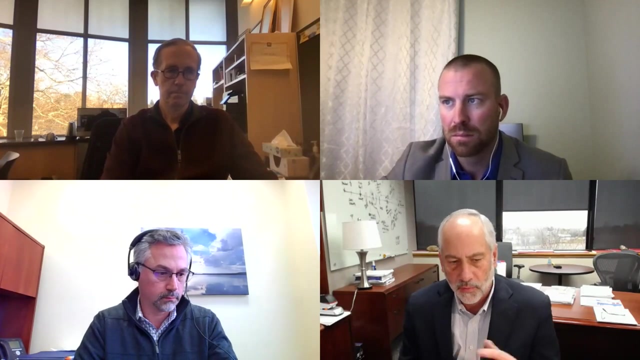 um, invite you all to comment uh on on the contents of that report and what your thoughts are. yeah, so i'll, maybe i'll, uh, i'll start. so the um, the analyses that were done in in the report certainly are. they didn't, they didn't. i was very i've been familiar uh with, with um, with with that. 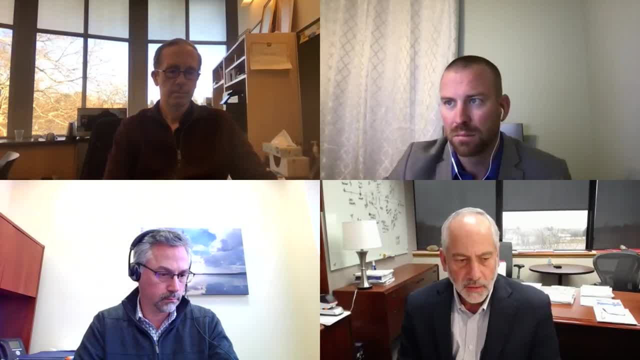 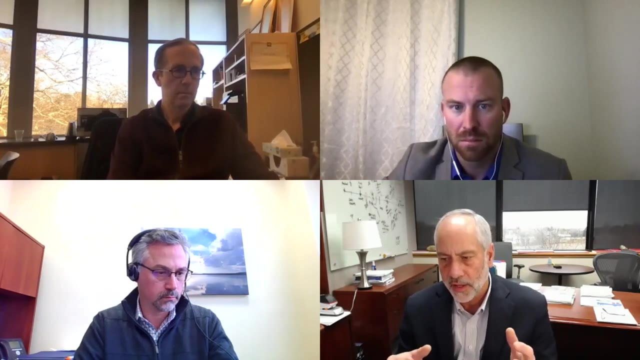 that line of analysis and reasoning, and you know you talk about advanced reactors as a bin, but. but maybe just to focus on a couple things i do know something about. so, for example, um, i gave the uh, the example of the sodium cooled fast reactor, if you have a pool uh, a pool type reactor, 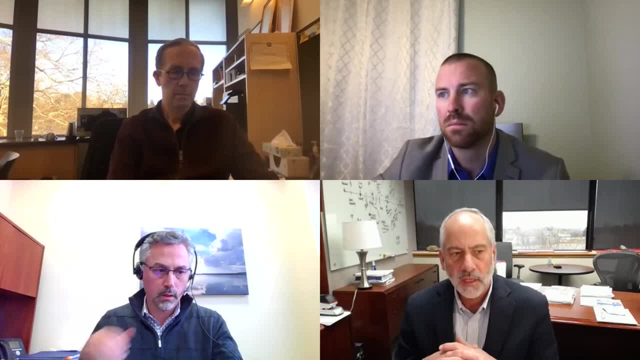 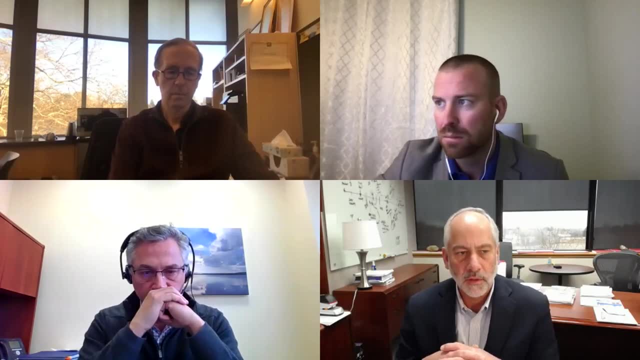 the experience on those uh have actually been really very good. um. i gave you the ebr2 examples, so the the, the notion of passive safety um isn't a theoretical construct. i mean that that's something that's been uh, you know, we've shown and we've validated and demonstrated. 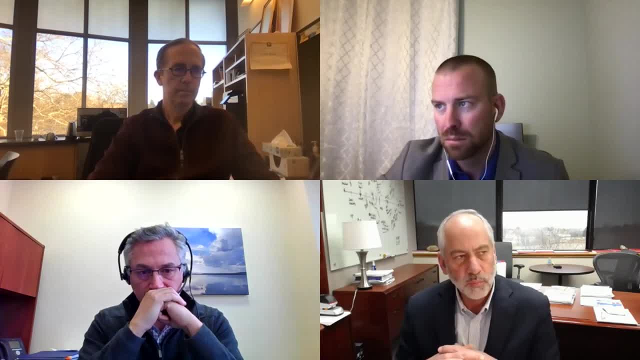 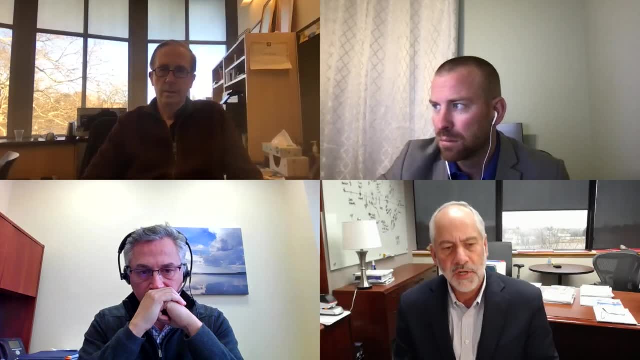 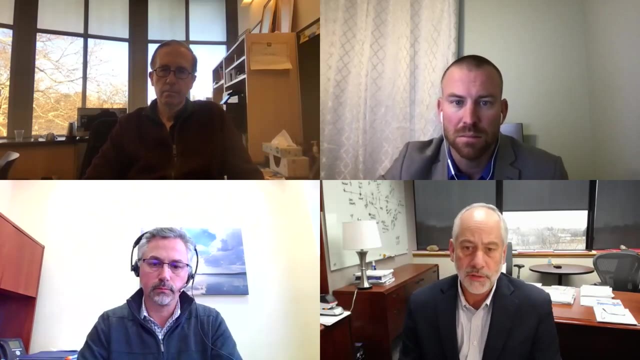 uh other systems around the world that they were not pool type uh sodium cooled fast reactors. for example, i think manju might have been mentioned in the report- that was a japanese reactor uh that shut down early um problems that they had were really operations uh oriented uh very much so um. 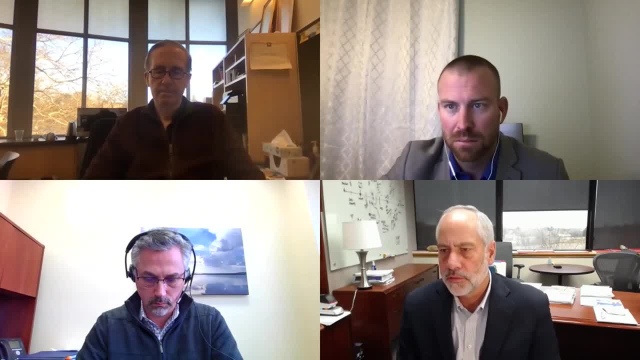 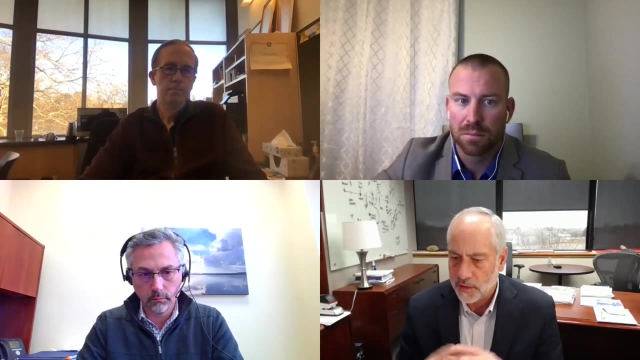 let me, let me touch on non-proliferation, because that's that's an interesting thing that comes up uh quite a lot uh when we're- even when we're talking about us uh reactors to be built in the us. so non-proliferation is a is is a serious, it's to be taken seriously and it's a serious. 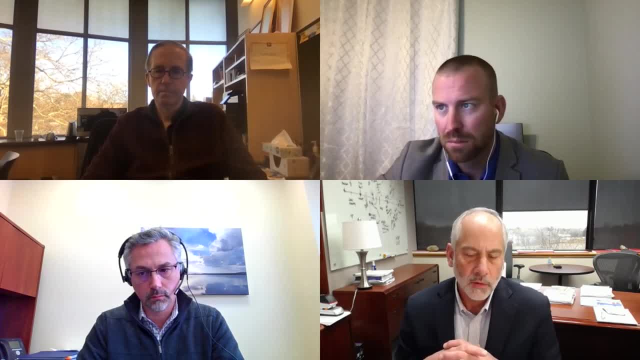 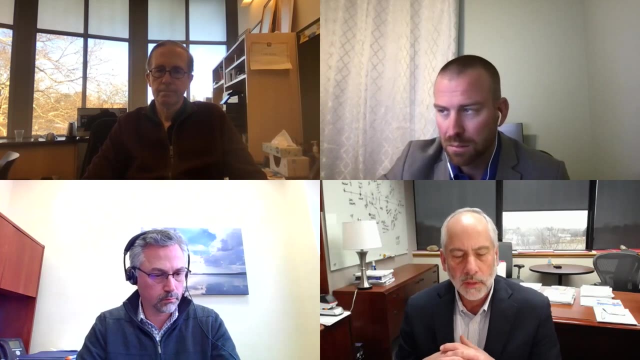 concern when you're thinking about where to deploy nuclear systems around the world. and and the question is, is somebody going to hijack a fuel cycle and begin the the arduous process of extracting weapons usable material from a fuel? that's typically not something we think about here in this country, because this country uh has, uh, you know, we, we, we own an. 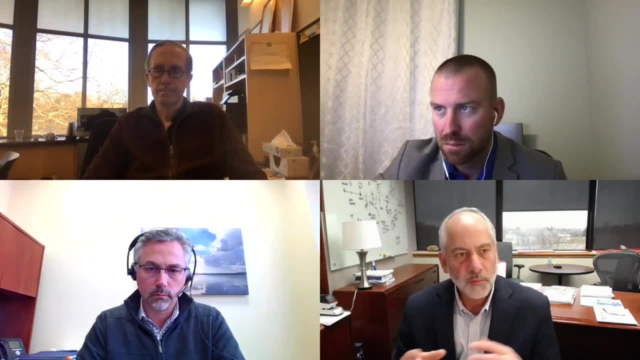 operating. we have uh limits on what people can do within our boundaries, but, you know, when you're thinking about export, uh, those are, those are considerations, those are considerations, and there's uh very effective uh regimes uh in place. i would also uh add: you know, if you're thinking, 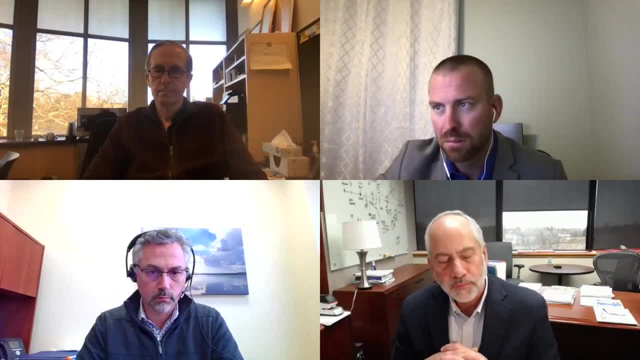 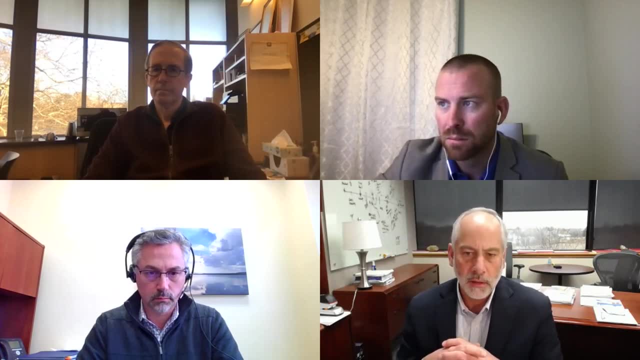 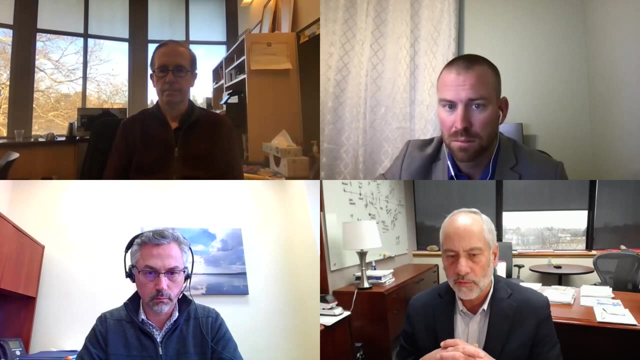 about exporting and growing the market, uh for nuclear technology, uh, globally, uh. the things that we can do today in terms of monitoring and control of a system anywhere in the world from anywhere in the world, simply couldn't have been imagined back in the 1960s, 1970s. 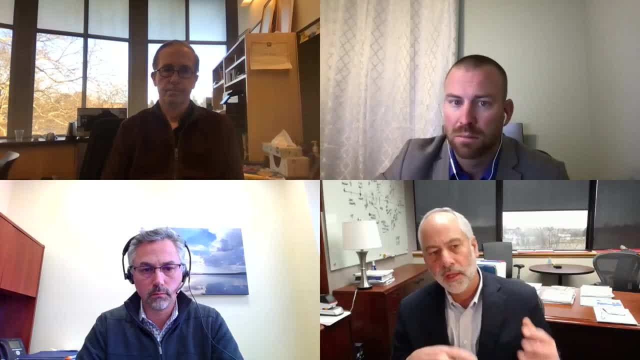 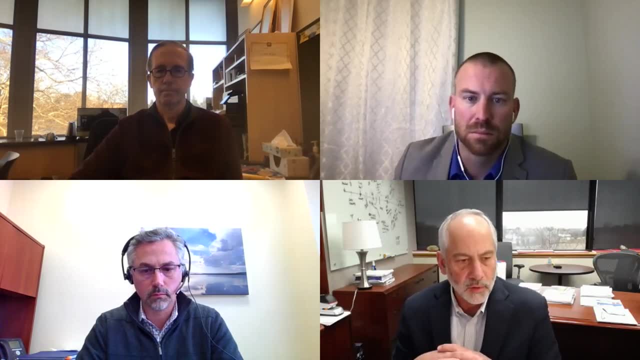 even the 1980s. so i argue that the landscape is fundamentally different and we need to think about exports uh differently as well. so that touches on non-proliferation. uh cost is brought up in the report we've talked about with the other questions that you had, glenn. 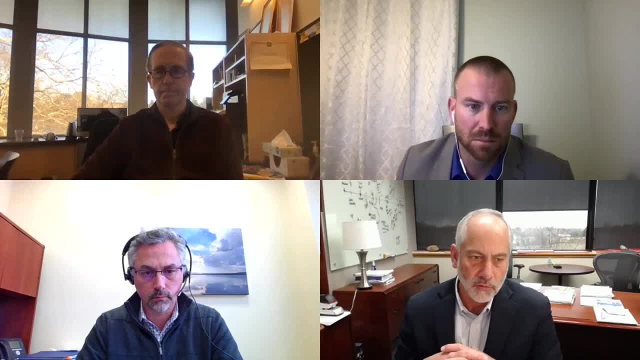 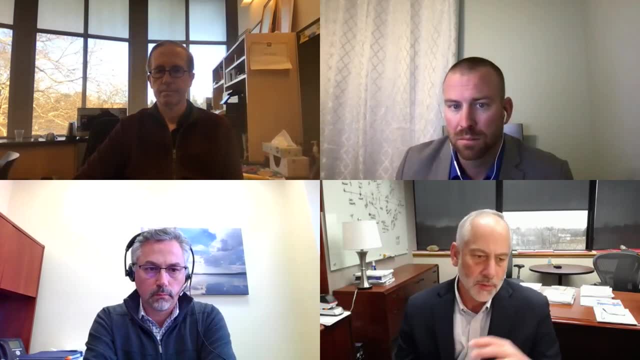 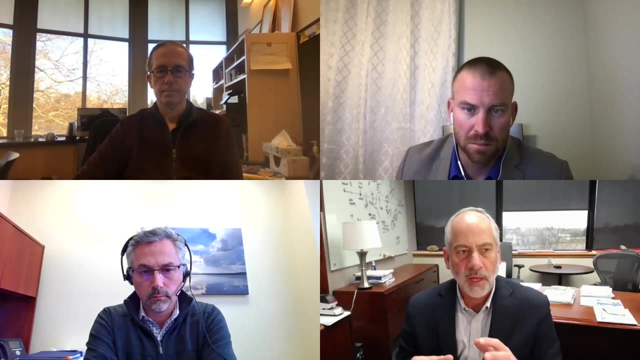 talked about cost, talked about what's different going forward, what's been learned over the past 65 years. so it's important to put all of that in a in in perspective and, uh, think about what todd mentioned. i like this this way of looking at it. uh, what's the value of what you're? 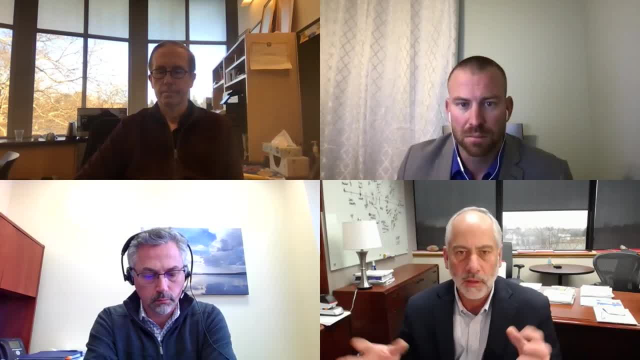 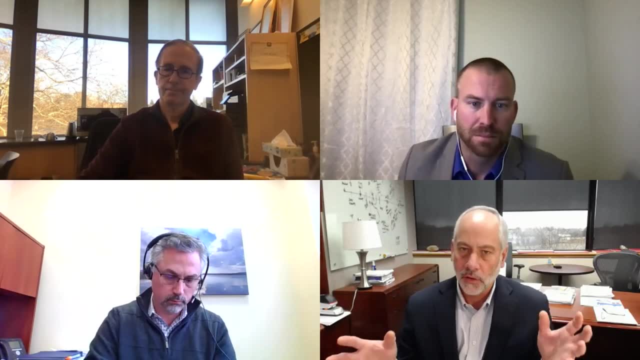 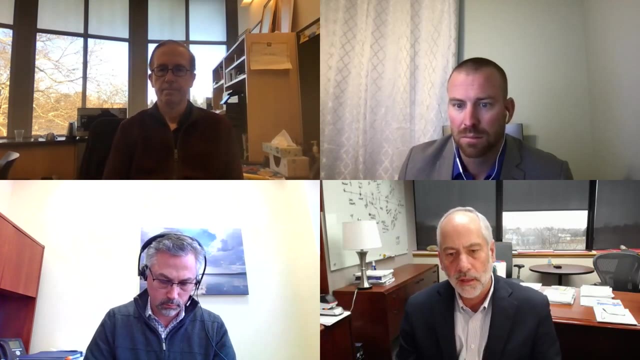 producing versus the uncertainty that you take on, or or the the cost, or the risk, and you need to approach that with very open eyes, right, and to do that, uh, you look at data and you look at the best, the best uh data available, uh and the best assessments, and the community has to make a 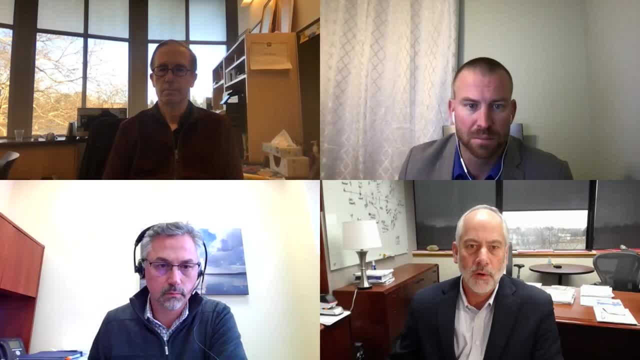 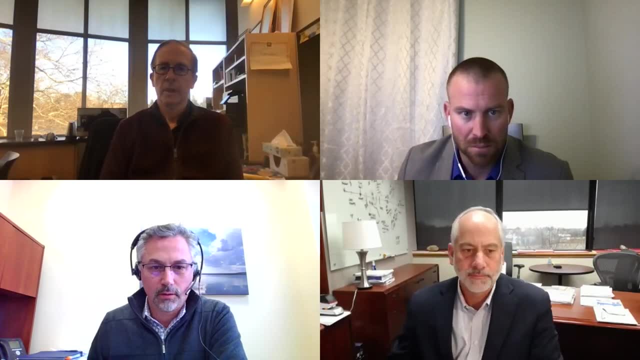 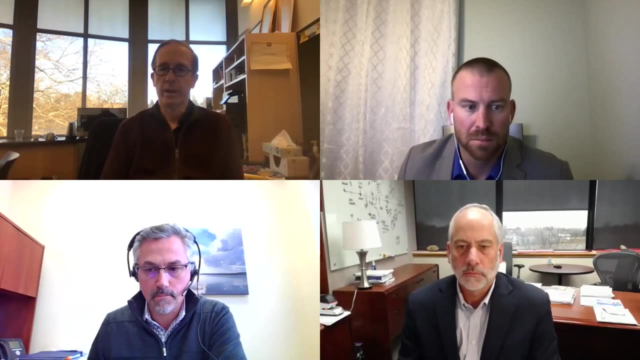 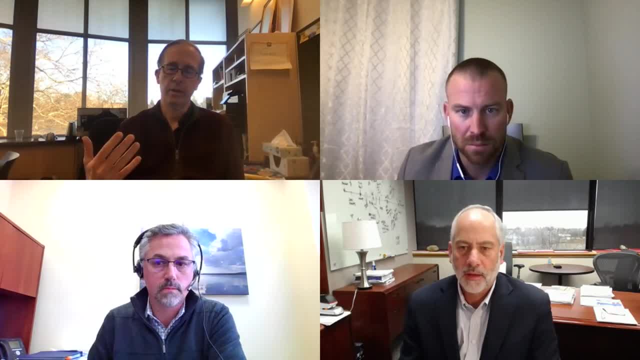 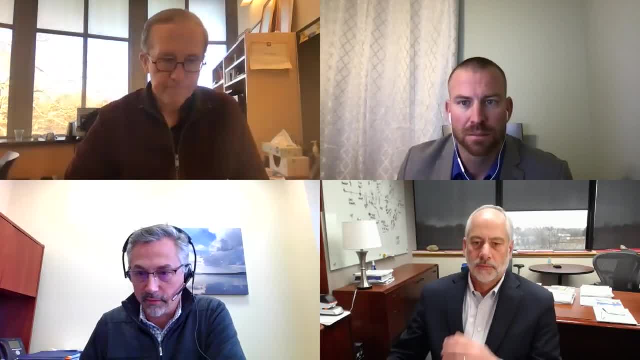 piece of what you just said about the cost. i think that's kind of kind of interesting and i think i'm going to talk about that um later and then we'll have to discuss some other things, but that's great. literally 30 seconds for any closing comments. 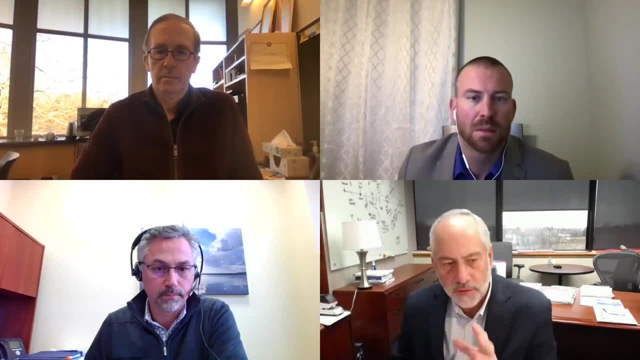 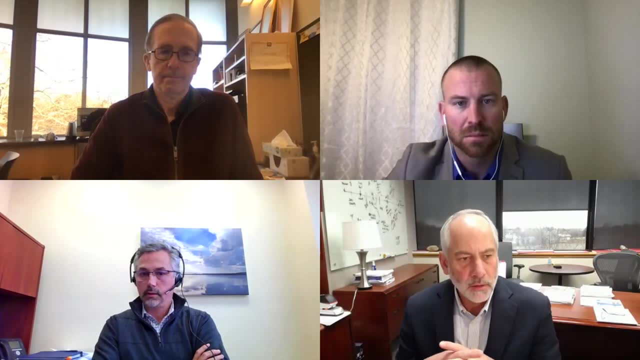 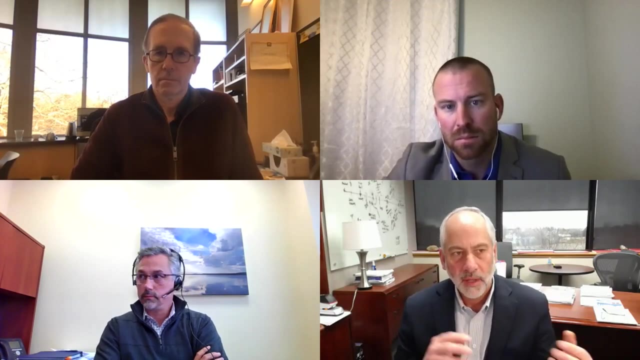 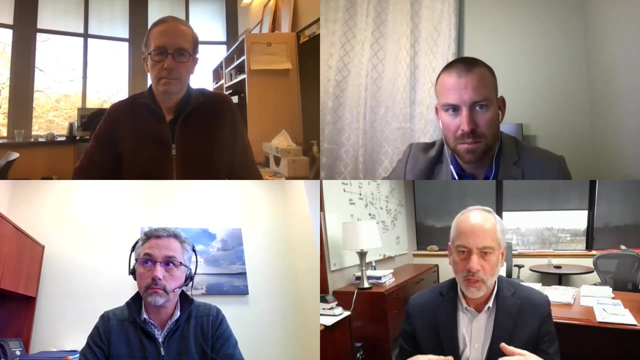 Quickly. anybody want to take opportunity there? Just make one comment: I'd applaud what the folks, what your colleagues and you, Glen, are doing in Wyoming. Have a dialogue, Have an ongoing dialogue about benefits and costs and what can communities get out of something beyond just. 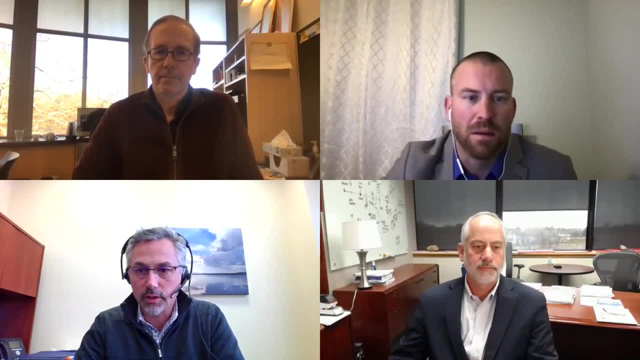 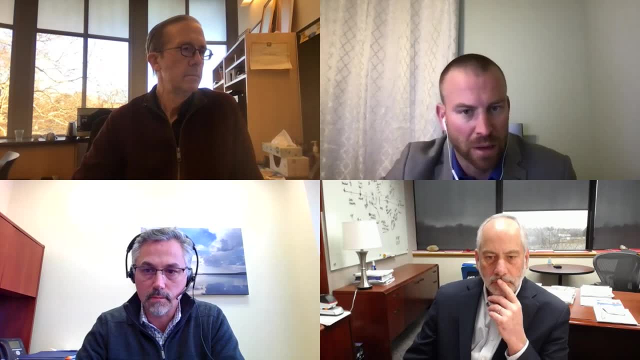 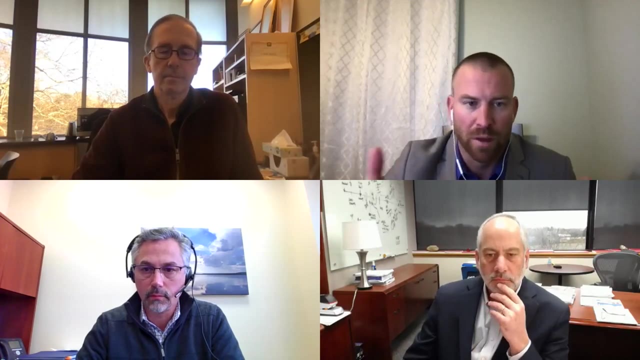 shipping electrons off Josh. Yeah, let me just go, Steve. I think had mentioned this a couple of times. There's several more deeper technical comments and discussions that could be had around advanced reactors and advanced nuclear And I think at any time if this organization is interested.